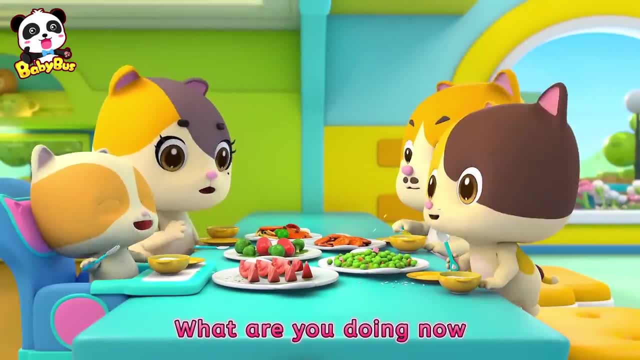 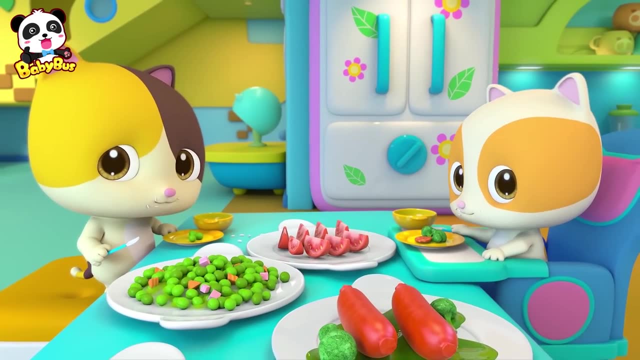 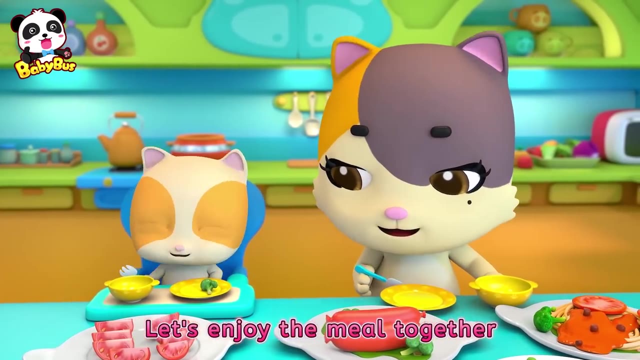 Oh, oh, oh. what are you doing now? No, no, no, don't talk with your mouth full. Okay, Let's enjoy the meal together. Who has the best table manners? Oh, oh, oh. what are you doing now? 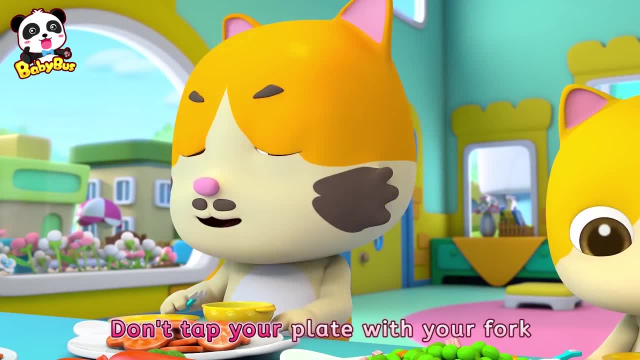 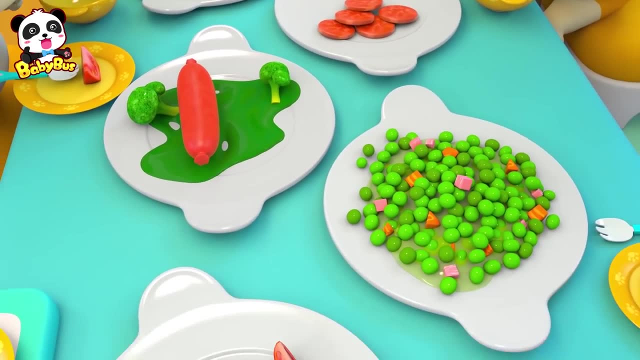 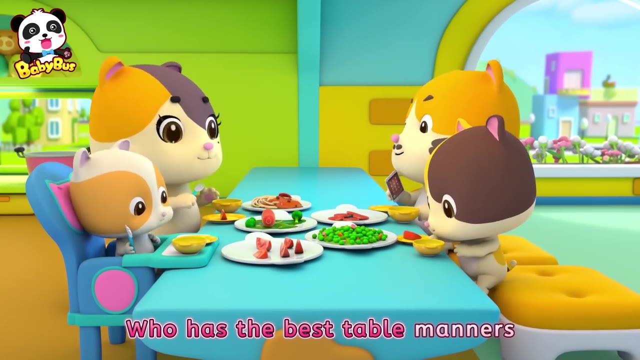 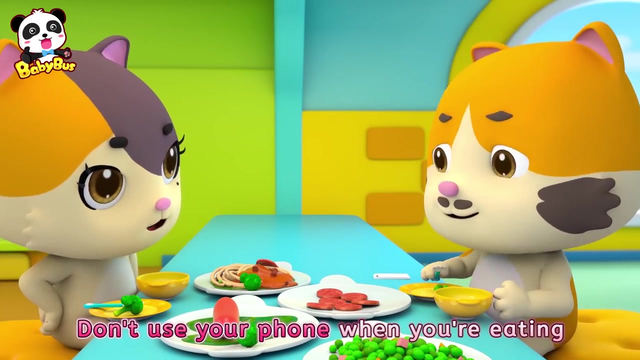 No, no, no. don't tap your plate with your fork. Okay, Let's enjoy the meal together. Who has the best table manners? Oh, oh, oh. what are you doing now, Now, now, now. Don't use your phone when you're eating. 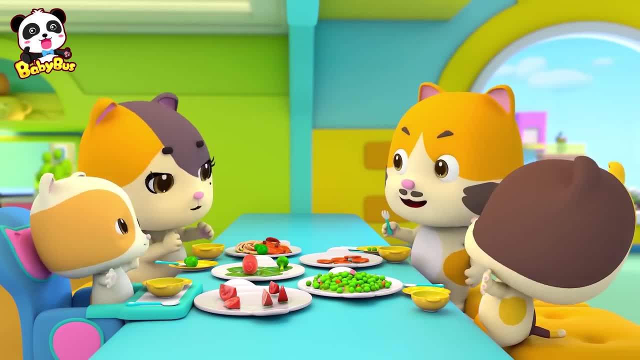 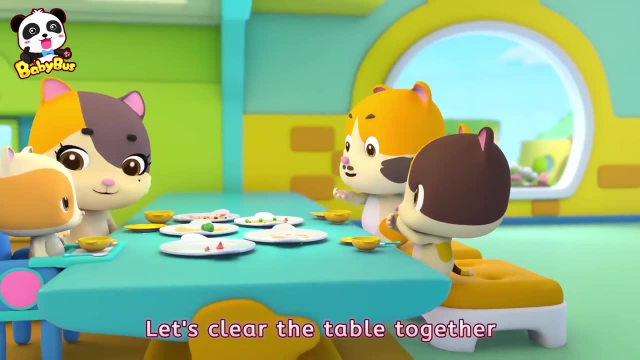 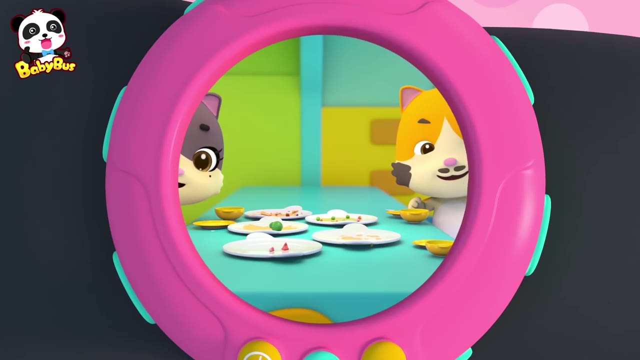 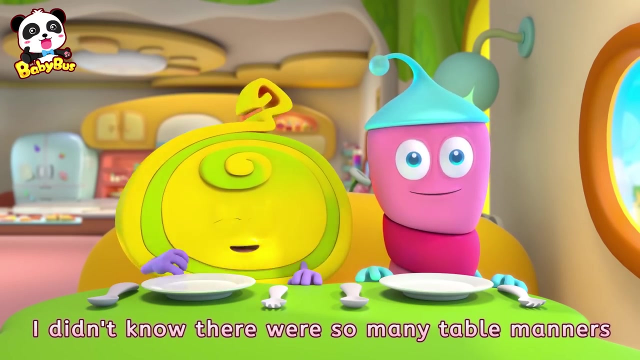 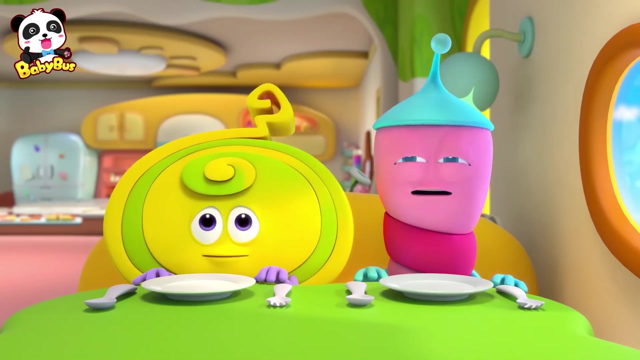 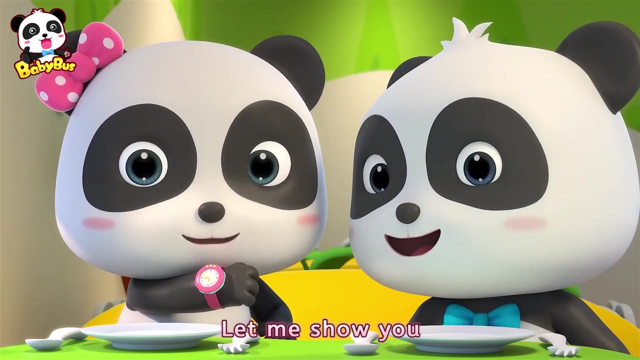 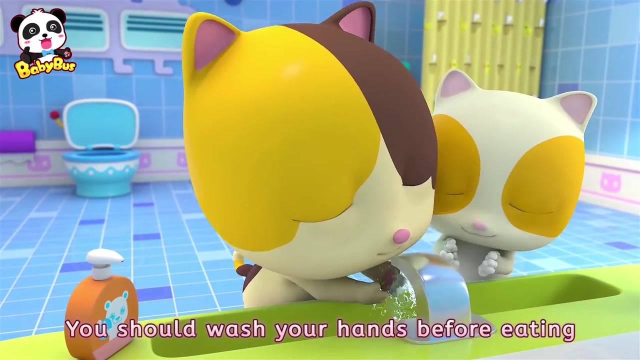 Okay, Daddy, hurry, Let's clear the table together. Okay, I didn't know there were so many table manners. I remember all of them. Do you know any other things about table manners? Let me show you. You should wash your hands. 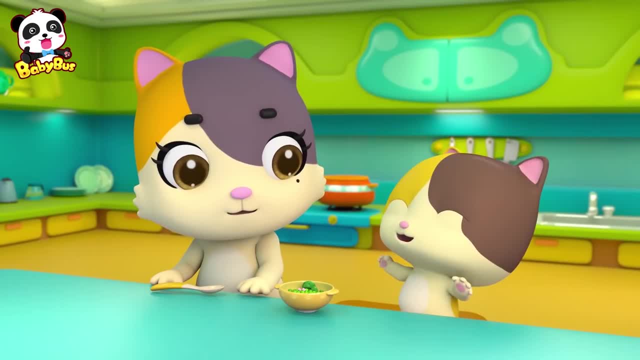 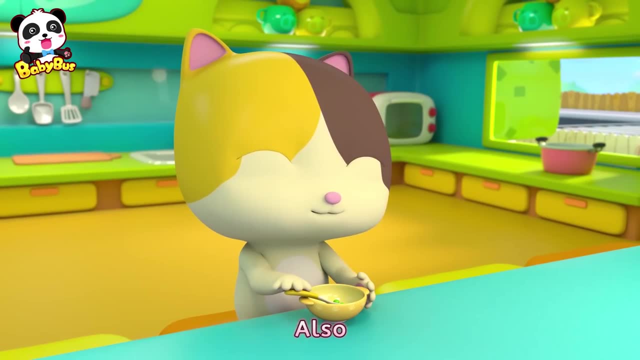 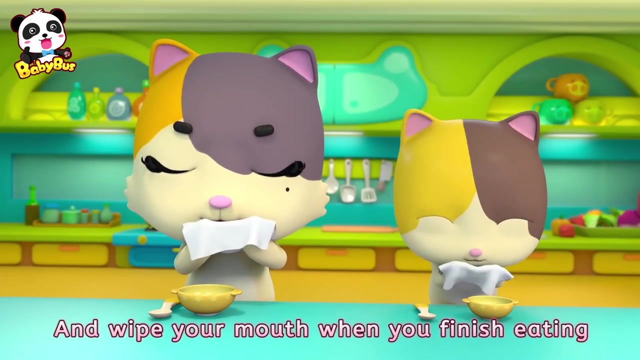 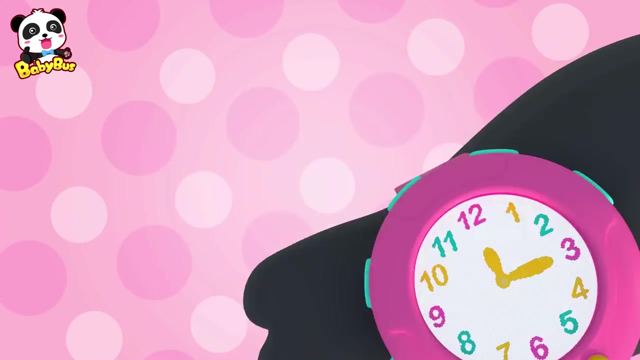 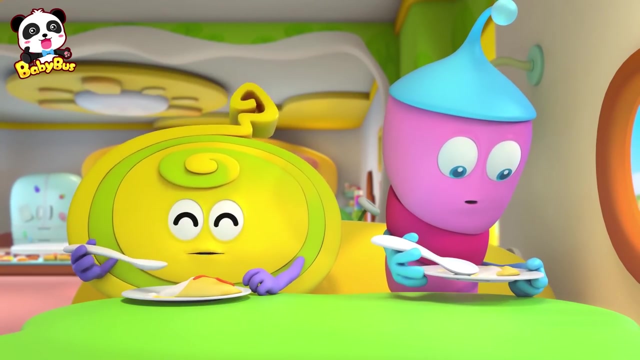 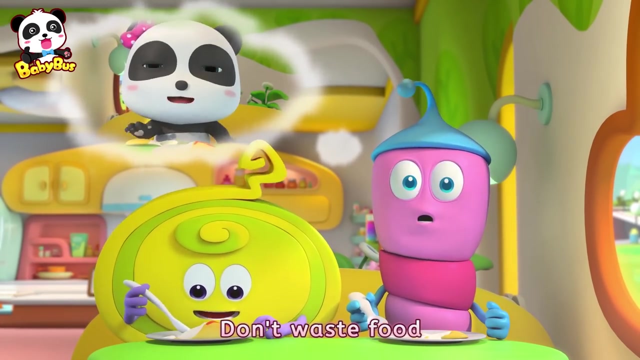 Wash your hands before eating. Don't eat with your hands at the table. Use your utensils. Also, try to eat everything in your dish and not waste any food, And wipe your mouth when you finish eating. Don't waste food. Don't waste food. 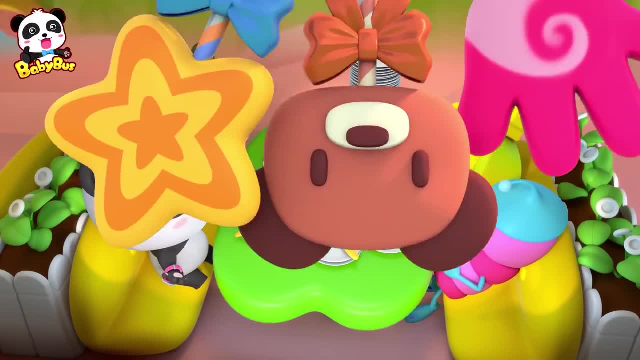 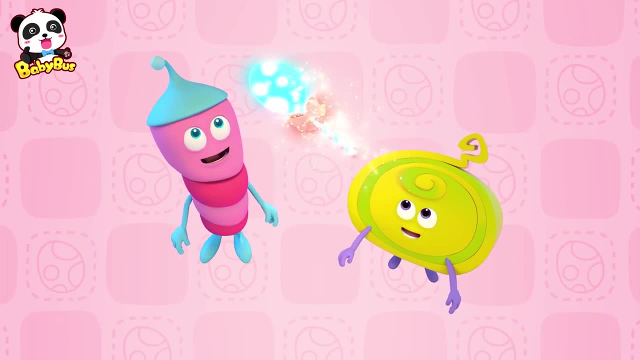 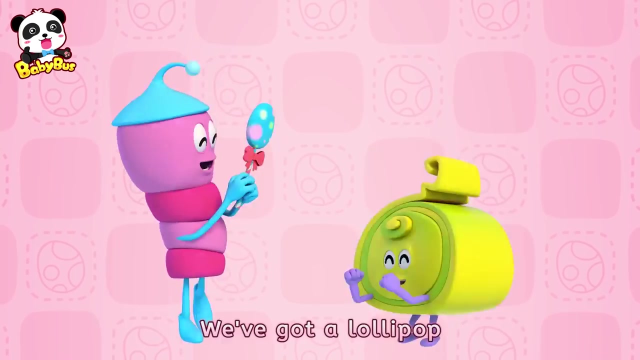 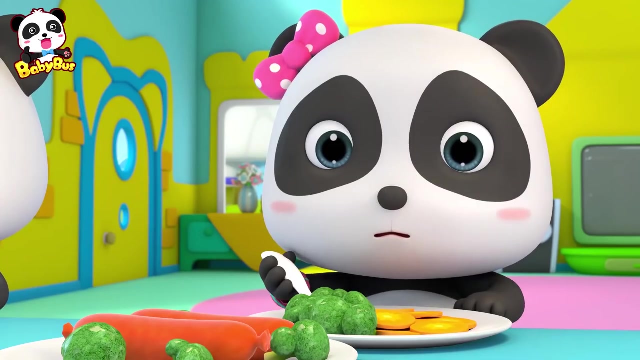 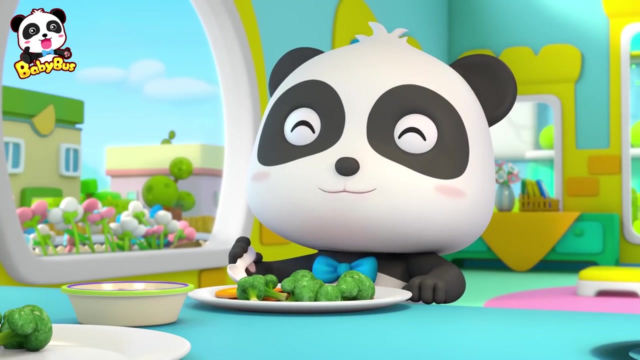 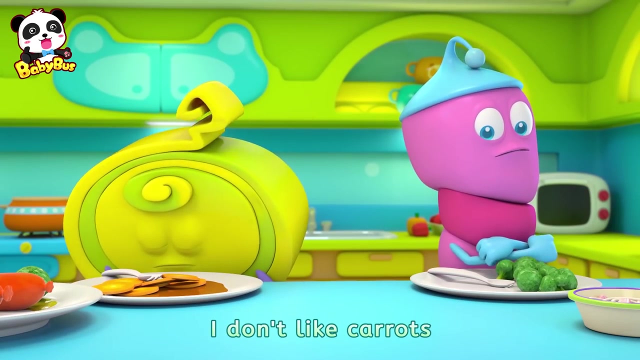 Wow, Aliens can eat a lot. Now we know about table manners. We've got a lollipop. We've got a lollipop. Have some broccoli And carrots. I don't like broccoli. I don't like carrots. Kid Cat, it's not good to be a picky eater. 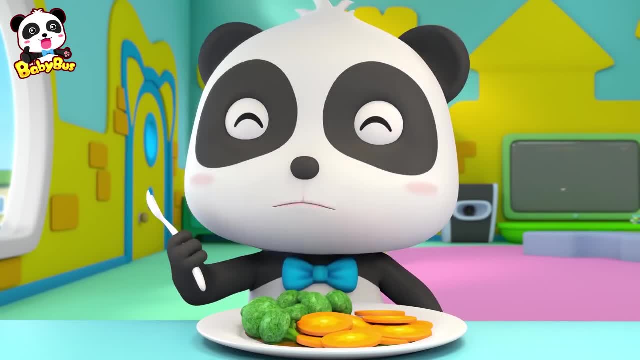 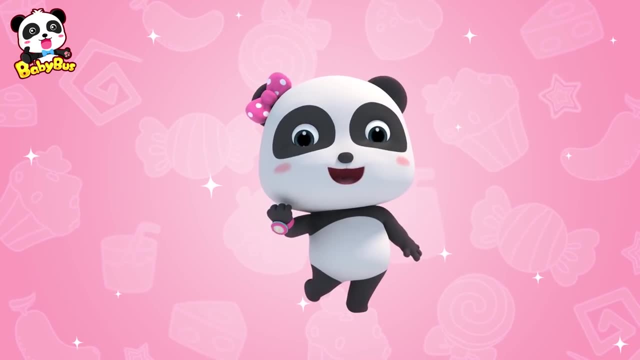 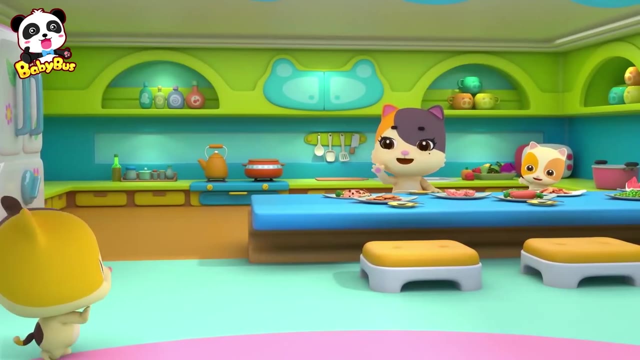 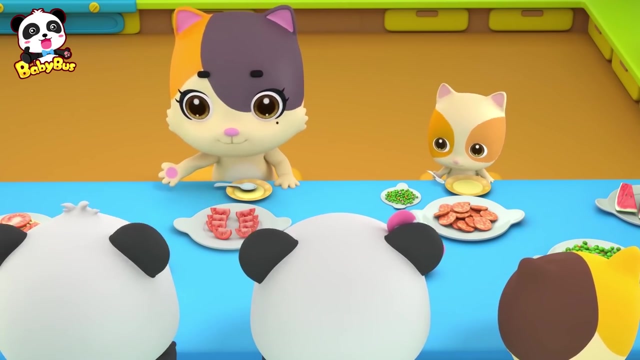 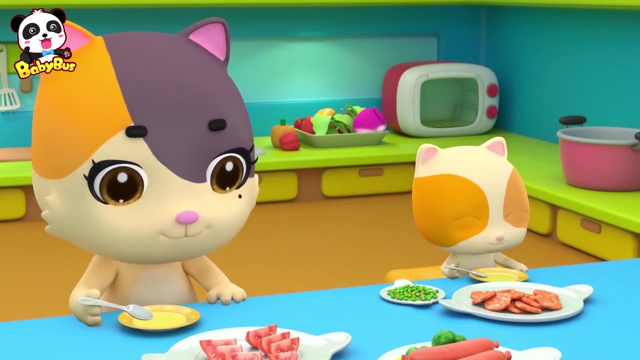 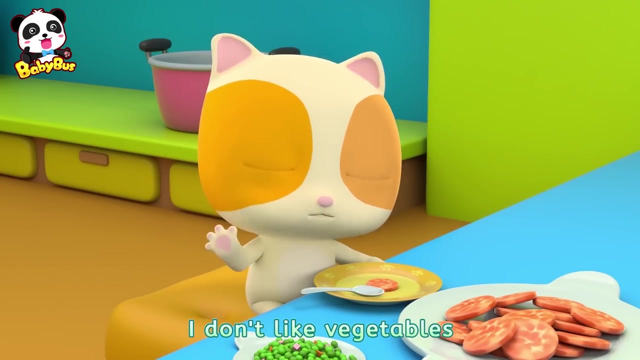 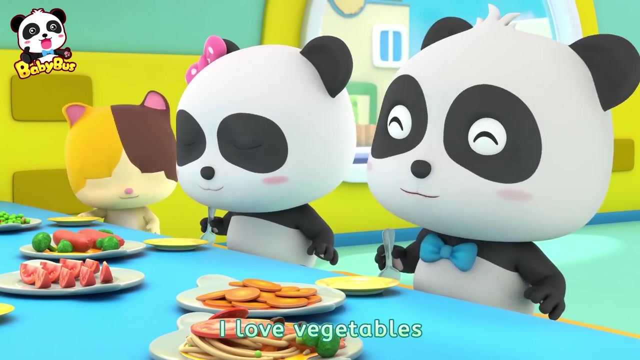 And veggies are good for you. Let's learn about healthy eating habits. It looks delicious. Help yourselves, Timmy, you should eat vegetables too. I don't like vegetables. Vegetables are good for you, Right? I love vegetables. Come everyone, let's eat together. 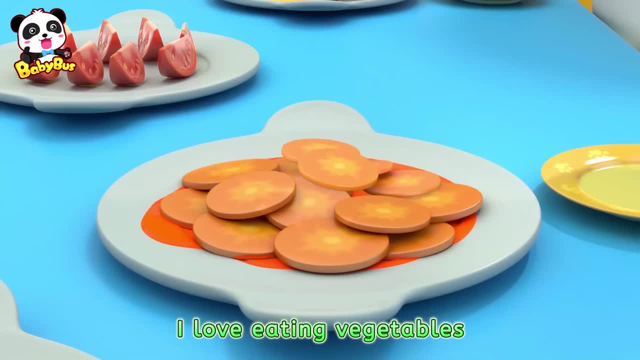 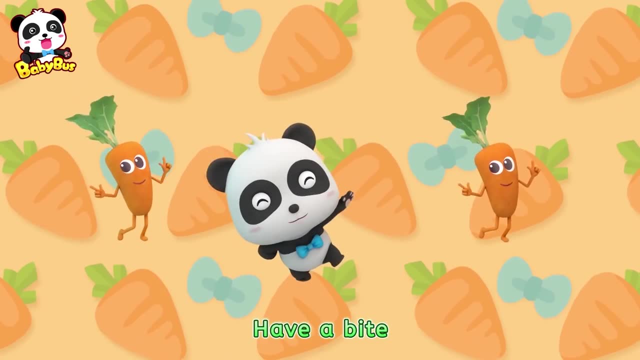 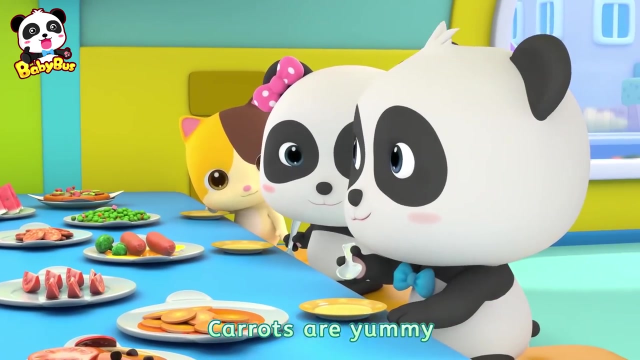 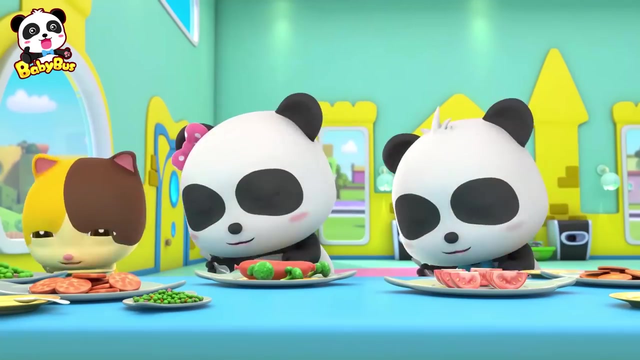 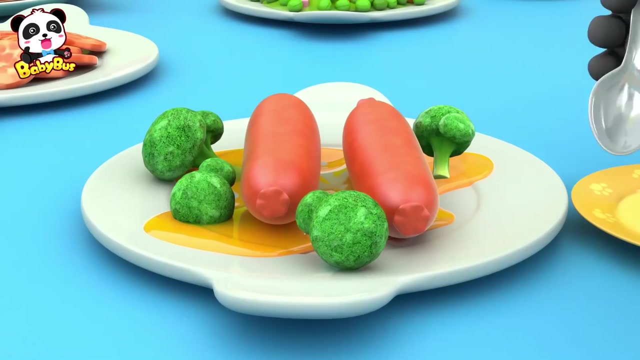 I love eating vegetables Carrots. Yum, yum, yum, yummy. have a bite So fresh, so good and good for me, Carrots are yummy. I want some broccoli. Come everyone, let's eat together. I love eating vegetables Broccoli. 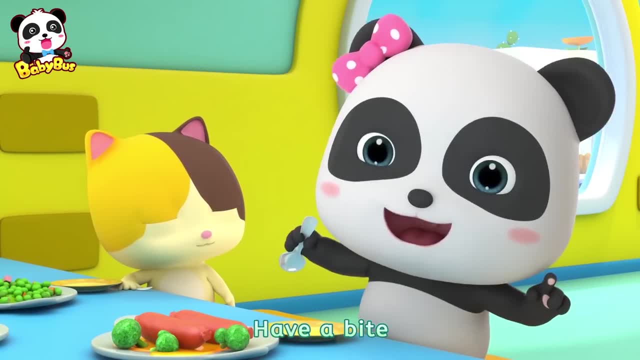 Broccoli. Yum yum, yum, yummy, have a bite. So fresh, so good and good for me. Come everyone, let's eat together. I love eating vegetables. Green peas, Green peas- Yum yum, yum, yummy, have a bite. 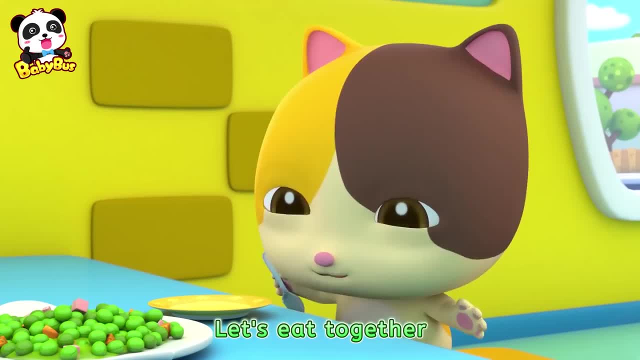 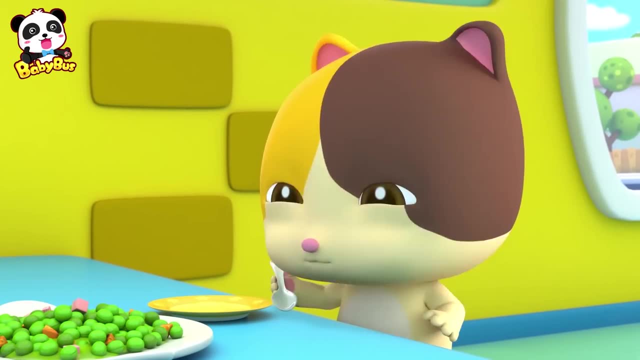 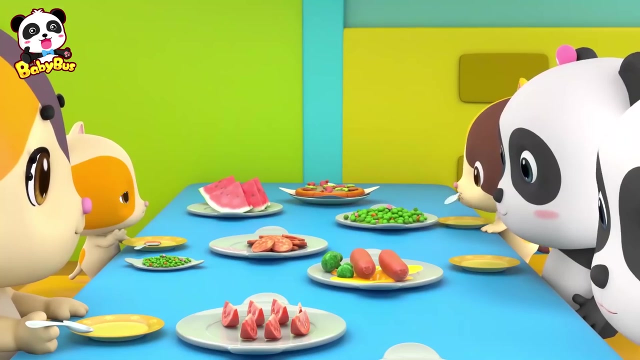 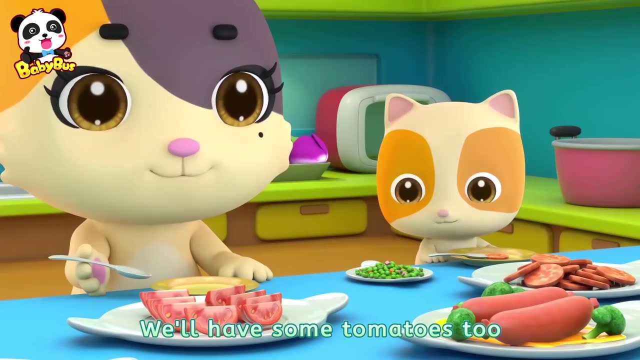 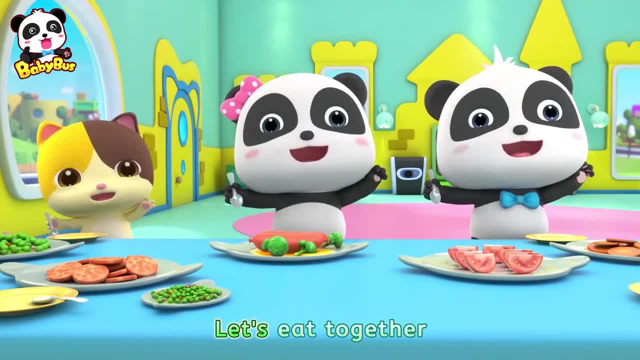 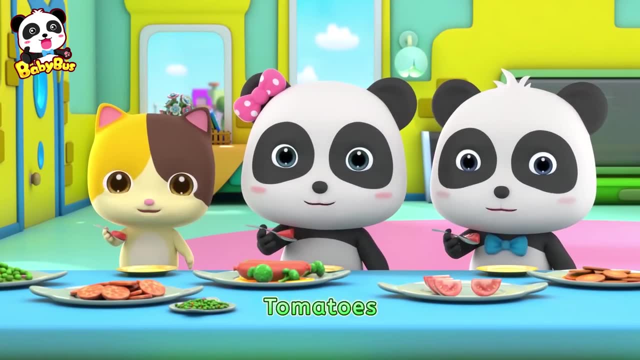 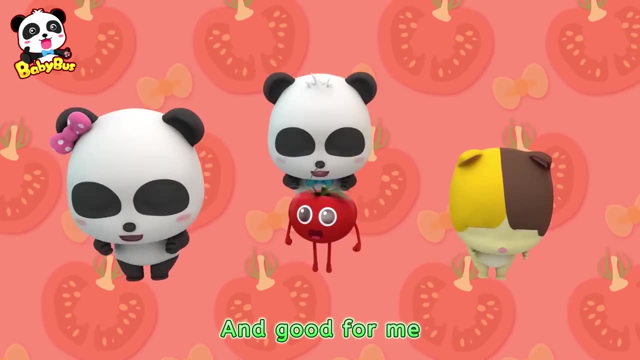 You got obrig one Time to go to school, And we'll have some tomatoes too. Come everyone, let's eat together. I love eating vegetables. Tomatoes, Tomatoes, Yum, yum, yum, yummy. have a bite So fresh, so good and good for me. 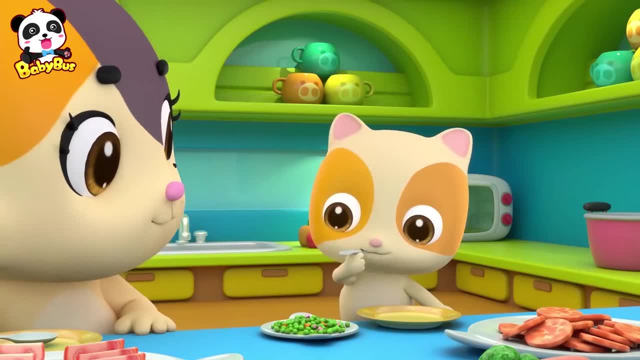 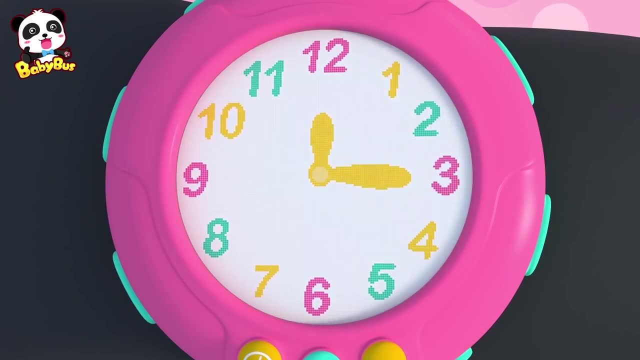 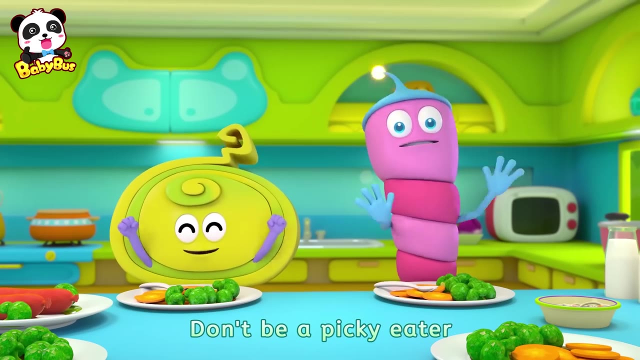 So fresh, so good and good for me. I want to eat some vegetables. Gutz Great, Got all my vegetables. That's great. I'm happy Got it Eating a lot of veggies. Don't be a picky eater. Don't eat just veggies, but all kinds of food. 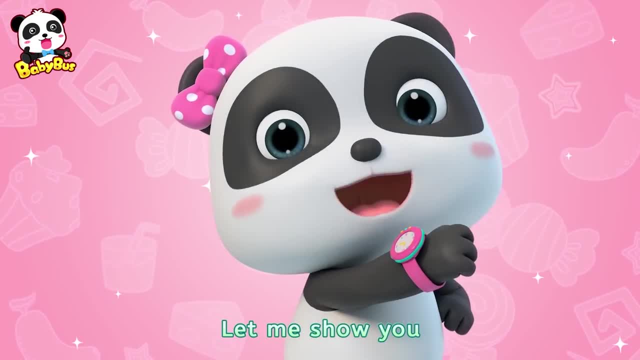 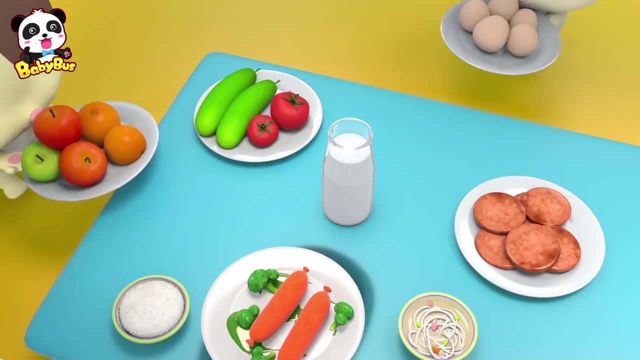 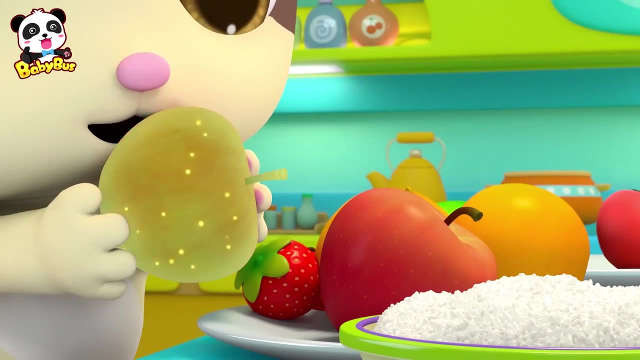 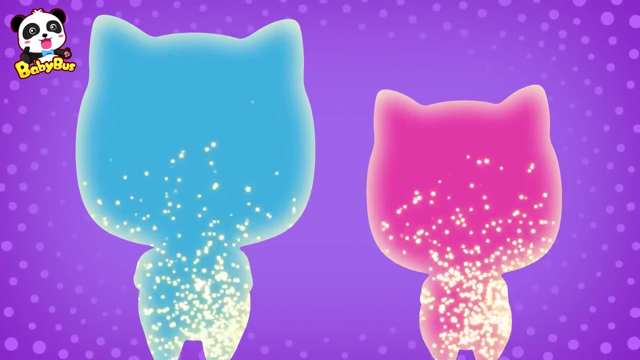 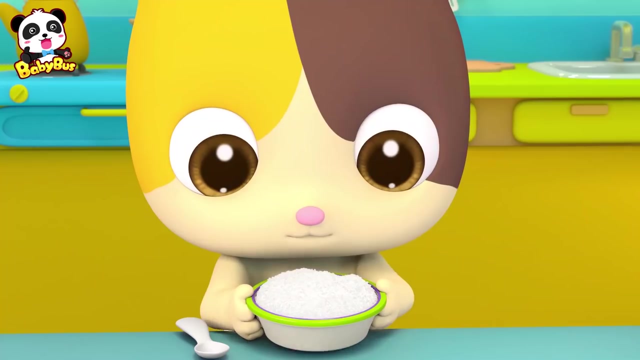 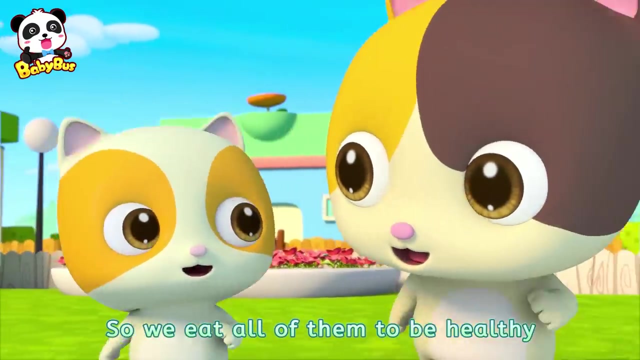 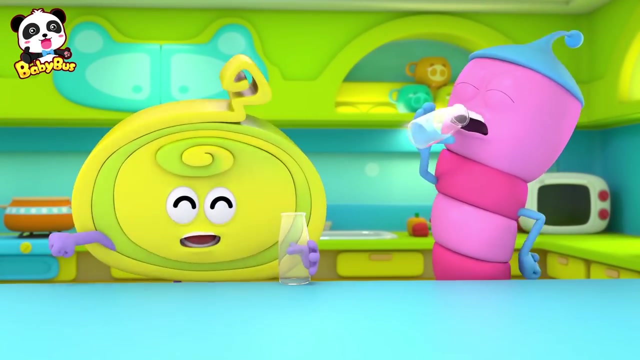 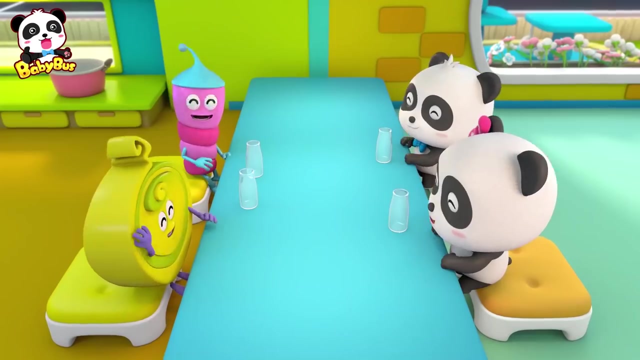 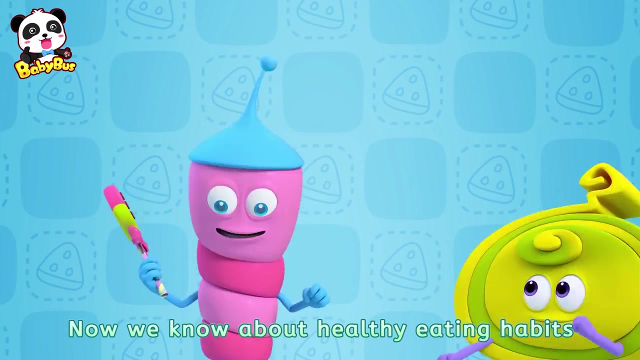 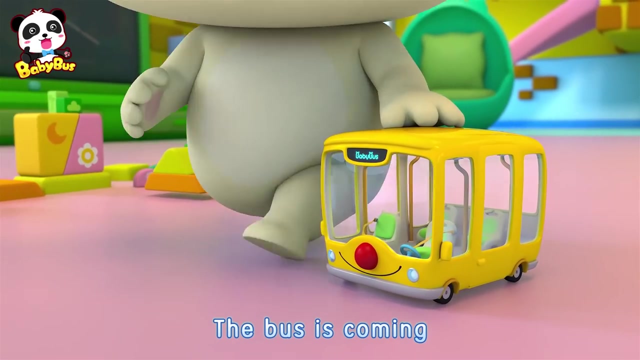 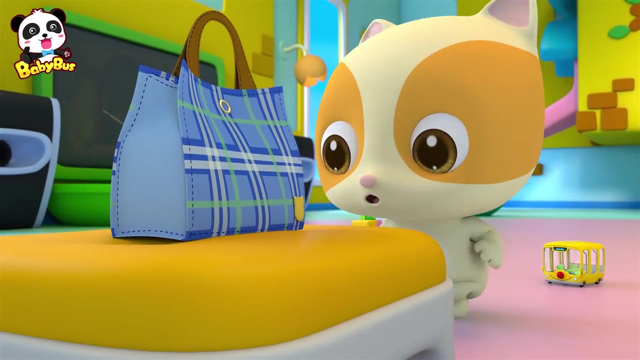 Why? Let me show you. Let me show you. So we eat all of them to be healthy. Now we know about healthy eating habits. We've got a lollipop. The bus is coming. What's that? It's Daddy's lunchbox. 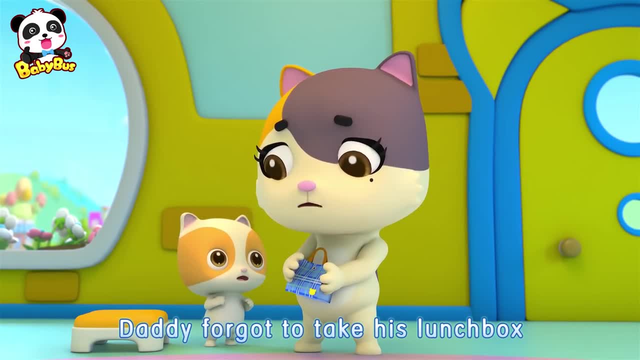 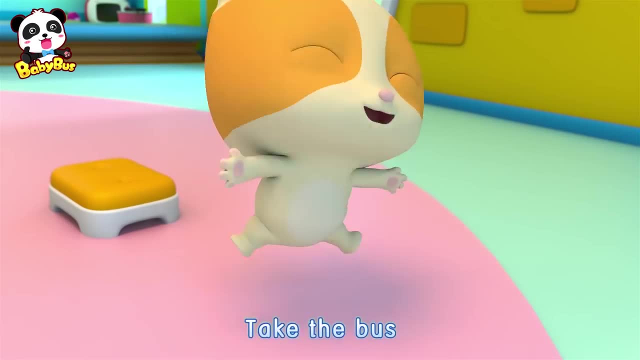 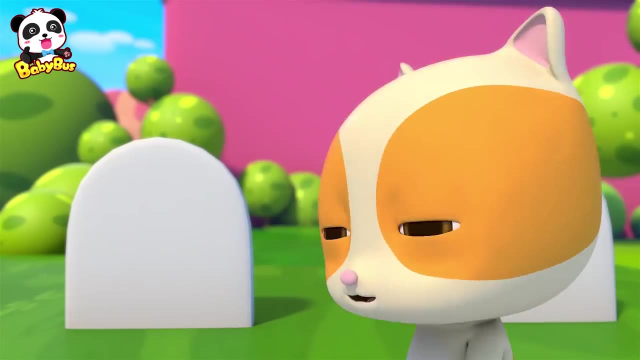 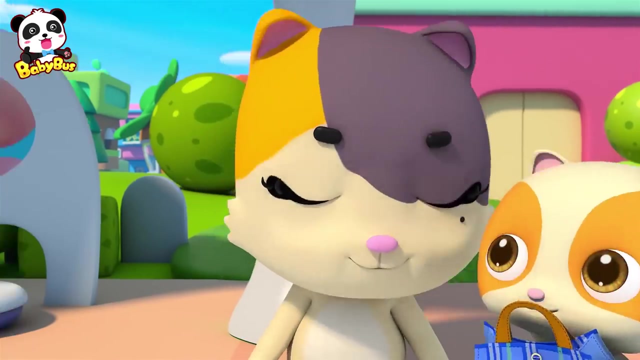 Daddy forgot to take his lunchbox. Let's go to Daddy by bus. Take the bus, Take the bus, Let's take the bus, yeah, yeah, The bus is coming, coming, Let's take the bus, yeah, yeah. 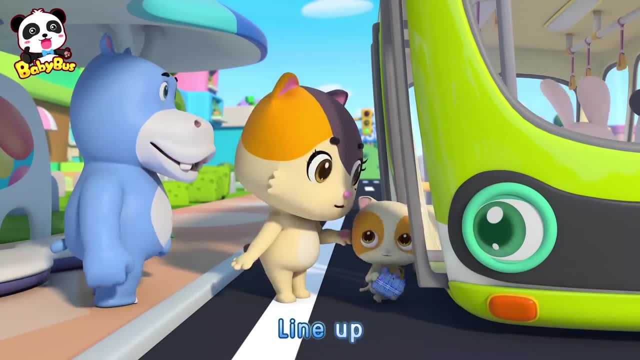 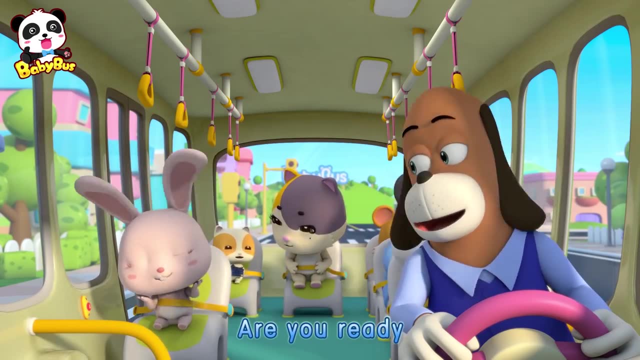 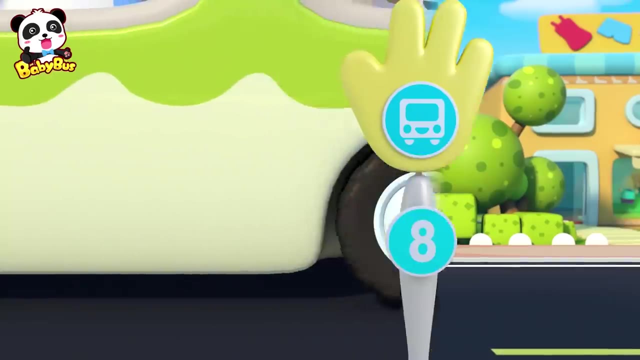 The bus is here. yeah, yeah, Line up, line up, ride the bus. Clink, clink, put the coins in. Everybody, are you ready? The bus is moving now. Yeah, The wheels of the bus go round and round. 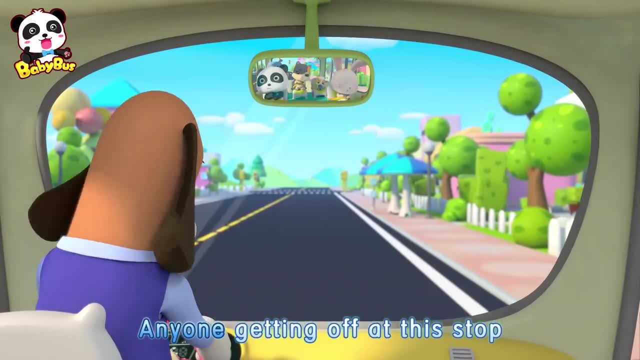 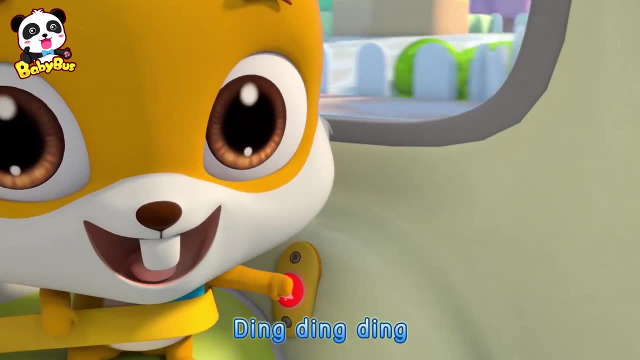 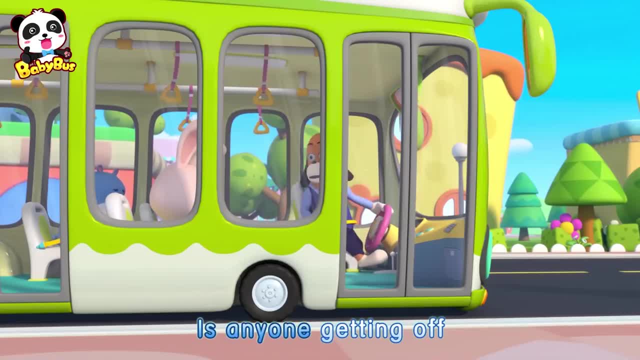 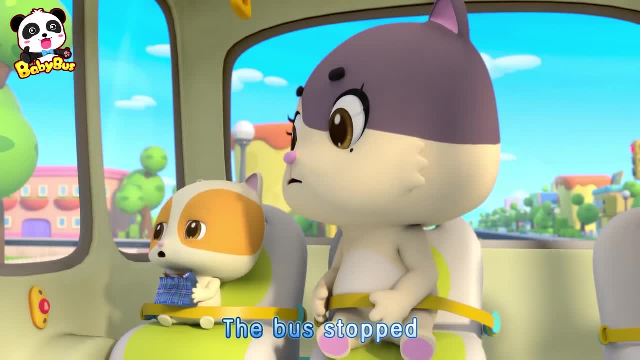 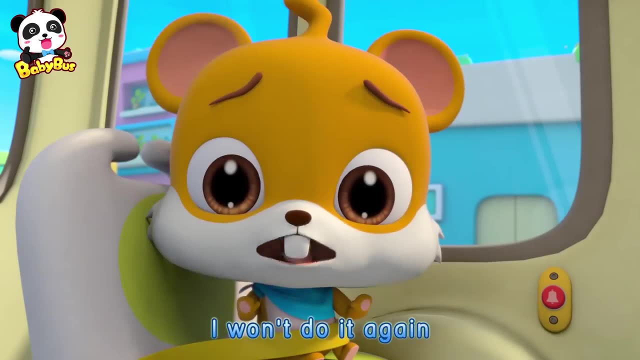 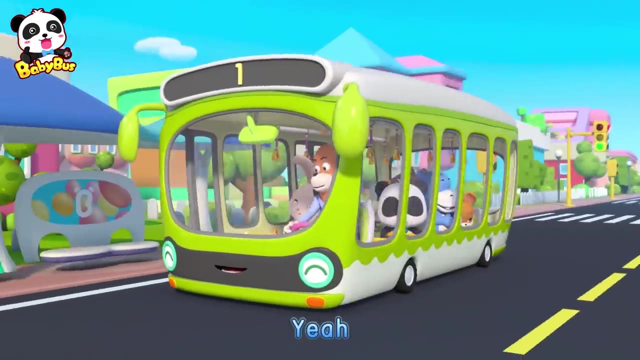 Is anyone getting off? No, no, the bus stopped. what should we do? Who did it? Who rang the bell? I'm sorry, I won't do it again. Ring the bell if you're getting off. The bus is moving now. yeah, yeah, yeah. 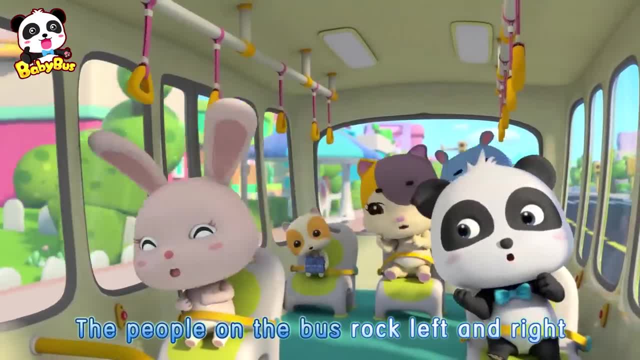 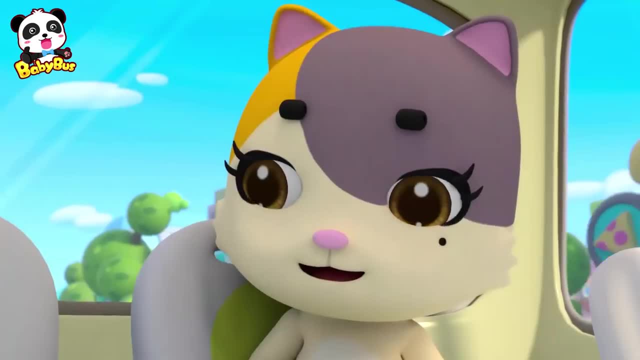 The wheels on the bus go round and round, The people on the bus rock left and right. We will be there, yeah, yeah, We will be at the next stop. Ding ding, ding. the bell is ringing. Who is getting off? 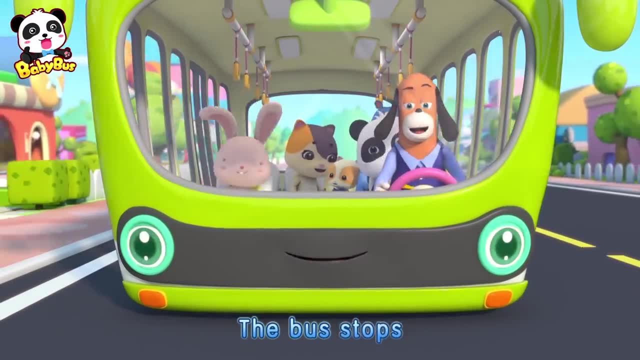 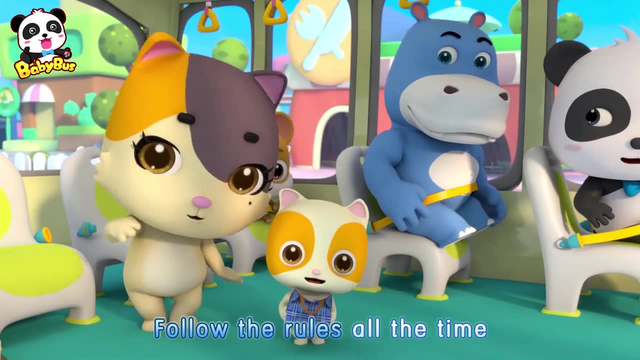 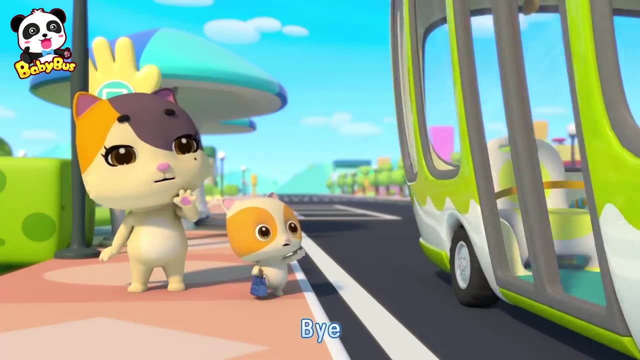 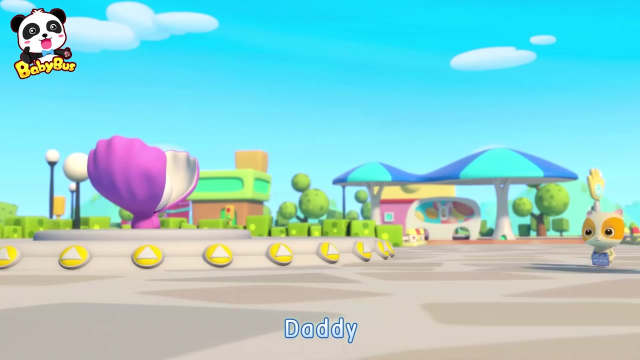 Me, me, The bus. the bus stops, stops. Who is getting off? Me, me. Wait until the bus stops. Follow the rules all the time And say thank you when you leave. Bye, Oh, Timmy, Daddy, Daddy. 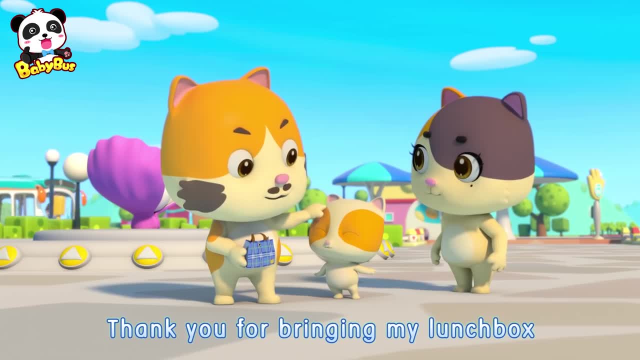 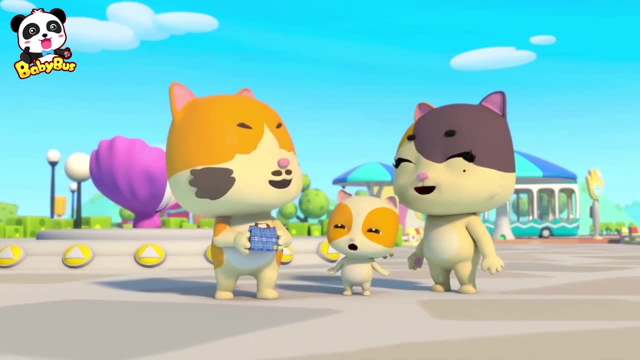 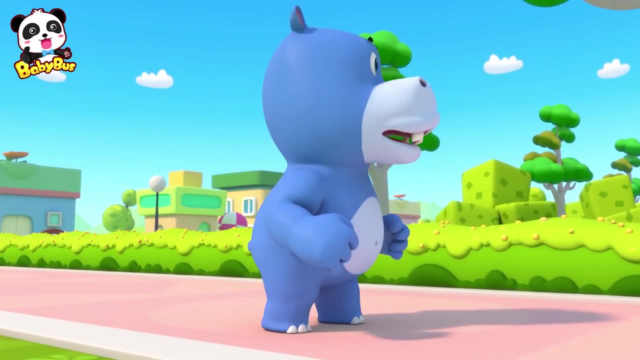 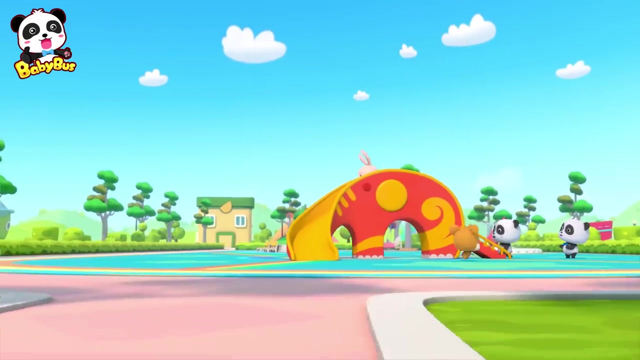 Your lunchbox, Timmy. thank you for bringing my lunchbox. I took a bus here. Good job, Timmy. Ha ha ha, Huh, Huh. Wow, it's a slide. I love it. He, he, he, he. 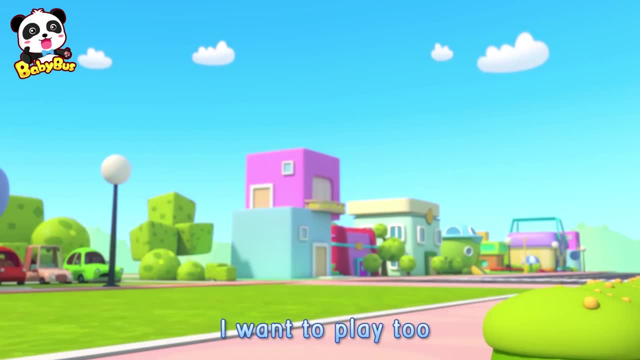 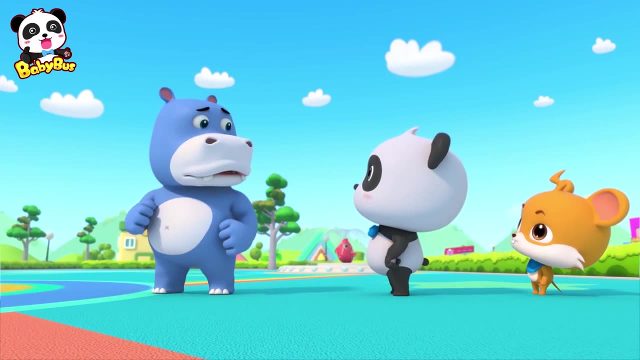 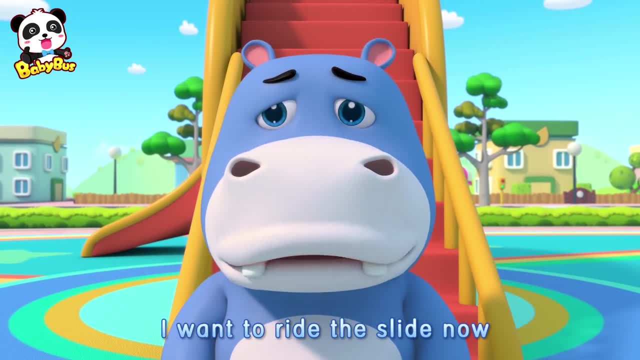 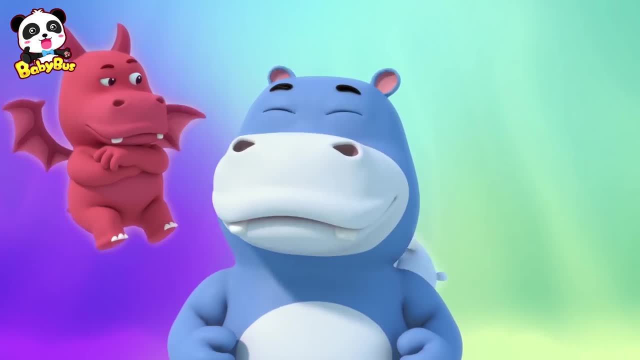 Why do I have to? I want to ride the slide now. He, he, he. You don't have to, You can ride the slide right now. Mm-hmm, It won't take long. If you line up, everyone can have fun together. 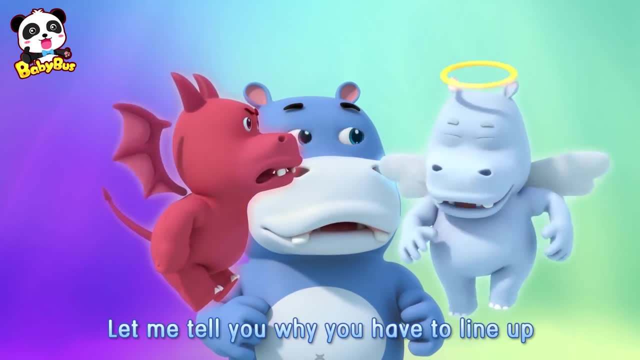 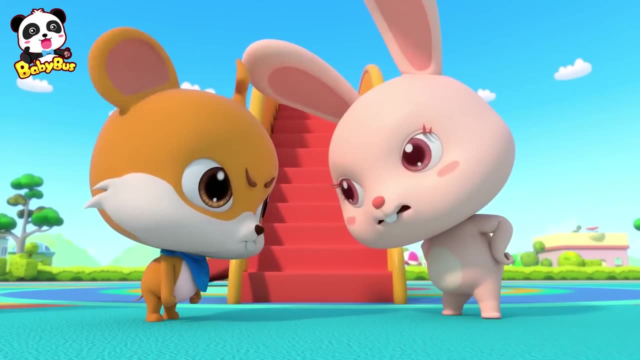 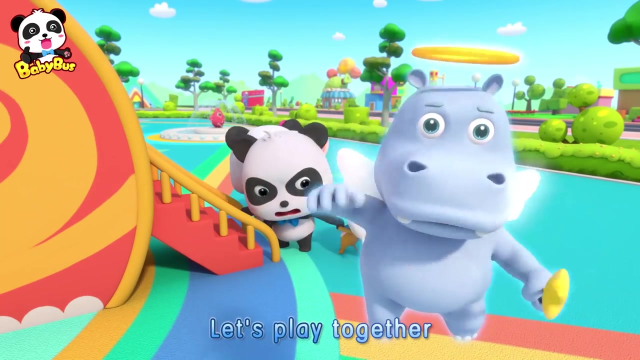 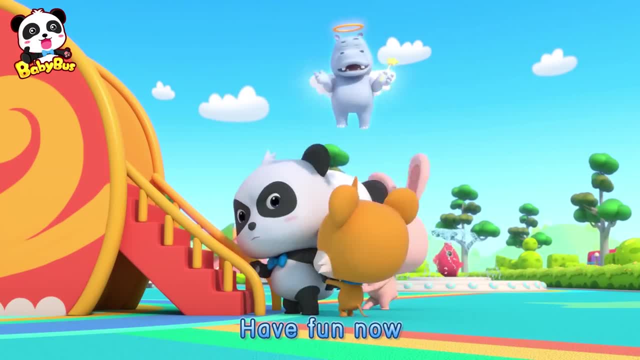 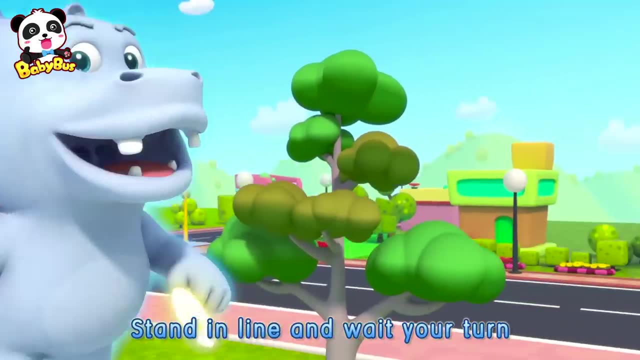 Line up, Oh, line up. Have fun now. Let's play together. Let's play together. Stand in line and wait your turn. Stand in line and wait your turn. Let's play together. Stand in line and wait your turn. 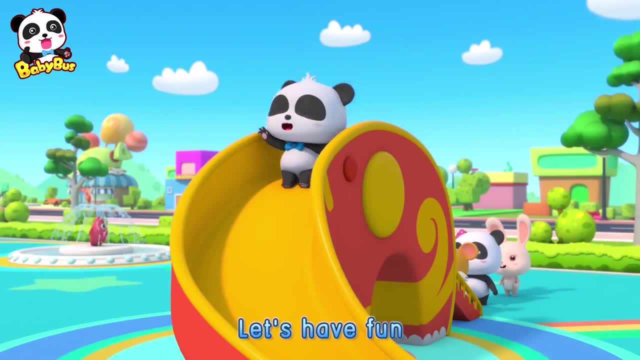 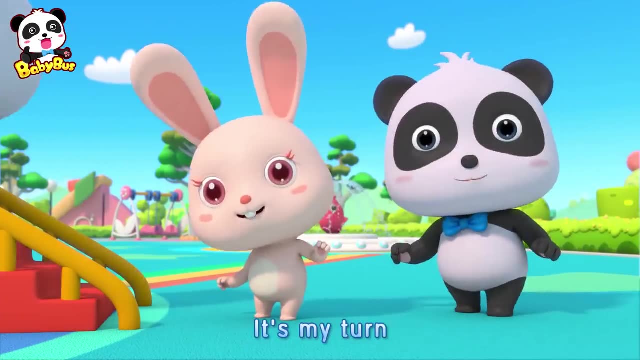 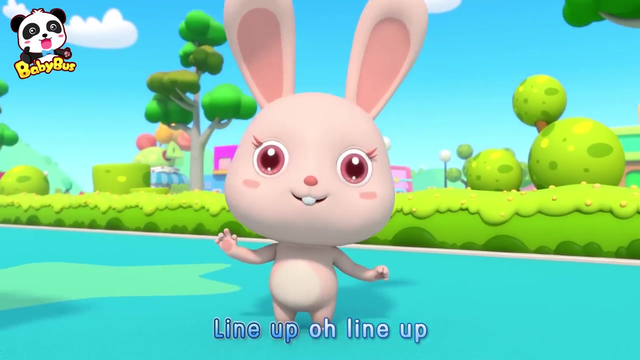 One and then another. Let's have fun. Let's play together. Please wait, don't be angry. Next one and next one. It's my turn. Let's play together, Do not push your friends. Line up, Oh, line up. 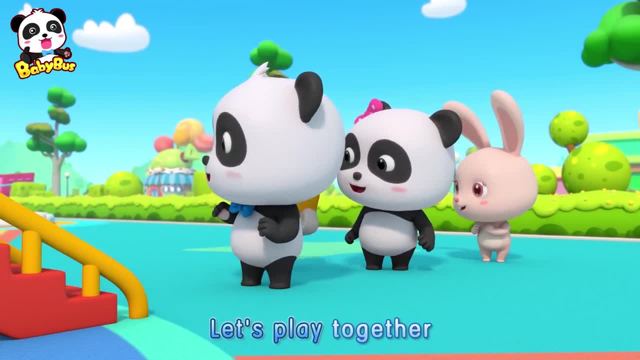 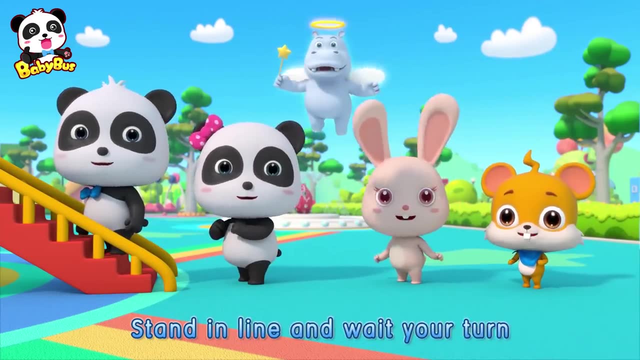 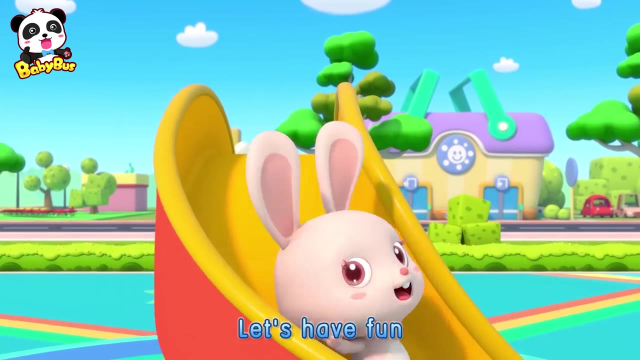 So much fun. Let's play together. Let's play together. Stand in line and wait your turn. Stand in line and wait your turn. Let's play together. Stand in line and wait your turn. One and then another. Let's have fun. 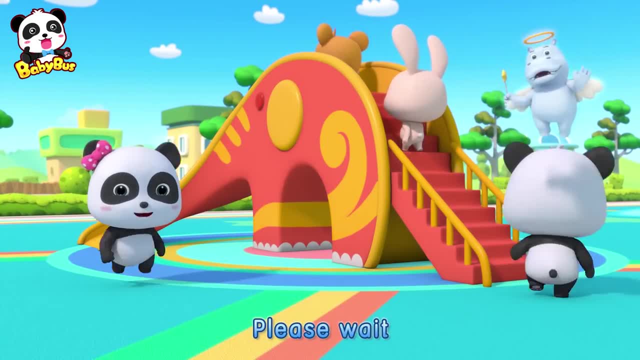 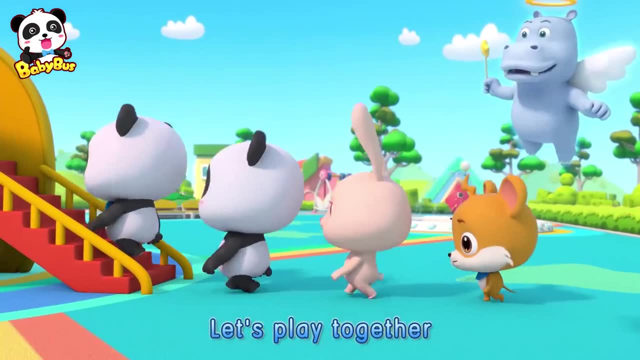 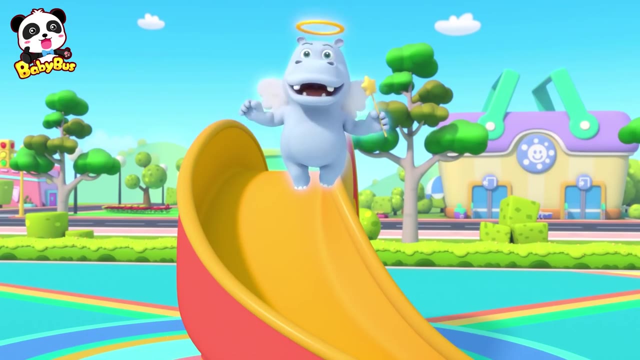 Let's play together. Please wait, don't be angry. Next one and next one. It's my turn. Let's play together. Let's play together. Stand in line and wait your turn. You can have so much fun. You can have so much fun. 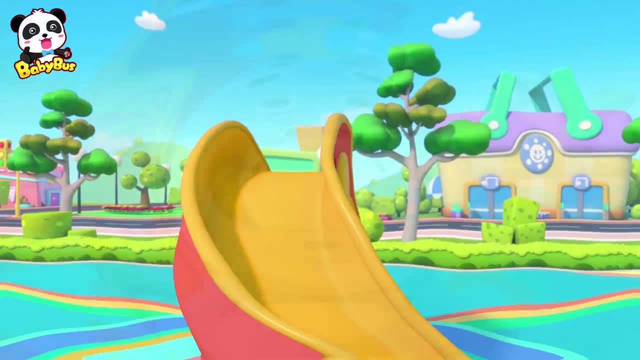 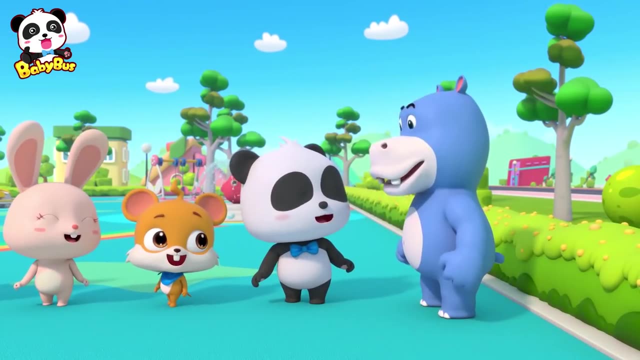 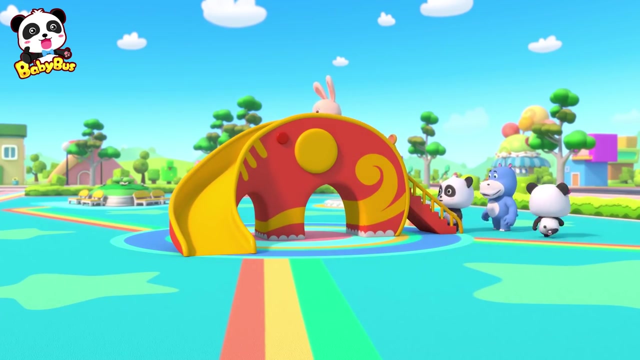 I said you don't have to line up. I said you don't have to line up. Alright, I will line up. Alright, I will line up. Yeah, I think we both might be good at this. Let's play together. 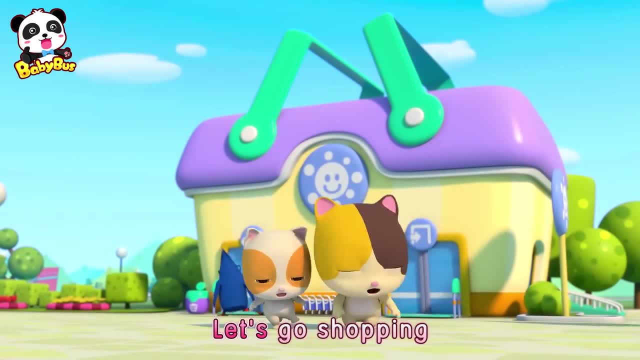 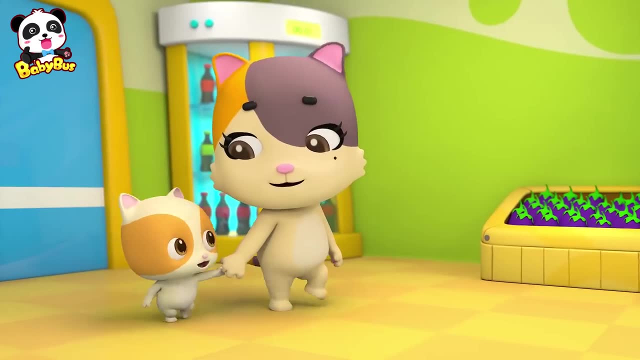 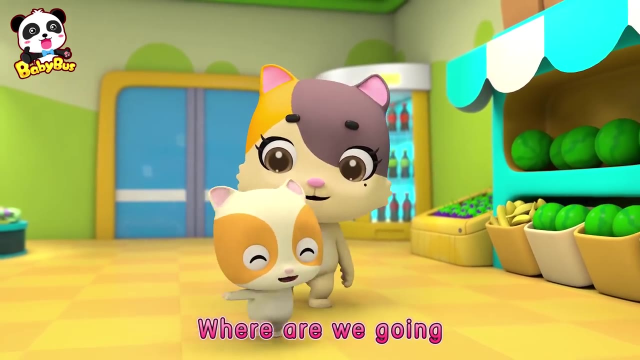 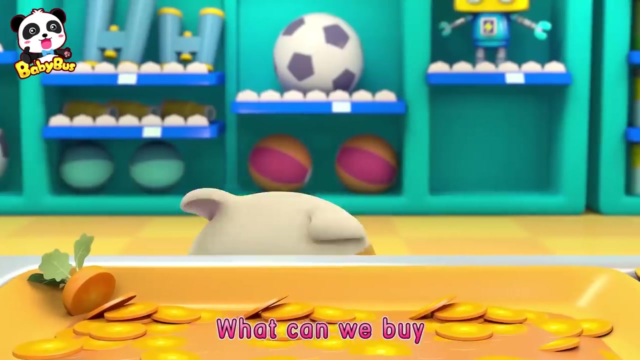 LEE BAAAY, I am so glad we made it. Let's play together Really. Yes, Let's stop. Oh yeah, I thought so. Let's play together. SONY, SONYY, SONYY, SONYY. 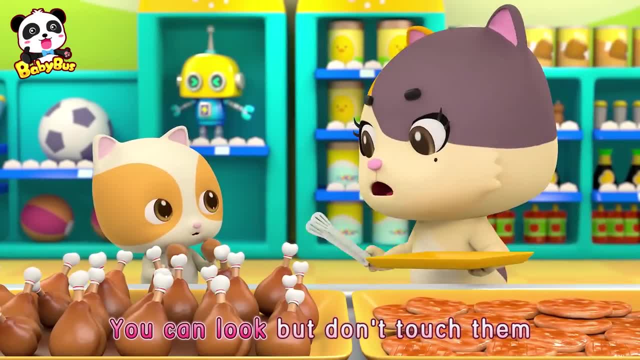 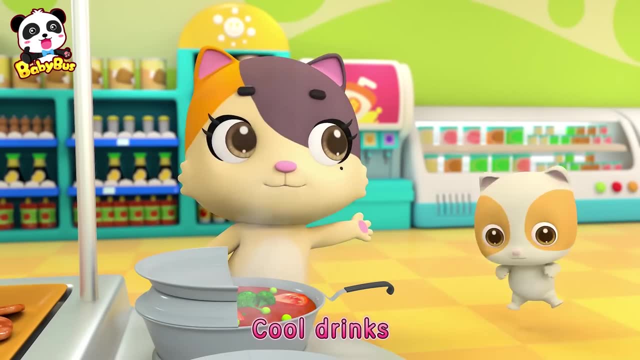 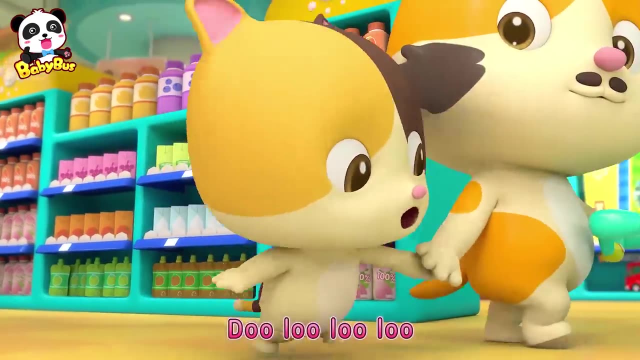 Something to buy, You can look, but don't touch them. Yummy bread, sweet cake- Just look, don't touch. Hot soup, cool drink- Just look, don't touch. Just look, don't touch Tilly-tilly-lilly-lilly hand in hand. 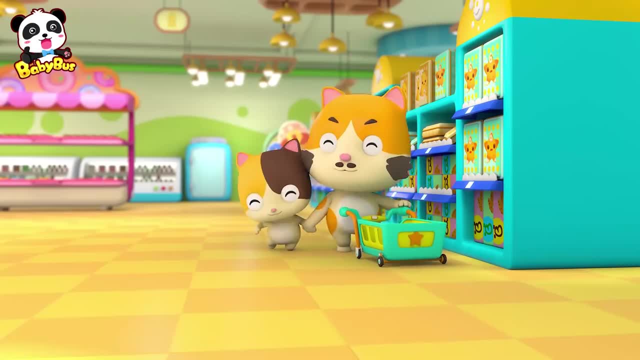 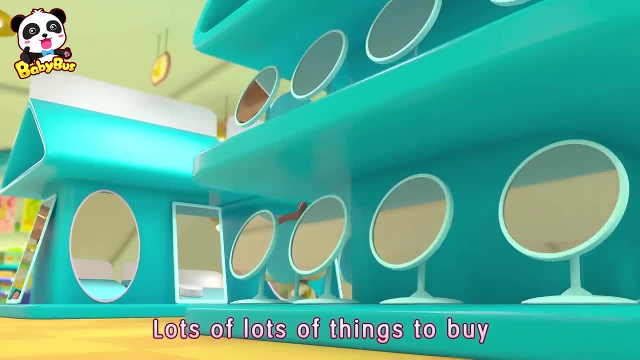 Yippee-yippee, hand in hand. Where are we going, Sha-la-sha-la-la, let's look around. Whoa, Whoa. What can we buy? Lots of, lots of things to buy. You can look, but don't touch them. 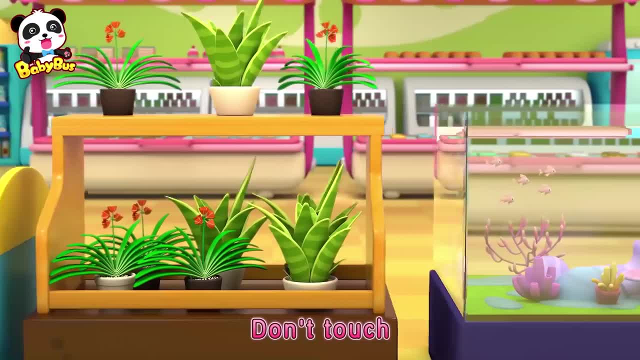 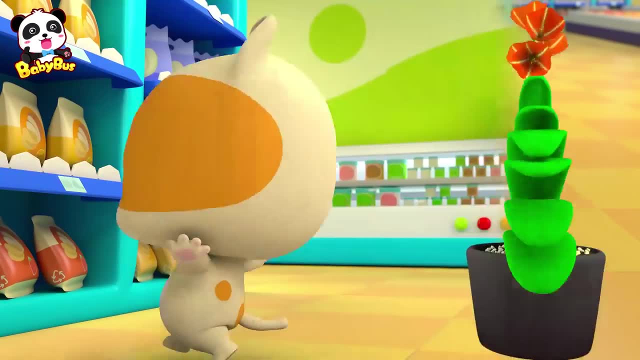 Round plates, tall glasses- Just look, don't touch. Little pots, fish tanks- Just look, don't touch. Just look, don't touch. Tilly-tilly-lilly-lilly, hand in hand, Yippee-yippee, hand in hand. 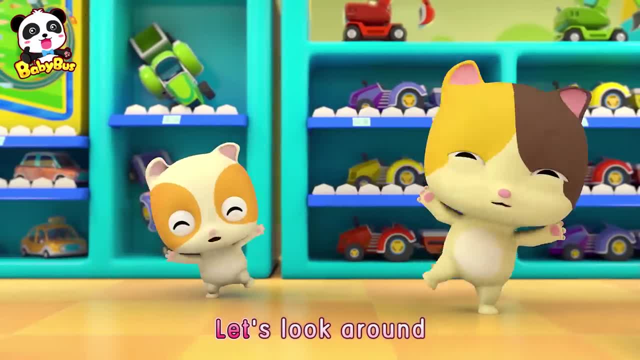 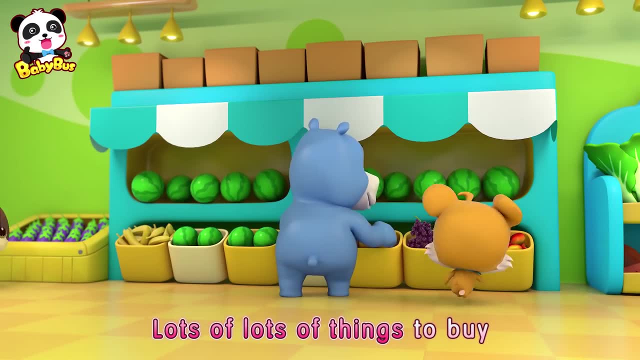 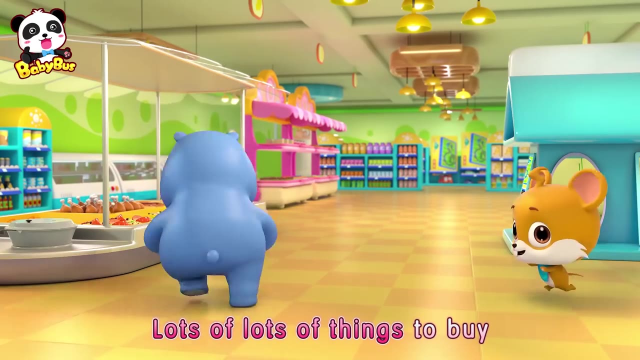 Where are we going? Sha-la-sha-la-la, let's look around. Whoa, Whoa. What can we buy? Lots of lots of things to buy. You can look, but don't touch them. Lots of lots of things to buy. 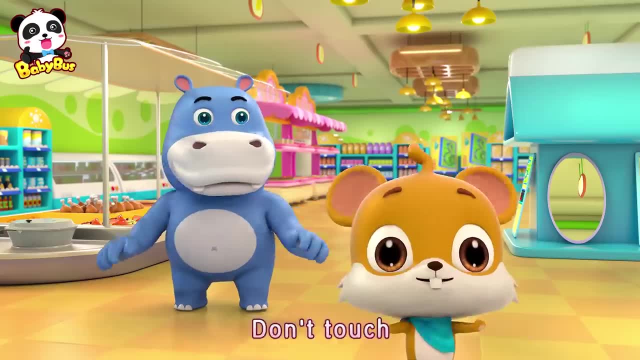 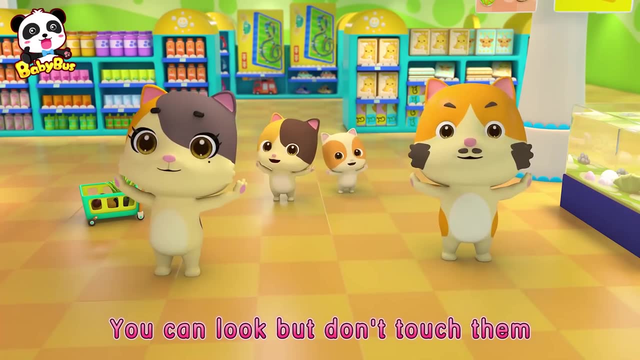 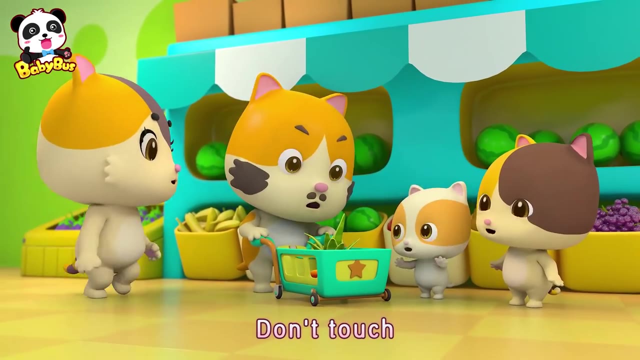 You can look, but don't touch them. Tilly-tilly-lilly-lilly hand in hand. Sha-la-sha-la-la, let's go shopping. You can look, but don't touch them. Just look, don't touch Tilly-tilly-lilly-lilly hand in hand. 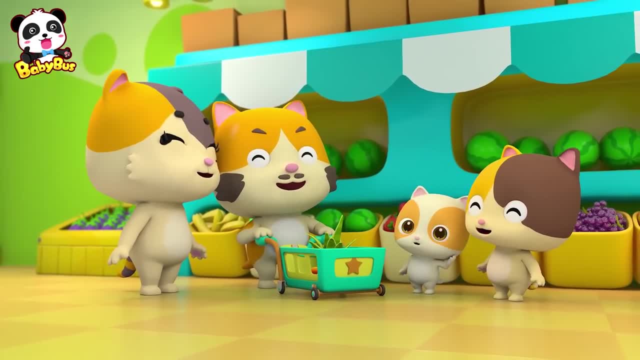 Whoa, What can we buy? Just look, don't touch them. Where are we going? Just look, don't touch them. Hey Hank, Wake up, let's go outside. Hey Hank, Wake up, let's go outside. 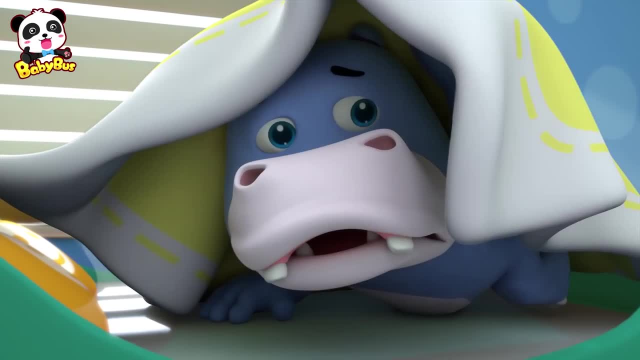 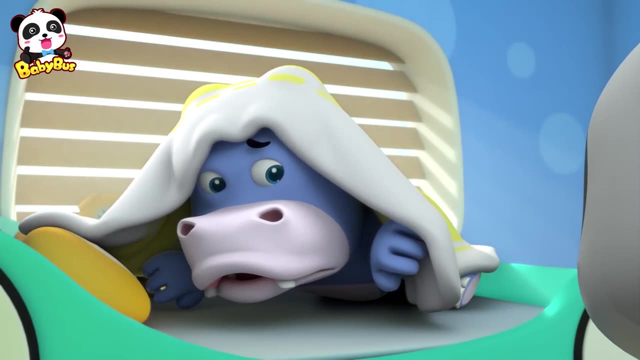 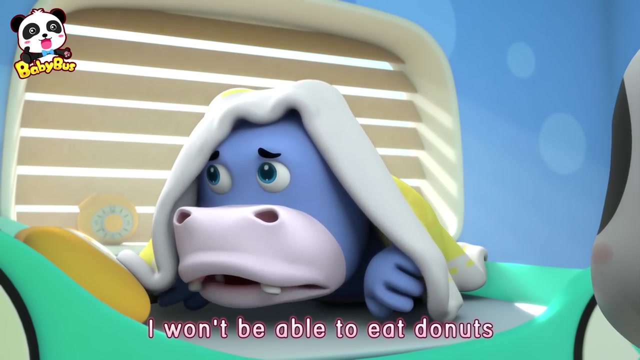 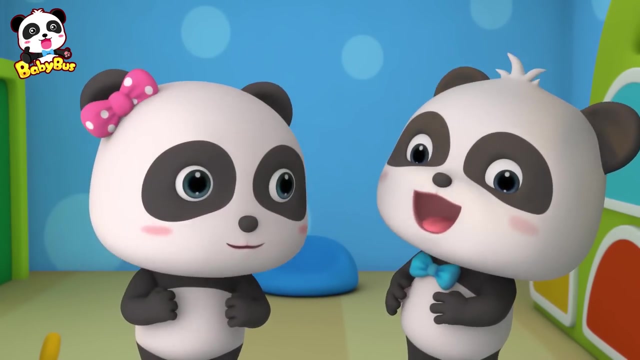 Hey, Hank, Wake up, let's go outside. What's wrong with you, Hank? I don't want to go out. it's so cold. If I catch a cold, I won't be able to eat doughnuts. Hank, if you don't want to catch a cold, you shouldn't stay in your bed. 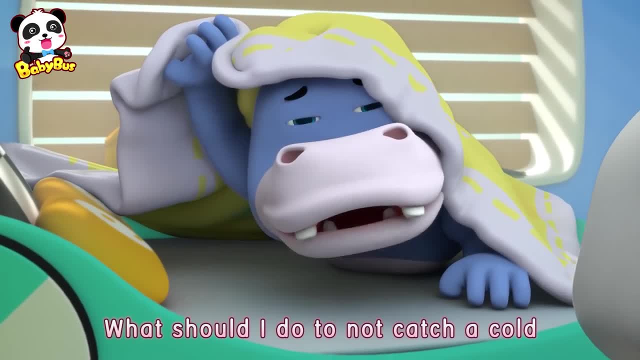 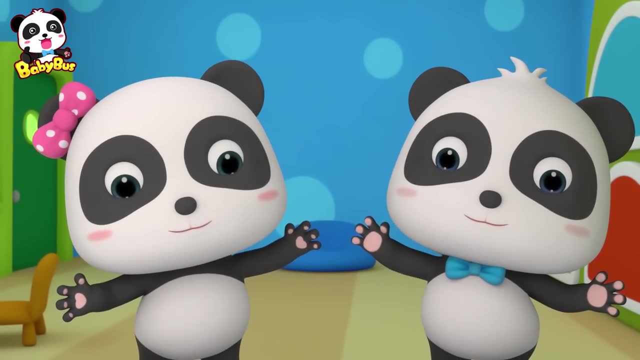 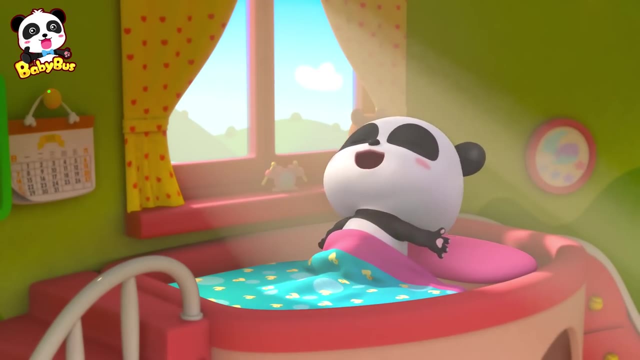 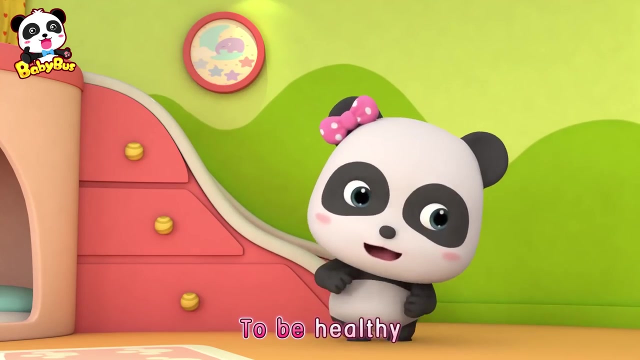 Right, What should I do to not catch a cold? Follow our directions, Then you can prevent a cold. Oh, please do as I do. Everyone, everyone. Oh, please do as I do To be healthy. Get up early every day, Enjoy the warm and bright sunshine. 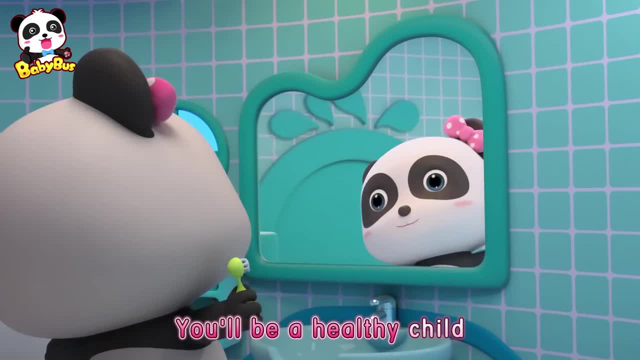 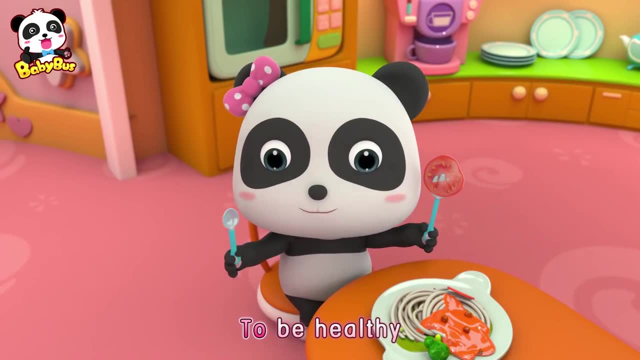 It's so fresh, it's so good. You'll be a healthy child. Oh, please do as I do Everyone, everyone. Oh, please do as I do: Everyone, everyone, Everyone, everyone. To be healthy, You should eat every day Lots of fruits and vegetables. 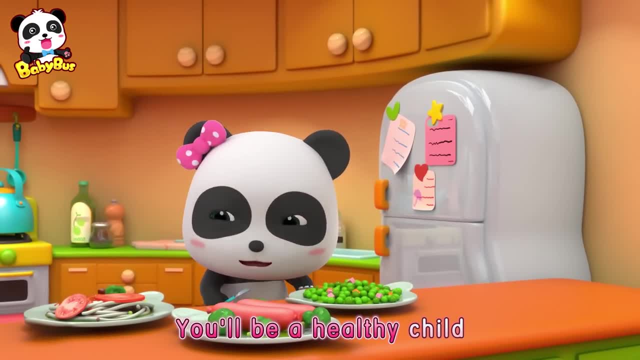 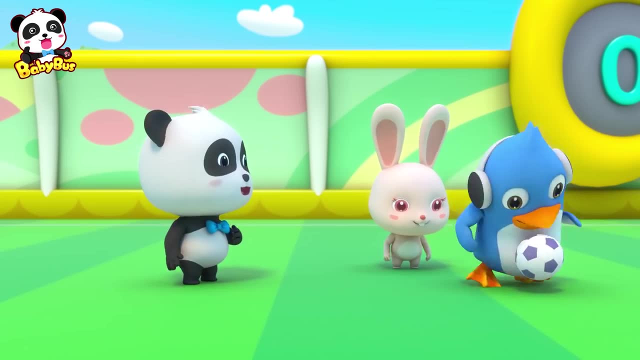 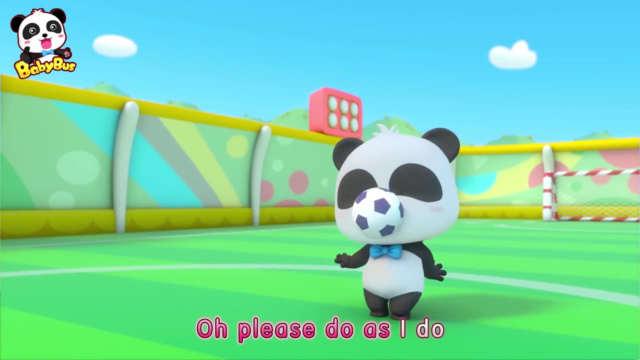 It's so fresh, it's so good. You'll be a healthy child. Oh, please do as I do. Everyone, everyone. Oh please do as I do. To be healthy, Have fun every day and play Soccer in the field. Oh, please do as I do. 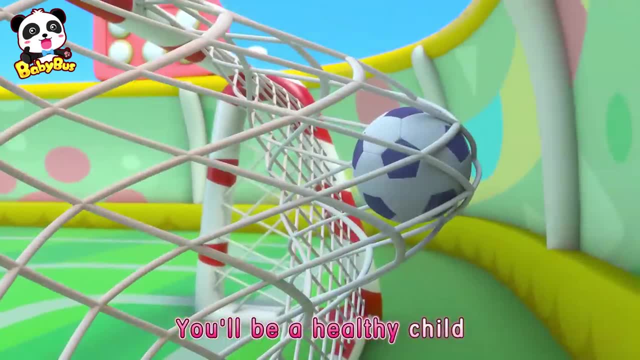 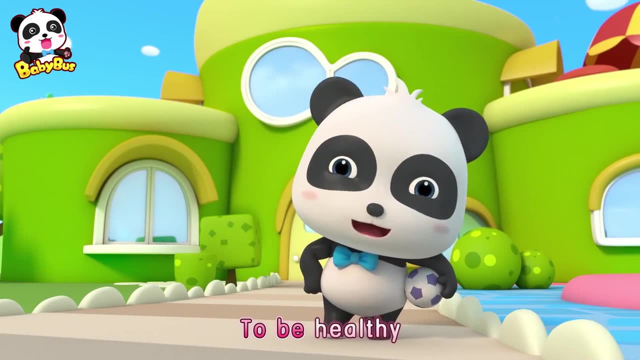 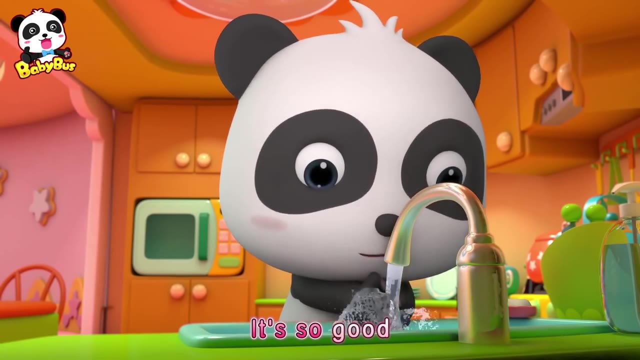 It's so fun, it's so good. You'll be a healthy child. Oh, please do as I do. Everyone, everyone. Oh, please do as I do To be healthy, Wash your hands with soap Every time you come back home. It's so clean, it's so good. 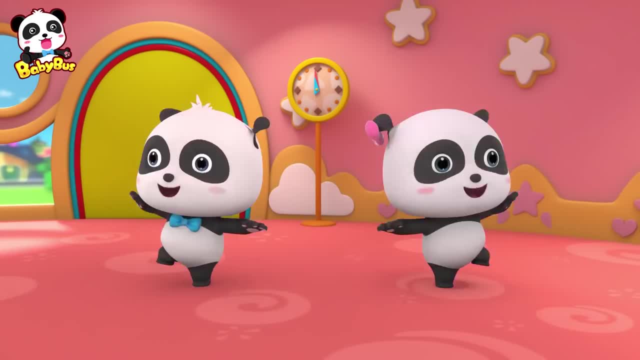 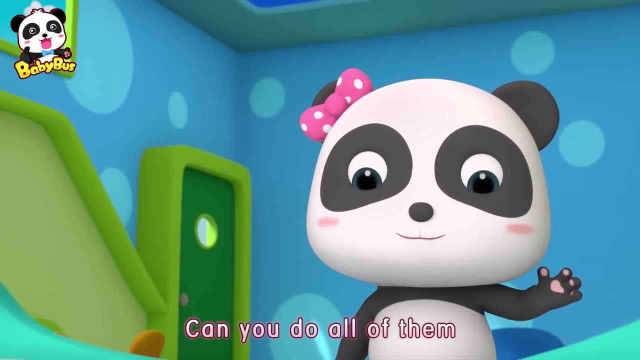 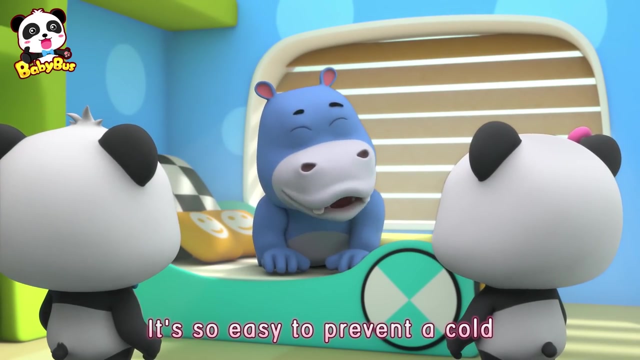 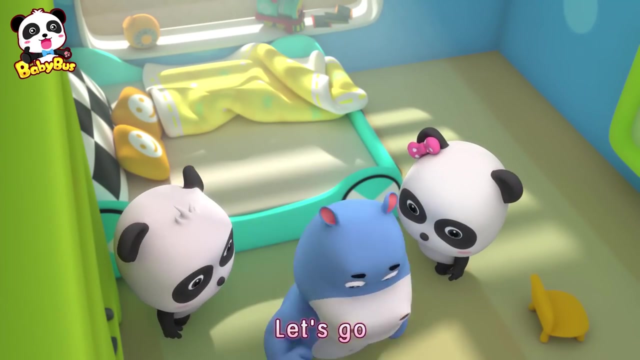 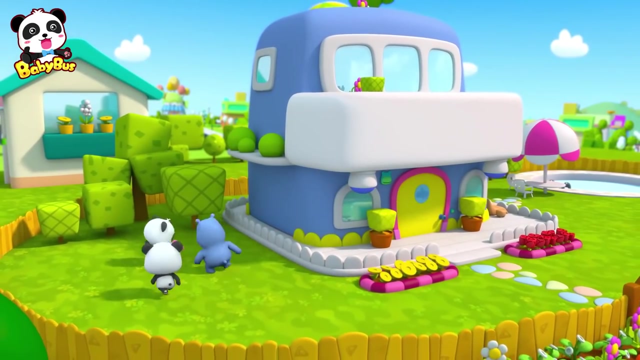 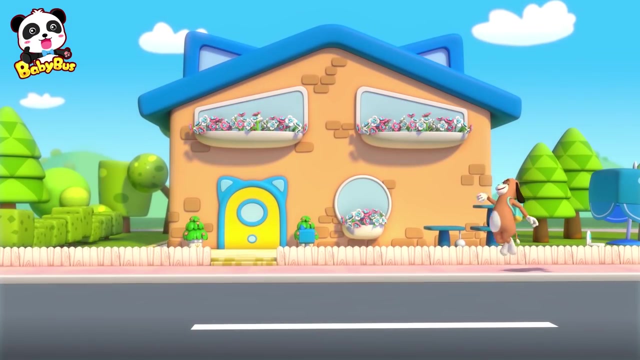 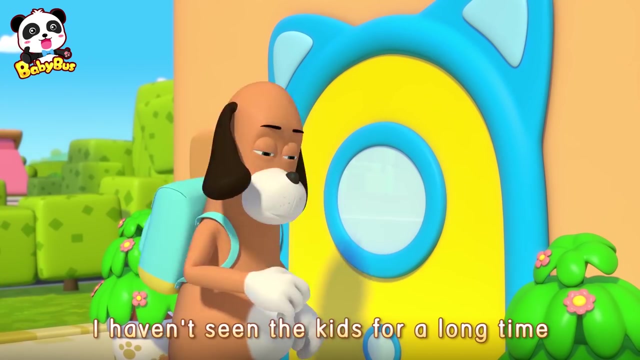 You'll be a healthy child. Hank, can you do all of them? Yes, I can. Yes, I can. It's so easy to prevent a cold. Are you ready to go out with us? Sure, let's go. Yeah, Oh, I haven't seen the kids for a long time. 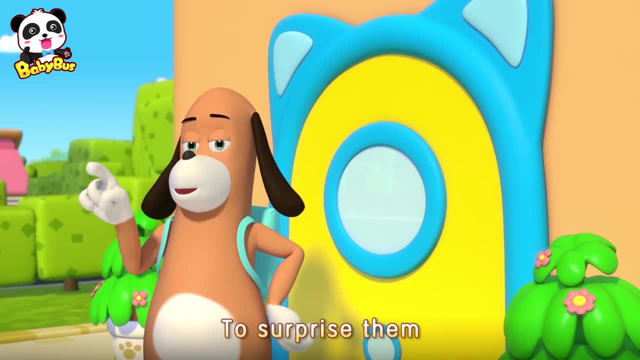 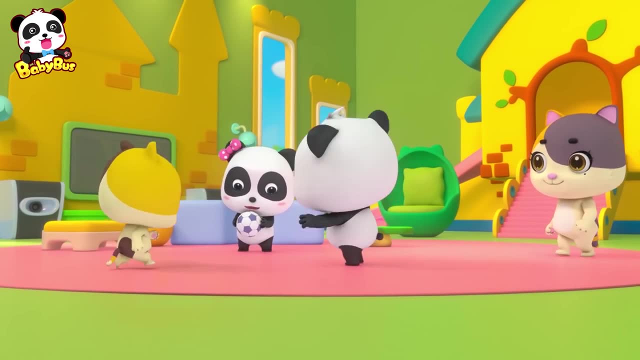 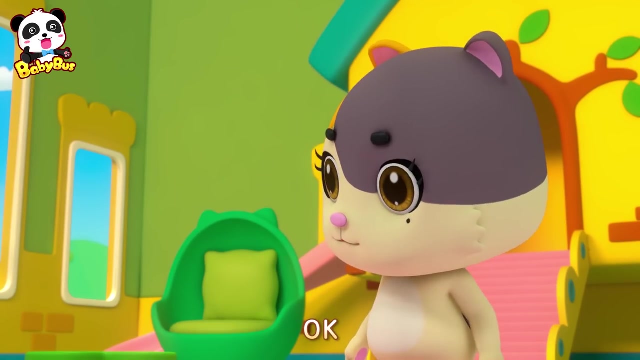 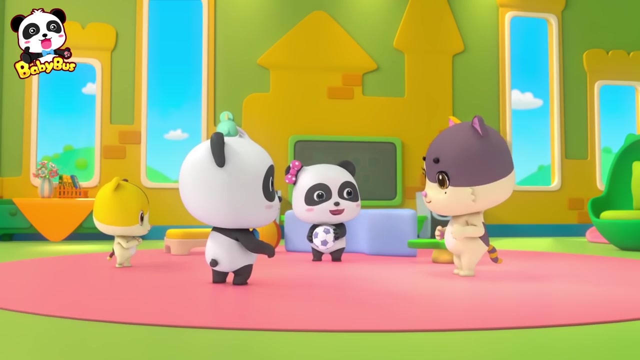 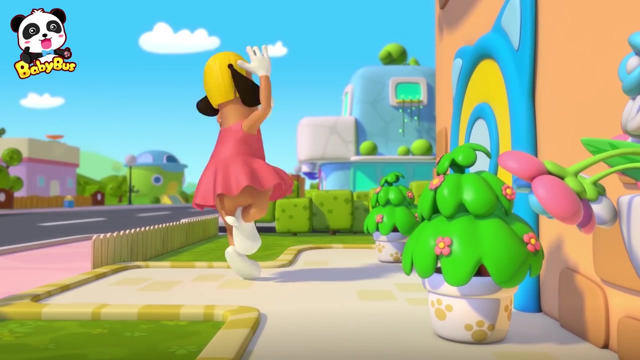 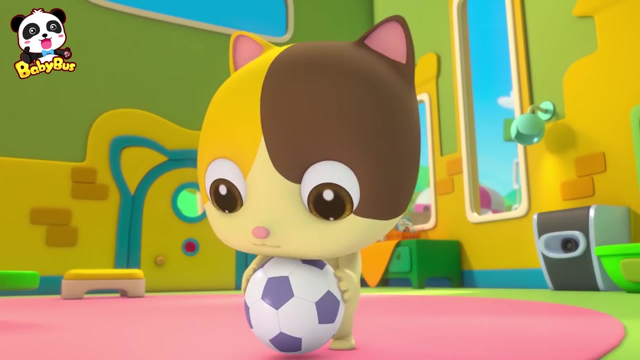 Oh, I'll disguise myself as someone else to surprise them. Kids, I'll go upstairs to clean the room now. Never open the door for a stranger, okay, Don't worry, we won't. Who's knocking on the door? Knock, knock on the door. 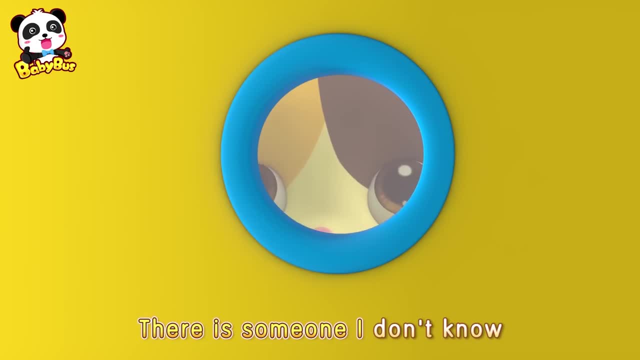 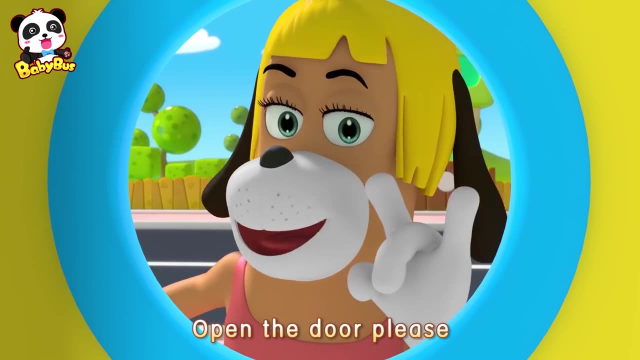 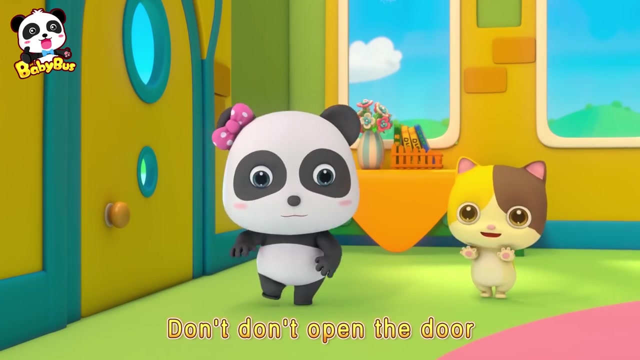 See who's knocking on the door. There is someone I don't know. Can I open the door for him? Who is it? Open the door, please. Open the door please. Who is she? Her voice sounds so weird. Don't, don't open the door. 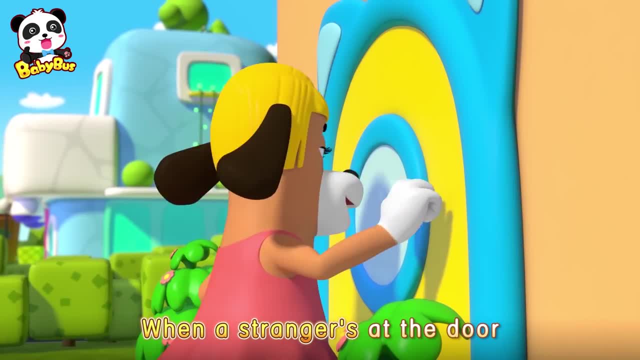 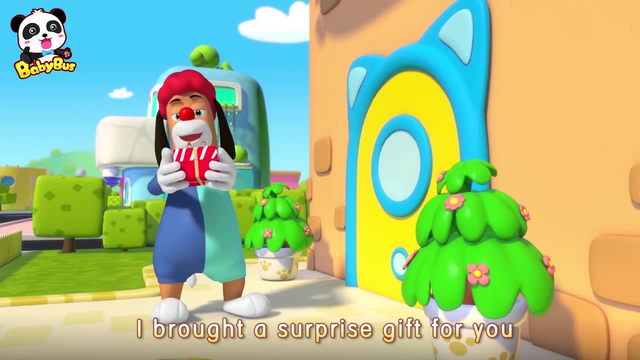 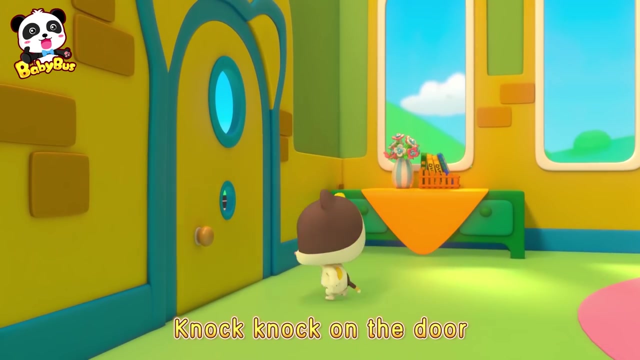 That's what mom and dad say When a stranger's at the door. Never open the door for him. Kids, I brought a surprise gift for you. Open the door, Knock, knock on the door. See who's knocking on the door. There is someone I don't know. 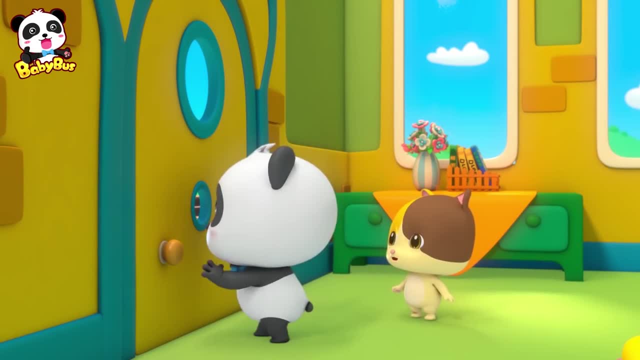 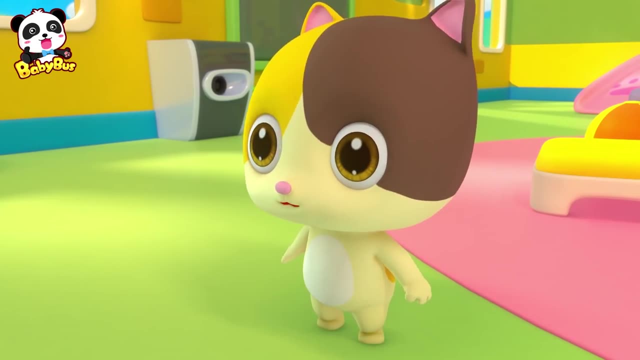 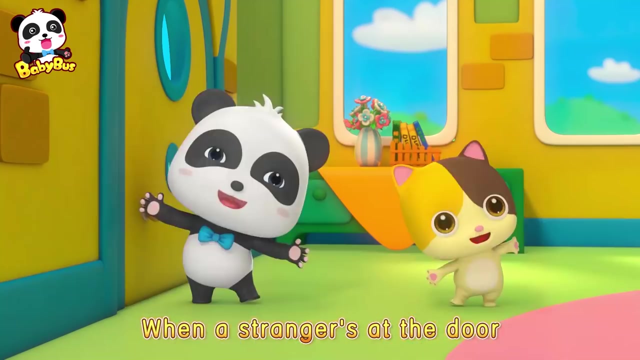 Can I open the door for him? Can I open the door for him? He's a clown, Mimi. do you know him? Don't, don't open the door. That's what mom and dad say When a stranger's at the door. Never open the door for him. 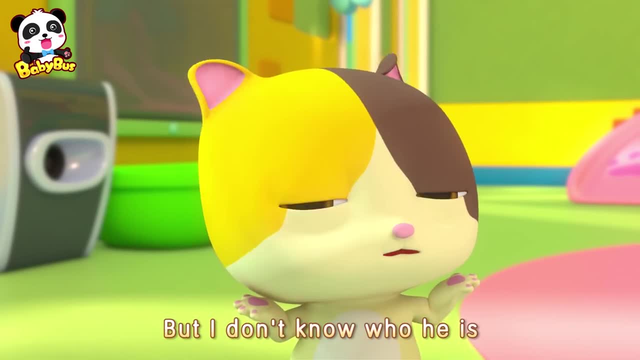 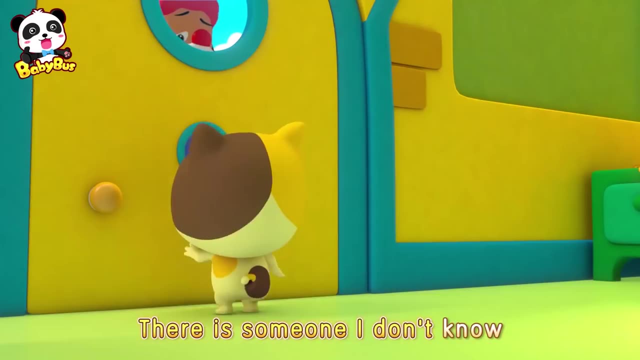 Mimi, please. He knows my name, but I don't know who he is. Knock, knock on the door. See who's knocking on the door. There is someone I don't know. Can I open the door for him? Don't, don't open the door. 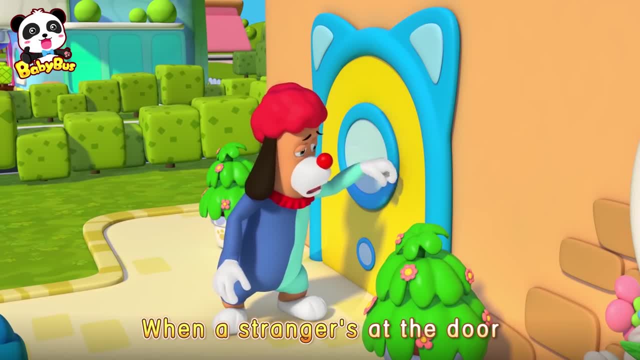 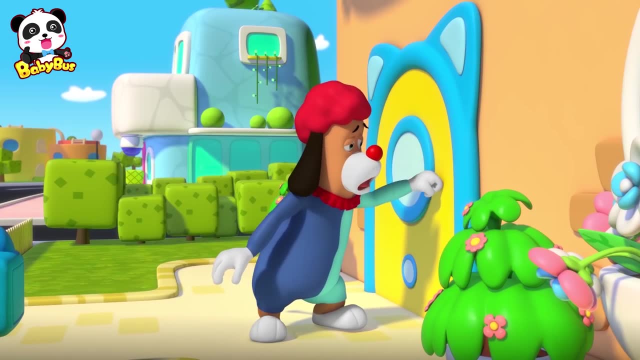 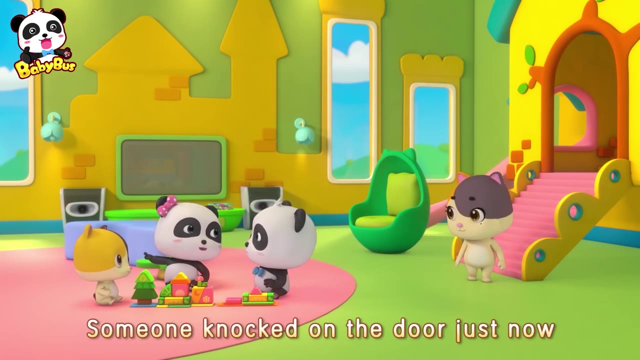 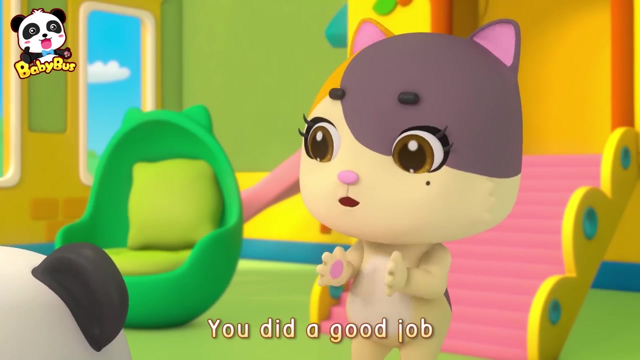 That's what mom and dad say. When a stranger's at the door, Never open the door for him. Huh, Ma'am, someone knocked on the door just now. It was a stranger, So we didn't open the door. You didn't open the door. 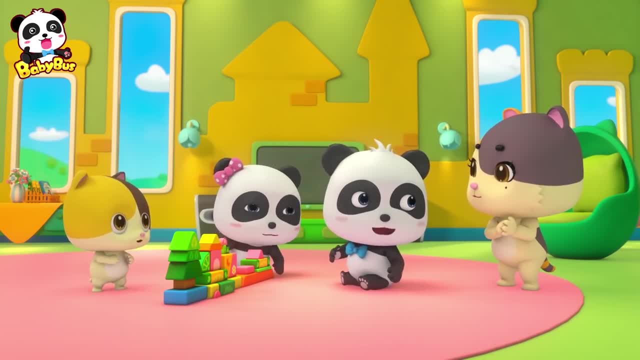 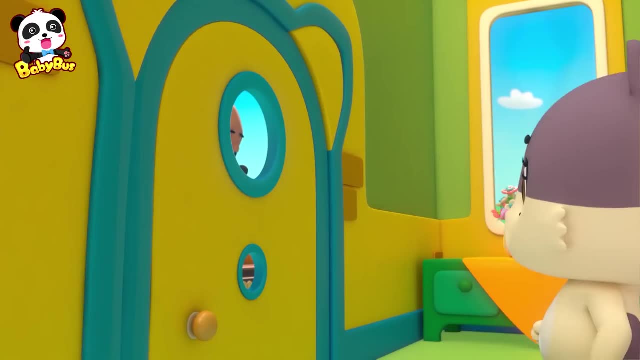 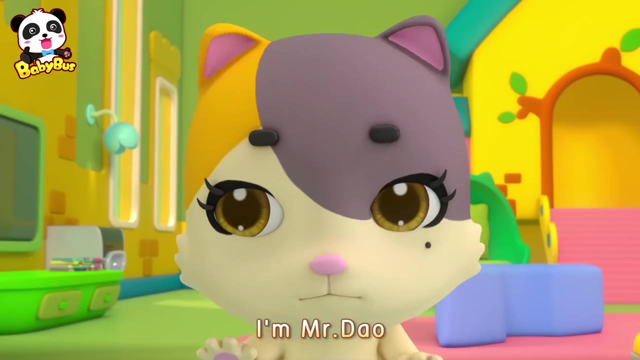 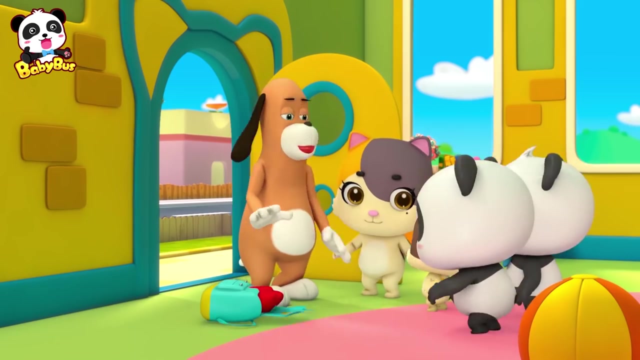 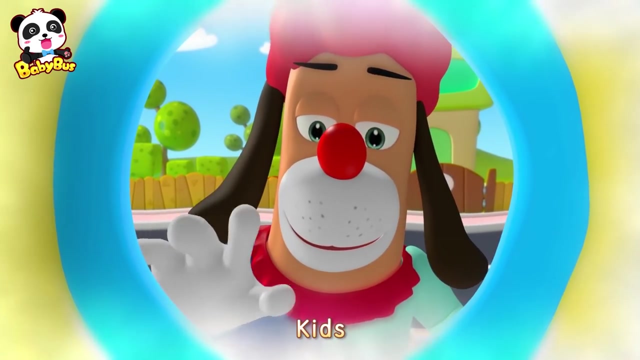 Good job. Never open the door for a stranger. Who is it? Let me go see, Open up. I'm Mr Dow. He is Mr Dow. Why did you take so long to open the door? Come on in, Mr Dow Kids. It was you who knocked on the door. 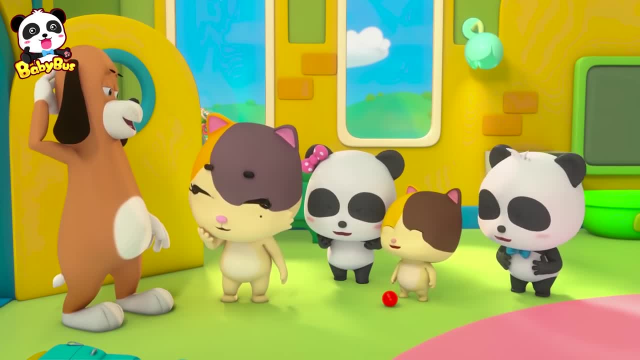 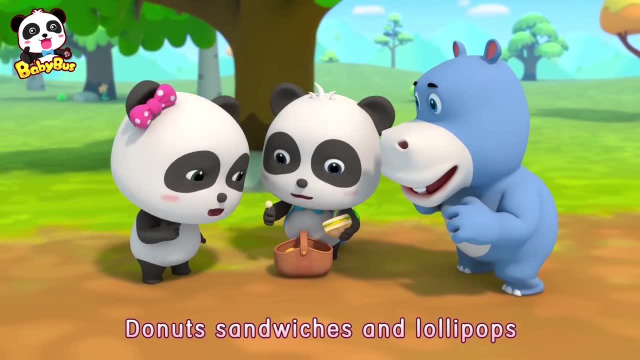 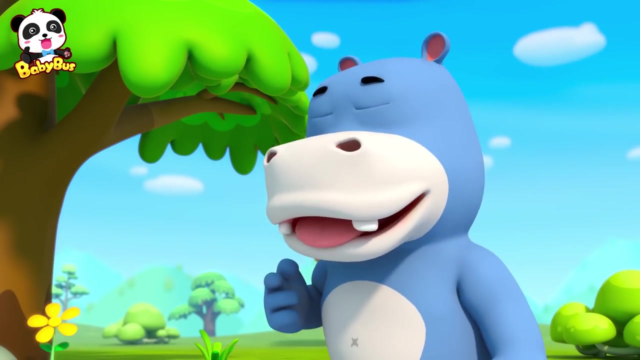 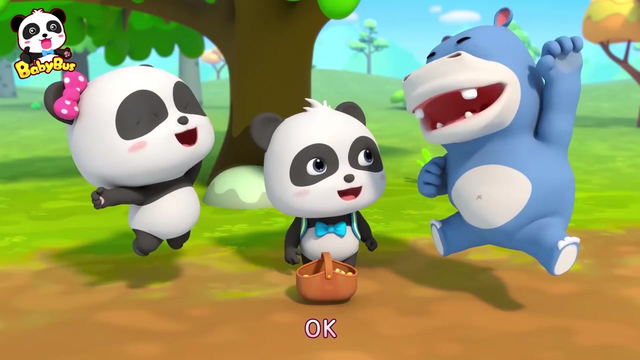 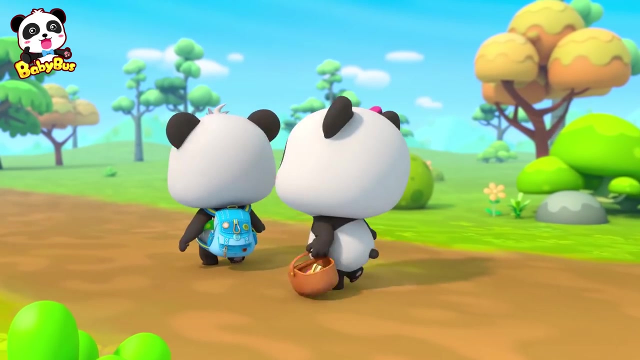 Knock, I brought a lot of food. Wow, donuts, sandwiches and lollipops. Wow, I want to have some right now. Wait till we arrive at the park for picnic. Let's get going. Okay, A donut is falling down and rolling around. 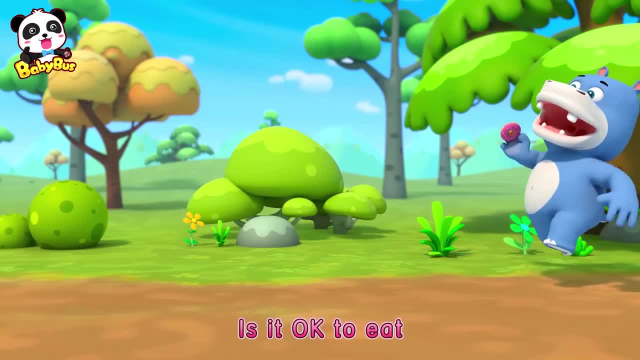 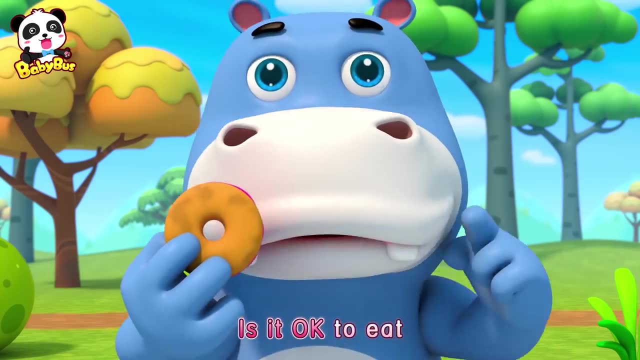 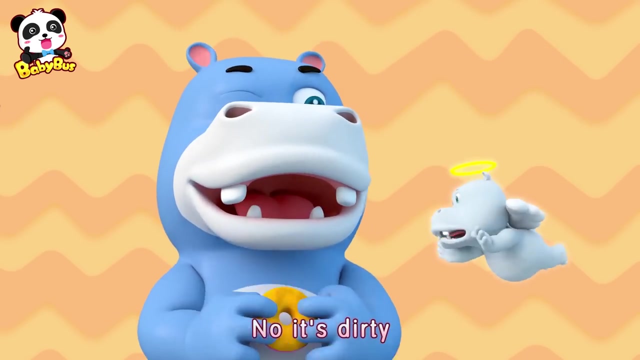 The donut on the ground isn't okay to eat. The yummy, yummy donut, I want to eat it, want to eat it. The donut on the ground isn't okay to eat. Let's eat it. Mm-hmm, Ah, No, it's dirty. 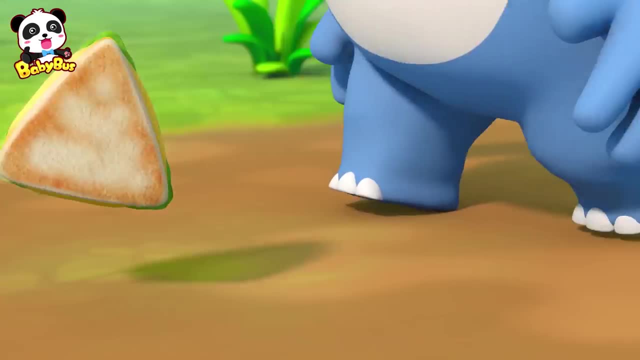 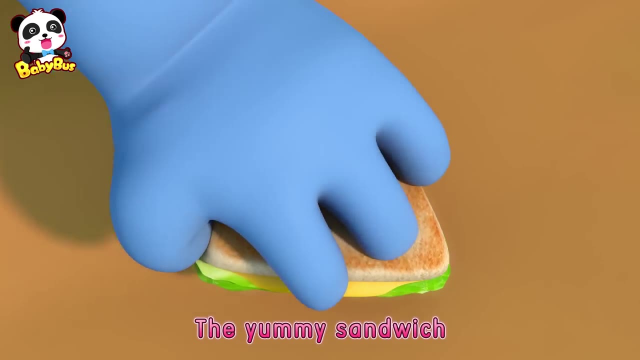 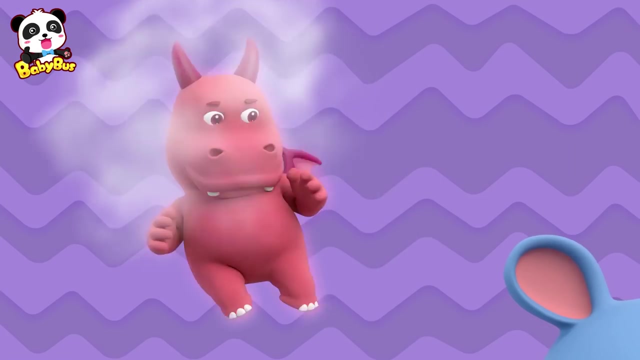 A sandwich is falling down and rolling around. The sandwich on the ground isn't okay to eat. The yummy sandwich. I want to eat it. want to eat it. The sandwich on the ground isn't okay to eat. Come on, eat it Okay. No, don't eat it. 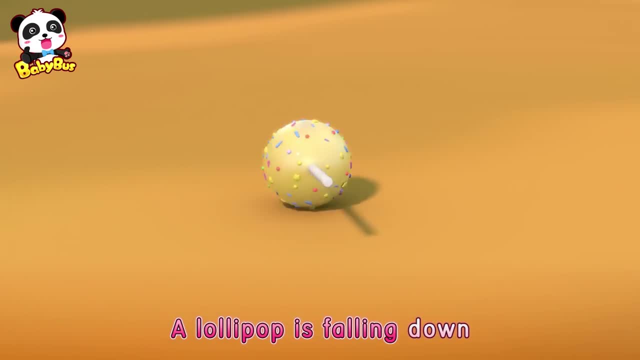 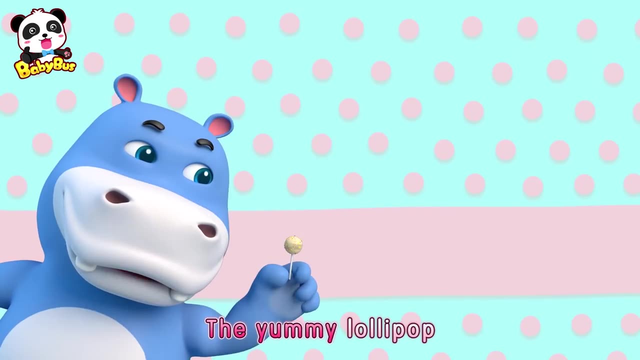 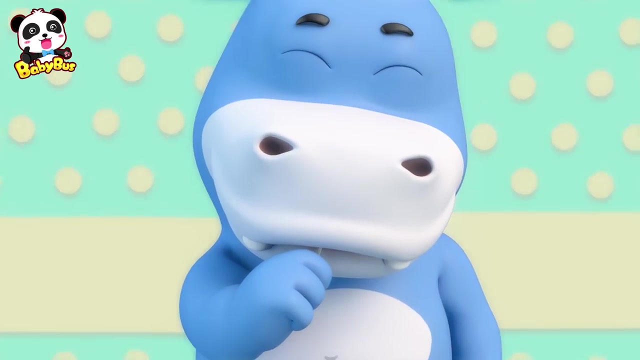 Ah, A lollipop is falling down and rolling around. The lollipop on the ground isn't okay to eat The yummy lollipop. I want to eat it. want to eat it. The lollipop on the ground. I put it in my mouth. The germs went into your tummy. 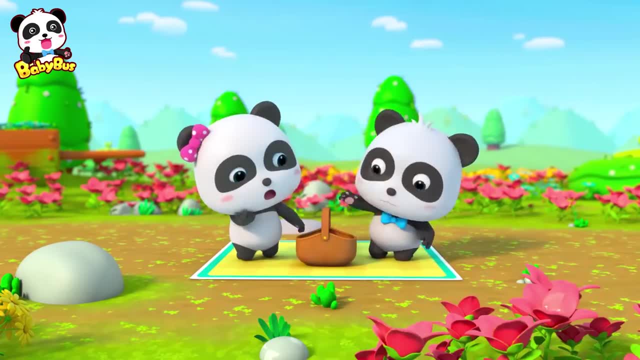 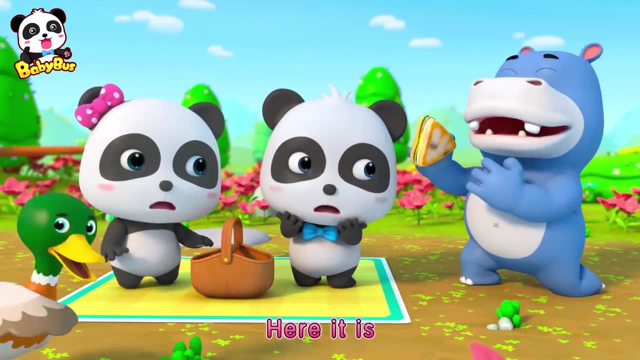 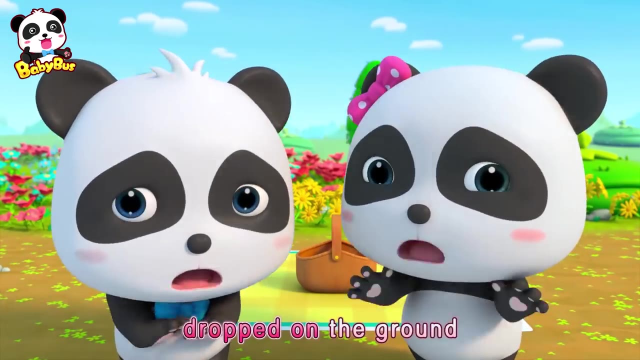 Oh no, Where is the donut? the donut, Here it is. Where is the sandwich? Here it is. Where is the lollipop, the lollipop pop, the lollipop in my tummy? you should not eat food dropped on the ground. 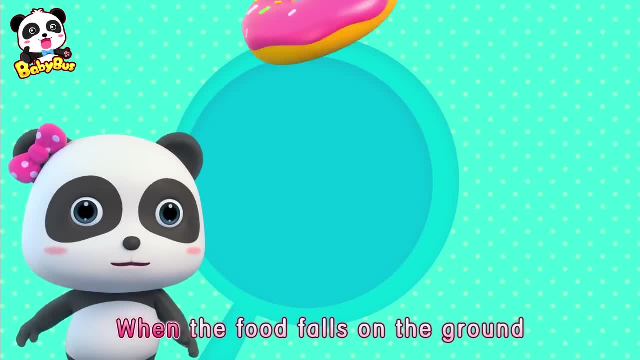 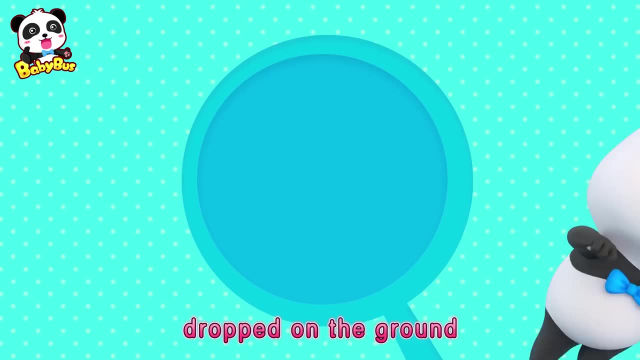 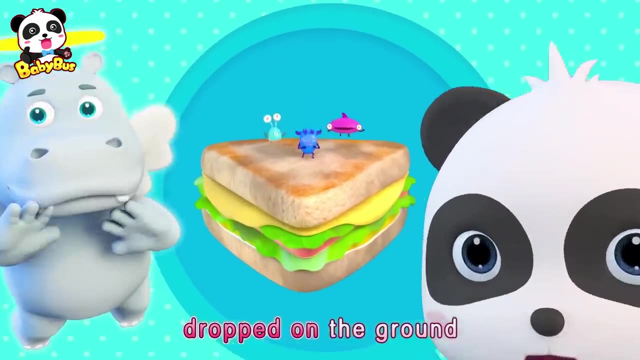 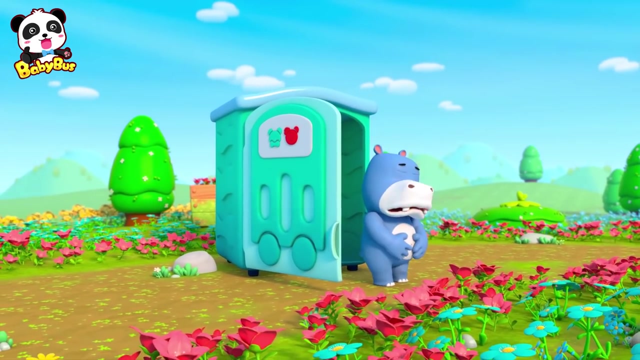 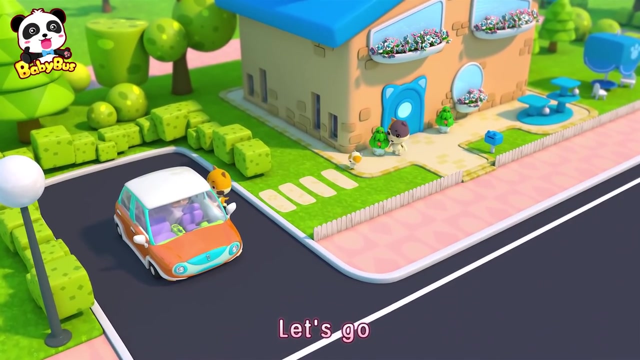 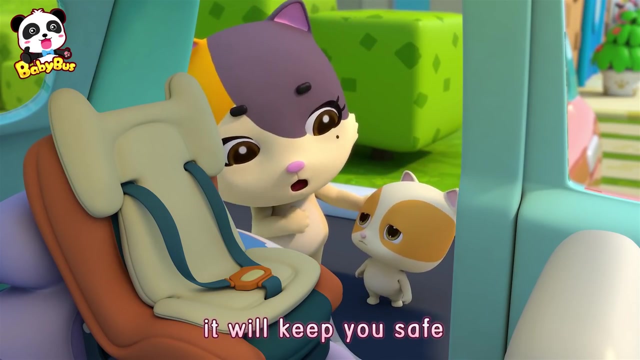 i feel sick in my tummy when the food falls on the ground. you should not eat food dropped on the ground. when the food falls on the ground. Yeah, let's go. I don't want to sit in the safety seat. Sweetie, it will keep you safe. 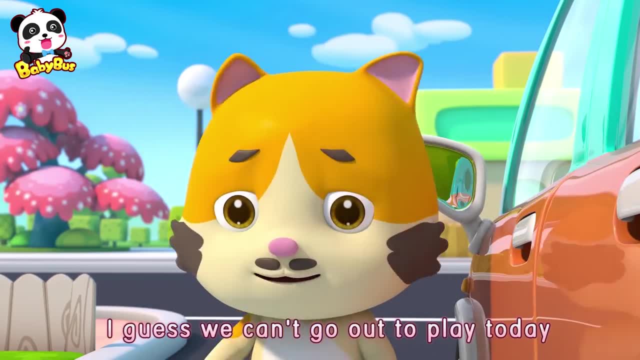 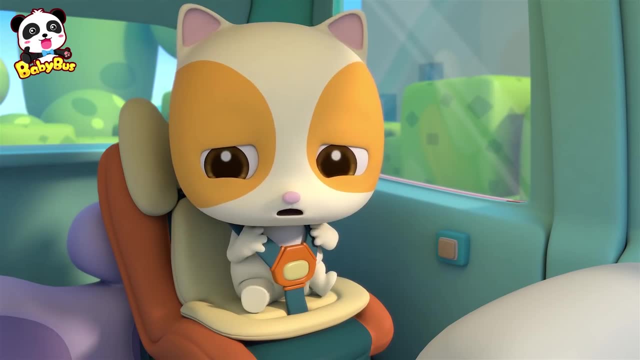 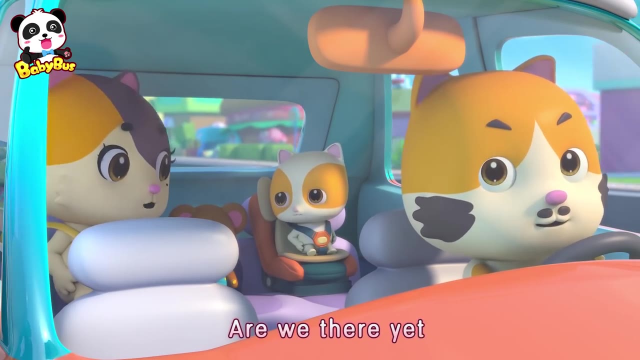 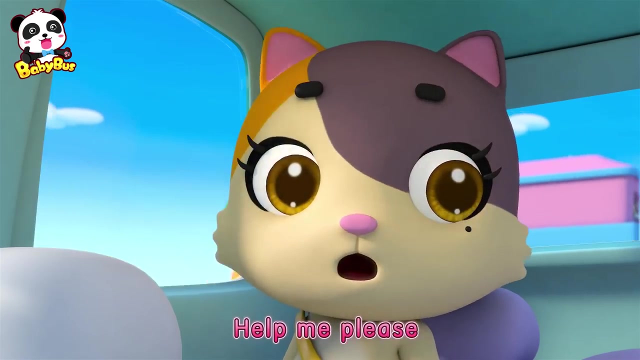 No, I don't want to. Well then, I guess we can't go out to play today, Mom, are we there yet? Not yet, Mommy. please, help me, please, Please, unbuckle my seatbelt. I don't like the safety seat. 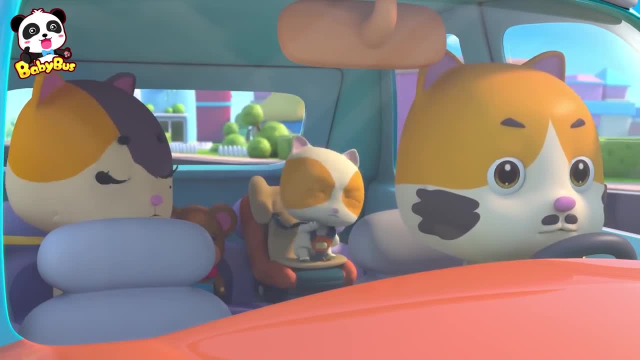 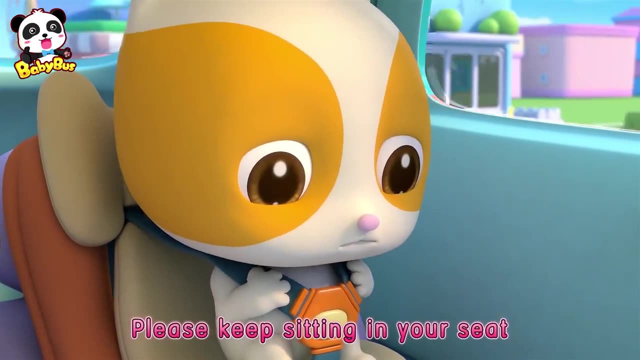 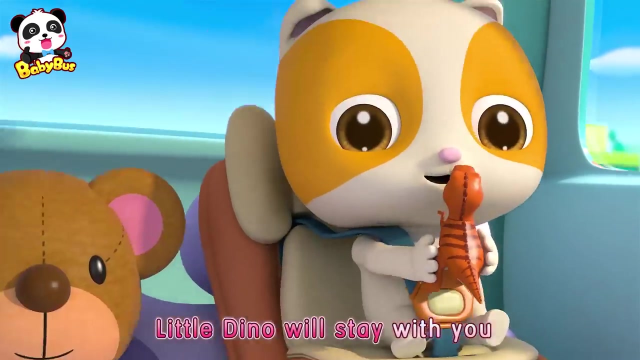 I want to get out of it. Sweetie, sweetie, sit up straight. Please keep sitting in your seat. Look what Mommy brought here for you. Wow, little dino, Little dino will stay with you. Here comes a curve. 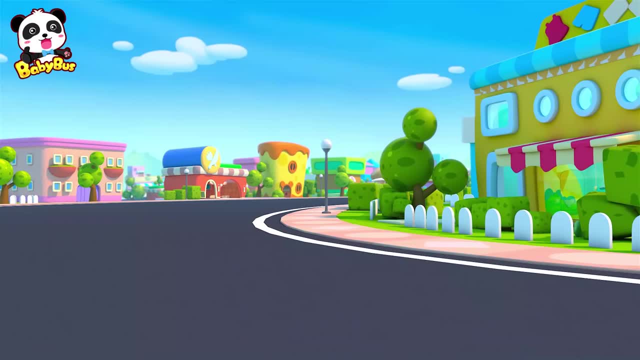 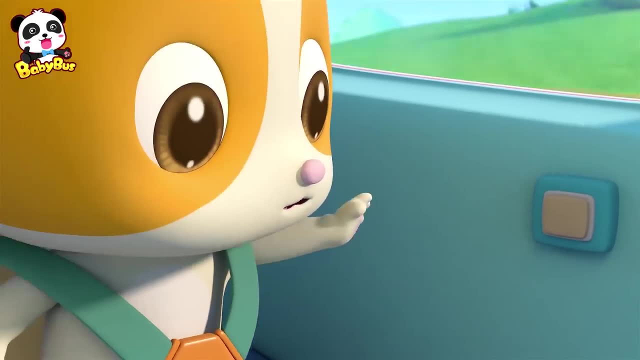 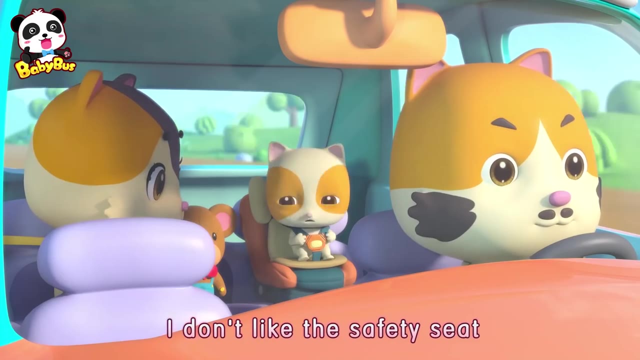 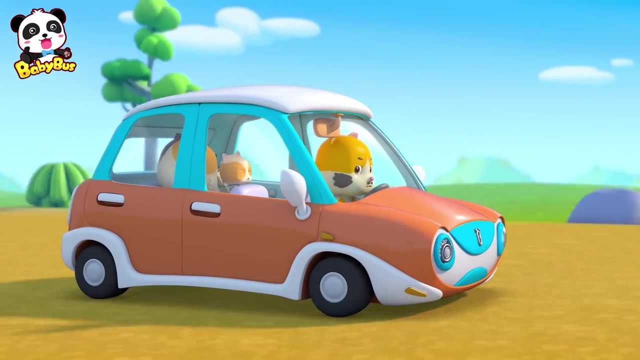 Don't worry, your seat will keep you safe. Mommy, please help me, please, Please, unbuckle my seatbelt. I don't like the safety seat. I want to get out of it. We can go on out today, Sweetie, sweetie, sit up straight. 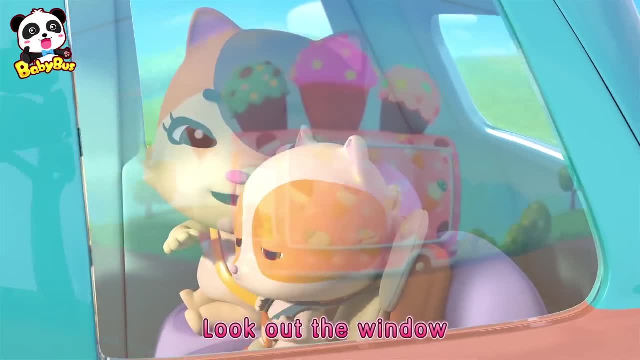 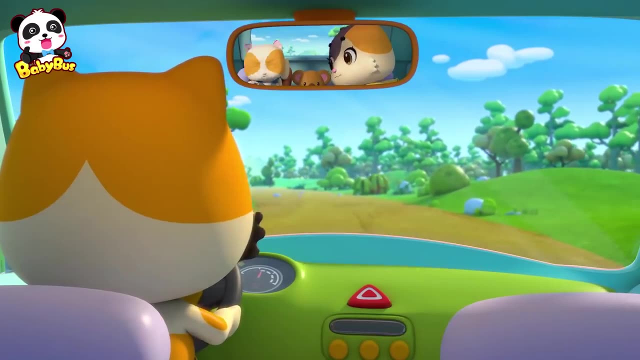 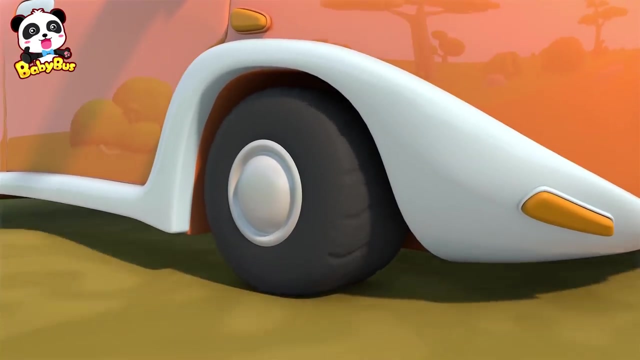 Please keep sitting in your seat. Look out the window, tell me what it is. Wow, it's an ice cream truck. There is lots of ice cream there. Bumpy Road coming hold on tight, Don't worry, Your seat will keep you safe. 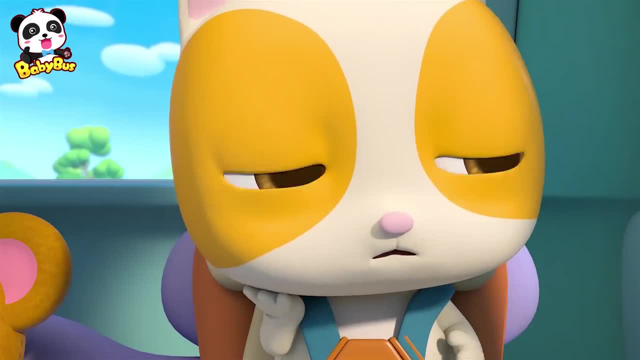 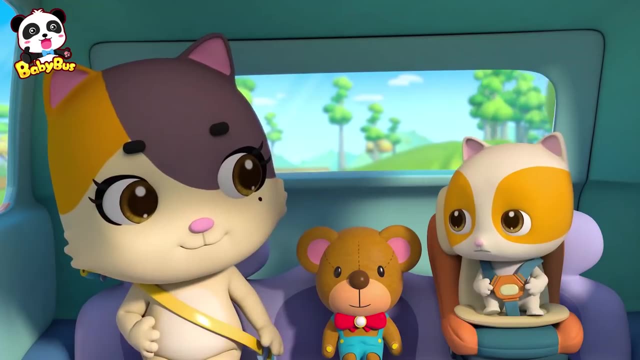 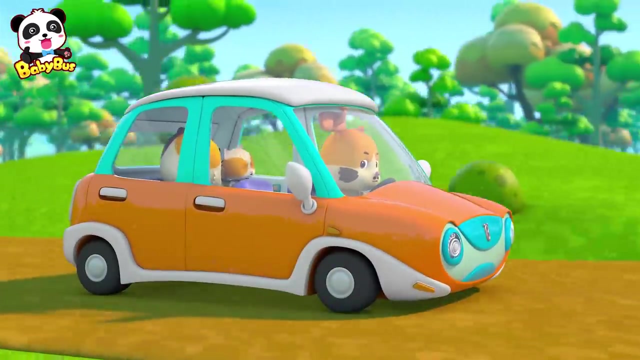 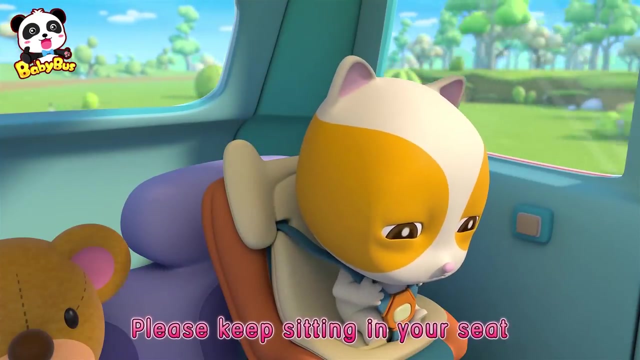 Mommy, please help me, please, Please, unbuckle my seatbelt. I don't like the city seat. I want to get out of it. Sweetie, sweetie, sit up straight. Please keep sitting in your seat. How about playing a game with me? 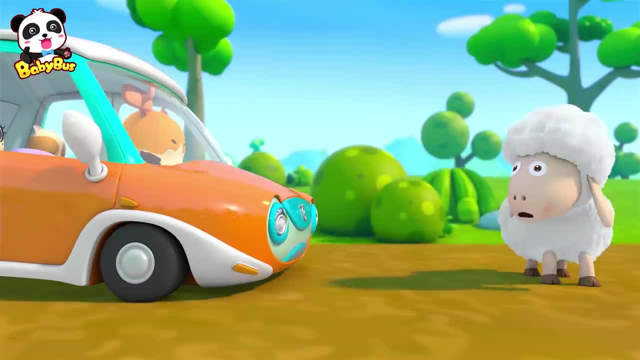 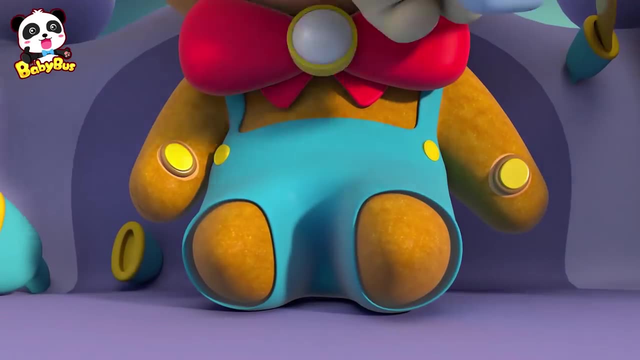 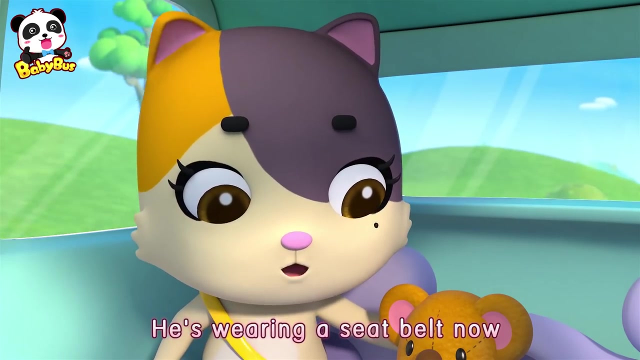 What kind of game Go watch out. My teddy Teddy fell down because he did not sit in his safety seat. He's wearing a seatbelt now, so he will be safe. I'm sitting in my safety seat, so I'll be safe too. 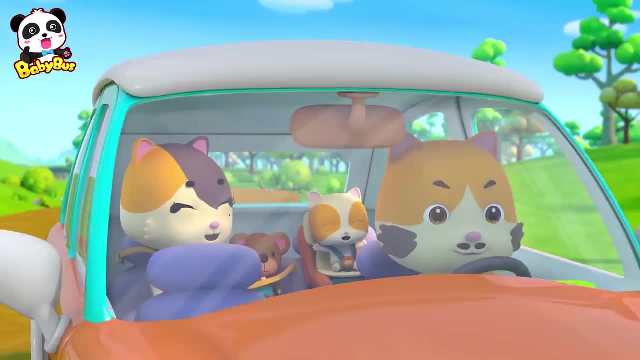 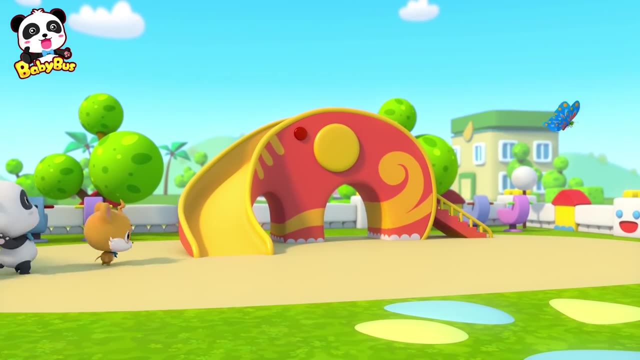 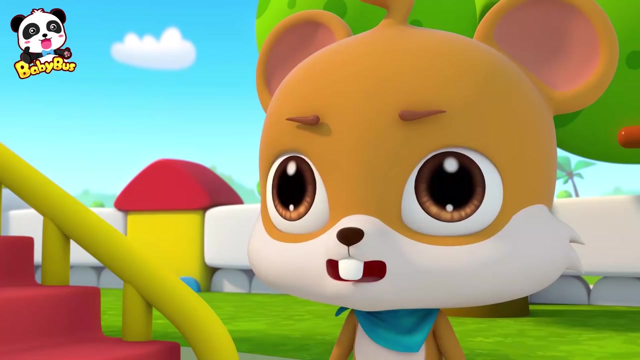 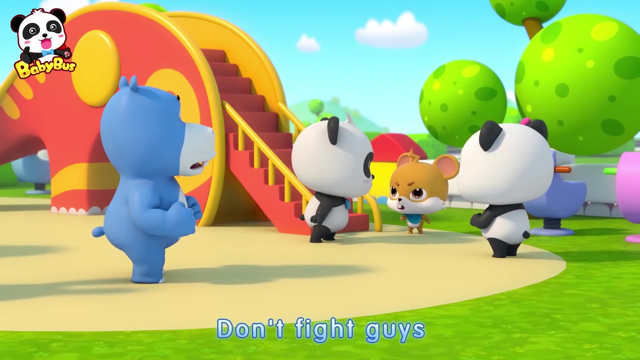 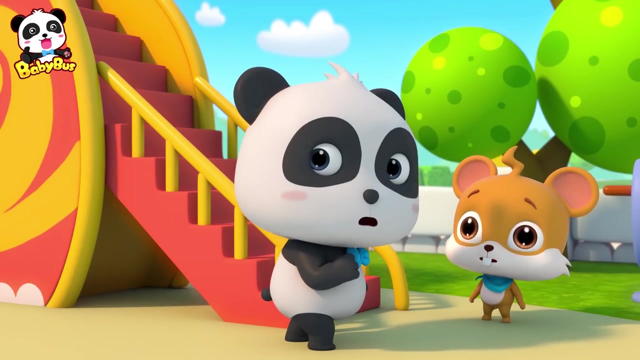 Yeah, I love my safety seat. I came first. No, I came first. Don't fight guys, I'm first. No, I'm first. Oh, what's the matter? Miss Mimi, I want to ride the slide first. 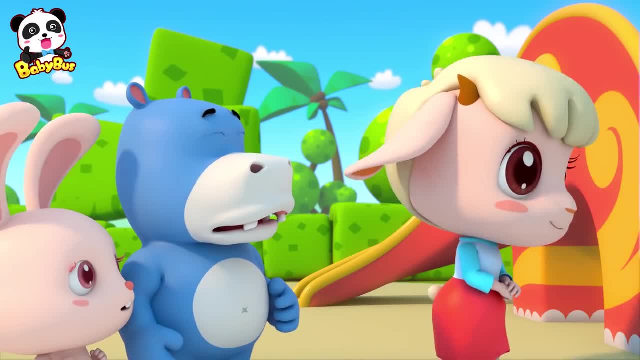 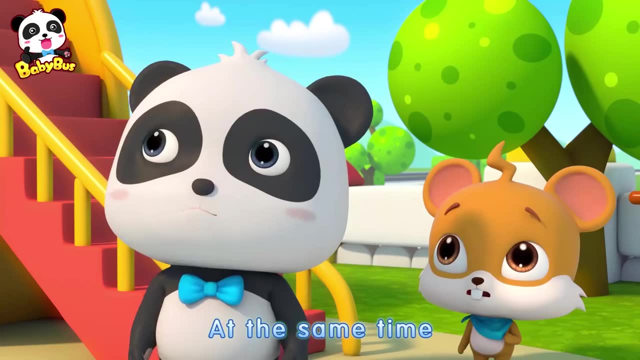 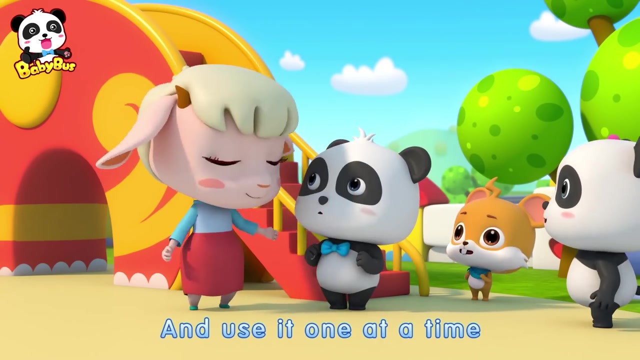 I want to ride the slide first too. Kiki Whiskers, we have only one slide here. When both of you want it at the same time, what should we do? You should line up and use it one at a time, So everyone will have a good time. 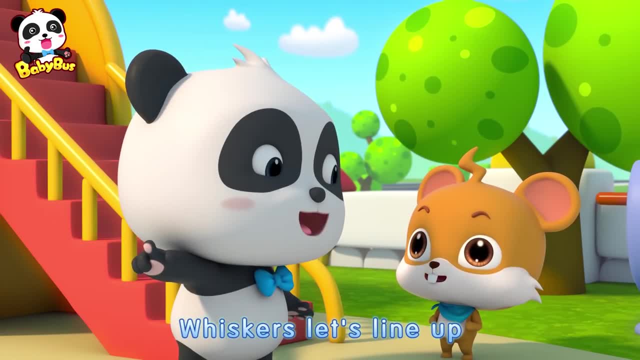 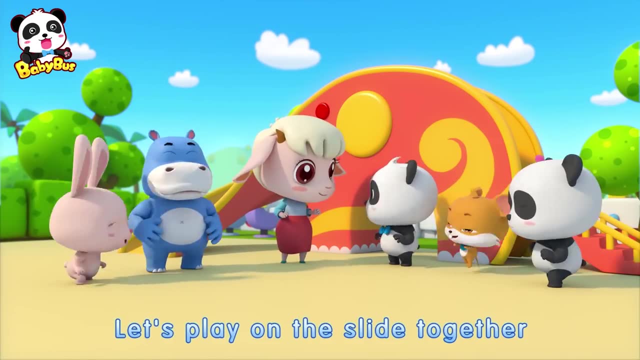 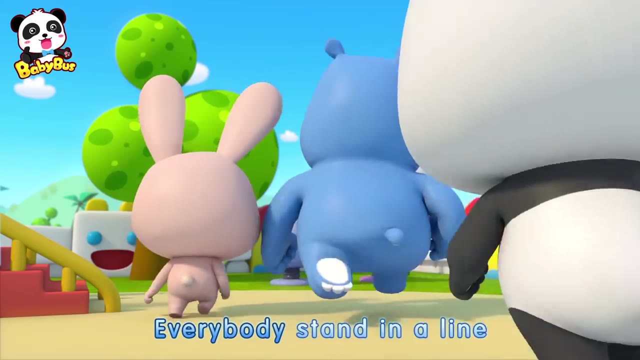 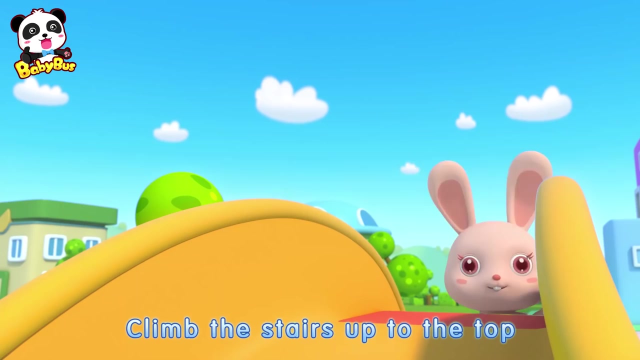 Whiskers. let's line up. Okay, Let's play on the slide together. Yeah, A long, long slide like an elephant's trunk. Everybody stand in a line. Hold the handrail tight. One step at a time, Climb the stairs up to the top. 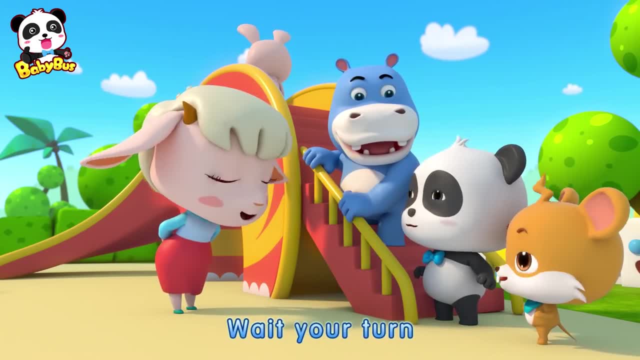 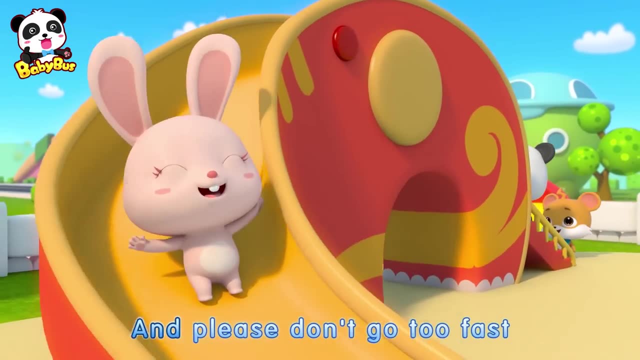 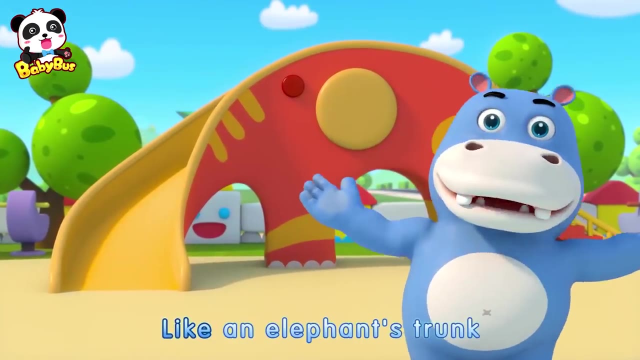 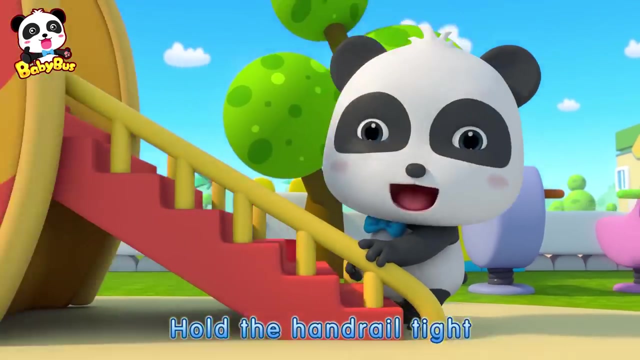 Hold on, wait your turn. Please go down the slide one at a time. Sit up straight, please, And please don't go too fast. It's so fun to ride the slide, A long, long slide like an elephant's trunk. Everybody stand in a line. Hold the handrail tight. 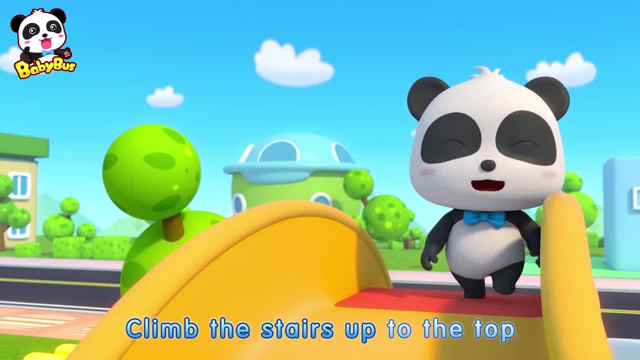 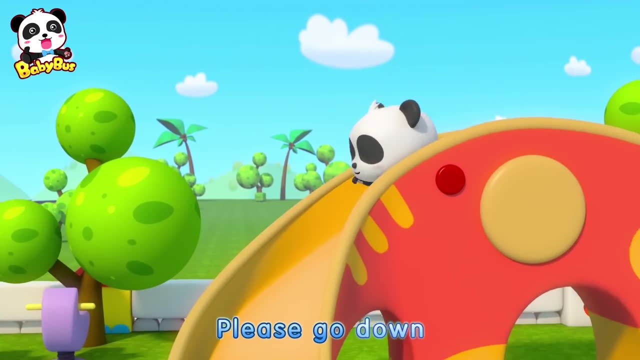 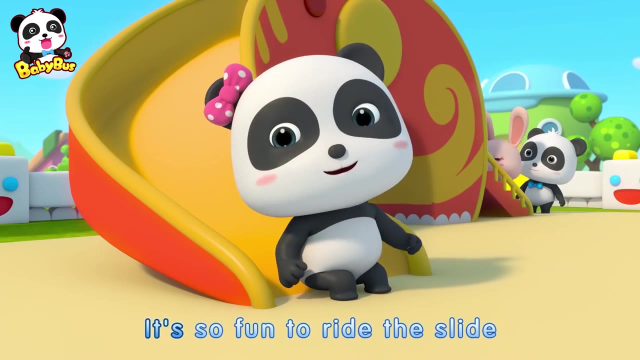 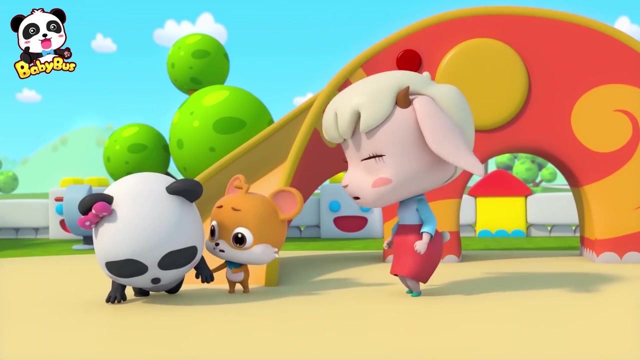 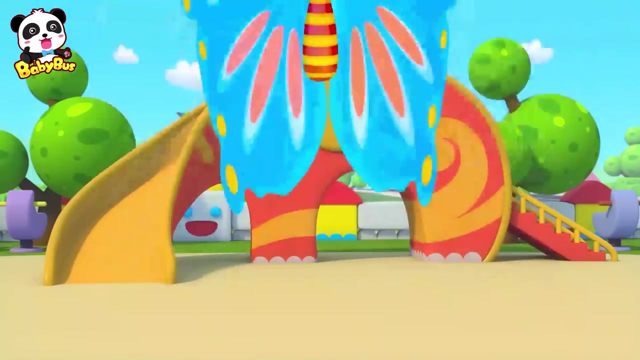 One step at a time. Climb the stairs up to the top. Hold on, wait your turn, Please. go down the slide one at a time. Sit up straight, please, And please don't go too fast. It's so fun to ride the slide- A long, long slide- like an elephant's trunk. 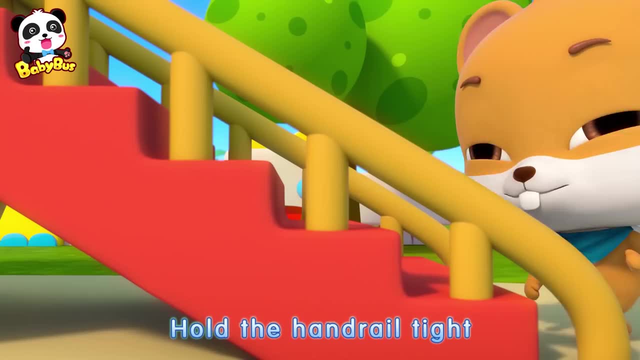 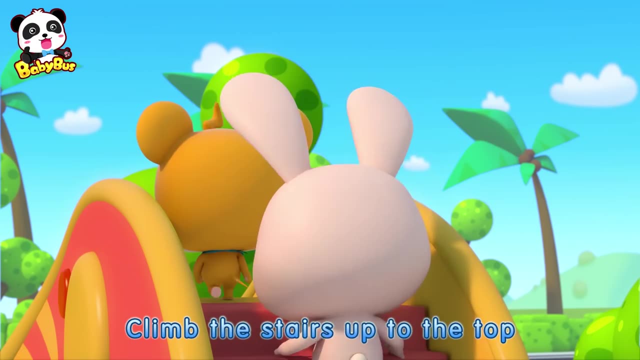 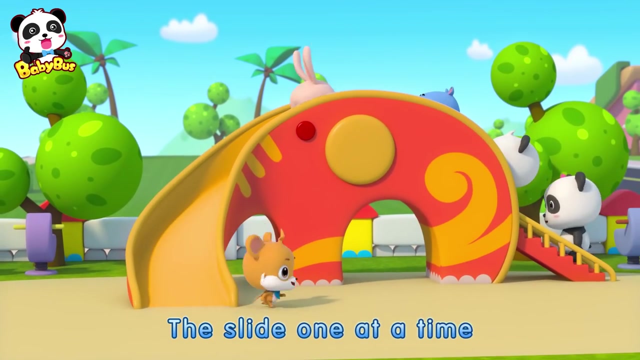 Everybody stand in a line. Hold the handrail tight, One step at a time. Climb the stairs up to the top. Please go down the slide one at a time. Hold on, wait your turn. Please go down the slide one at a time. Sit up straight, please. 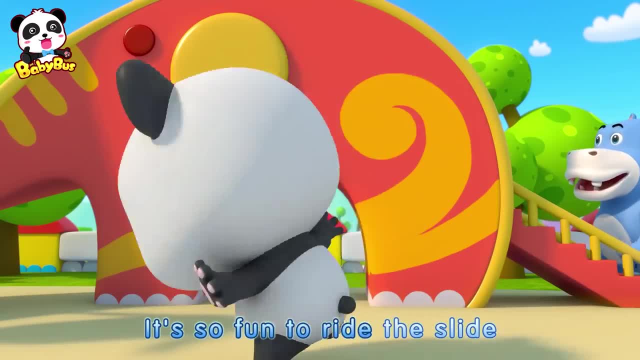 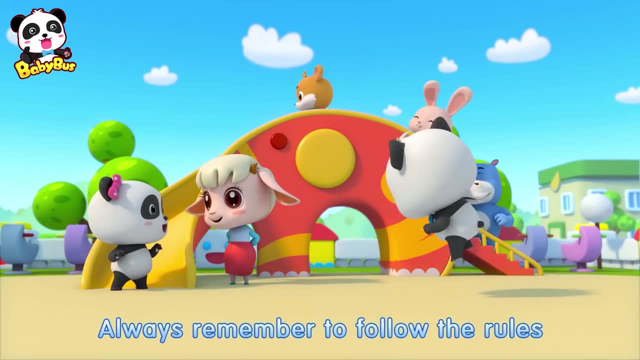 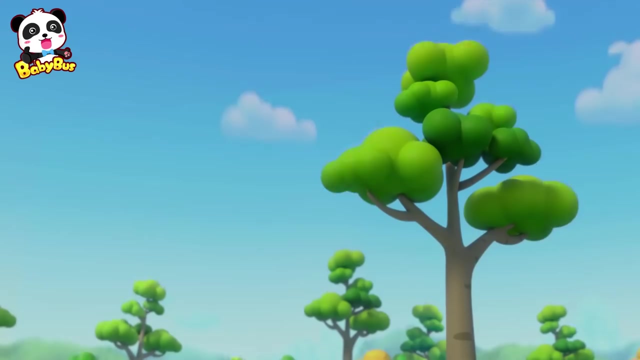 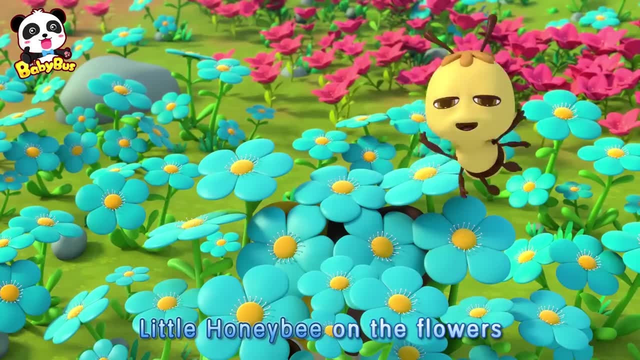 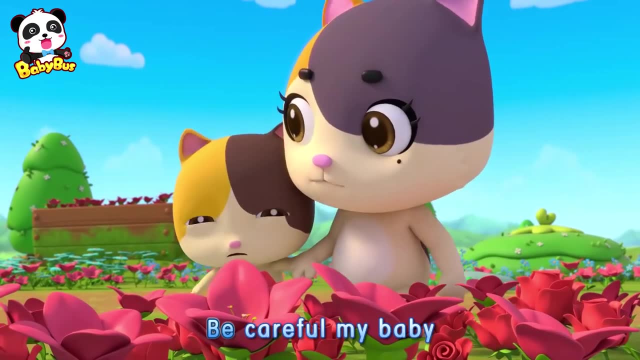 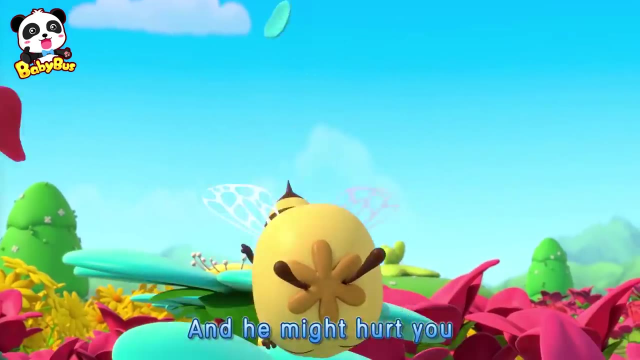 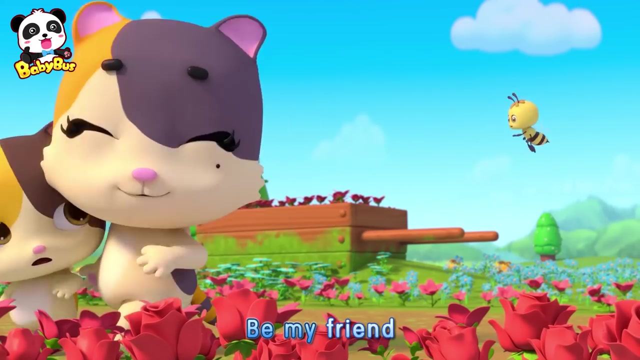 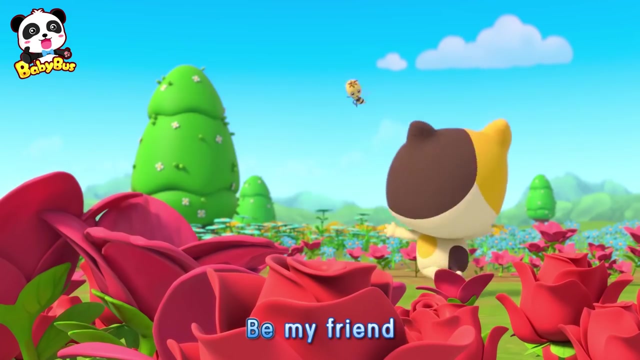 When you play with your friends, always remember to follow the rules so everyone can have a good time. When you play with your friends, always remember to follow the rules so everyone can have a good time. Be my friend. Little honeybee on the flowers. 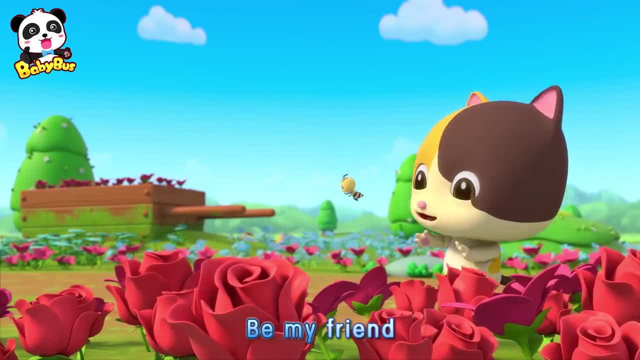 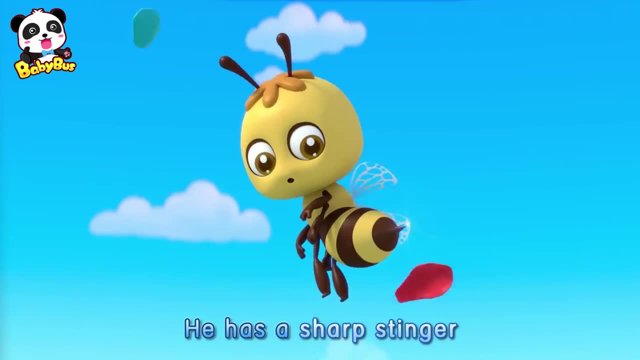 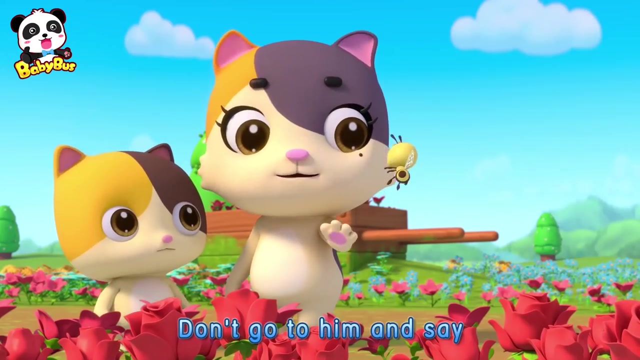 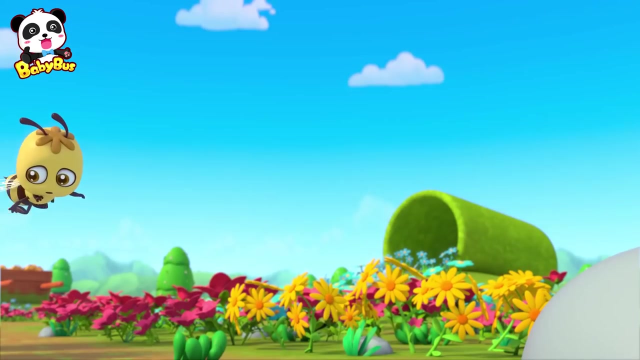 I go to him and say: Be my friend, Be careful my baby, Don't follow the honeybee. He has a sharp stinger And he might hurt you. Oh, little honeybee on the flowers. Don't go to him and say: Be my friend, Little honeybee, Don't fly away. 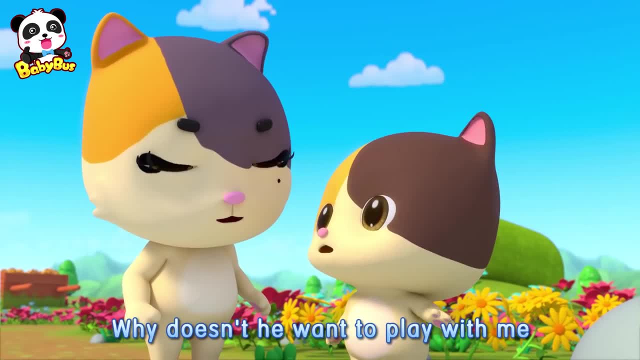 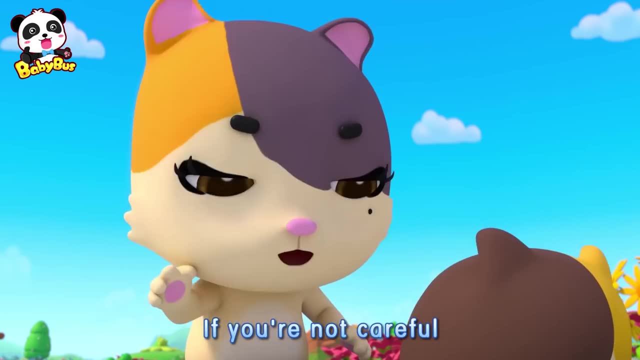 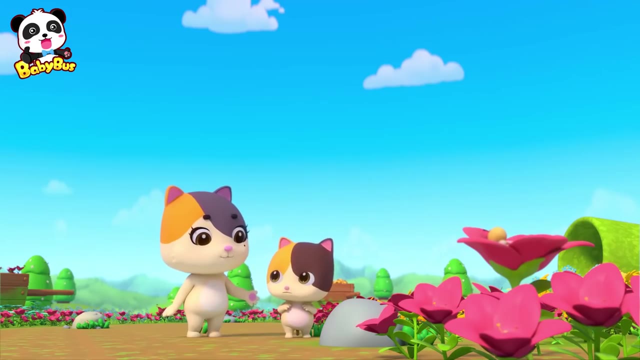 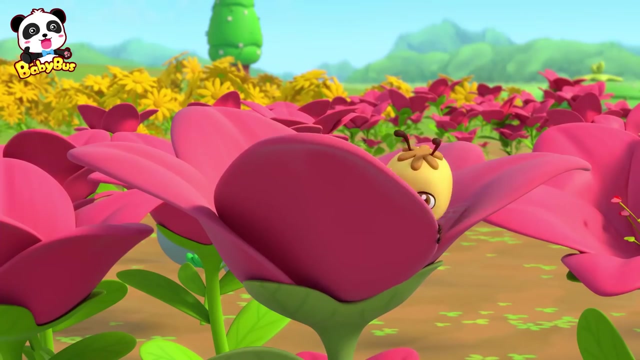 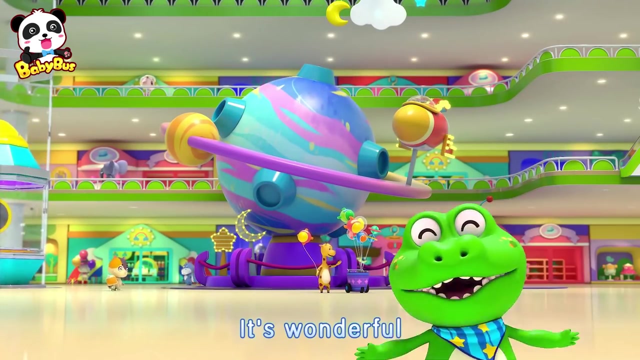 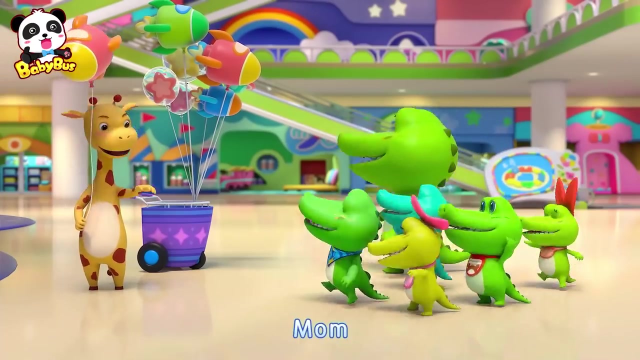 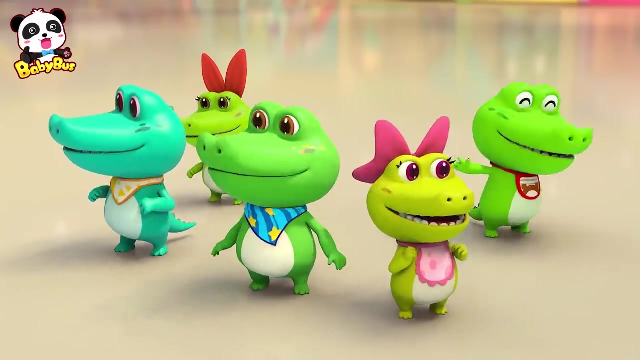 Why doesn't he want to play with me? Because he doesn't want to hurt you. If you're not careful, He can sting you. Let's go somewhere else. Alright, Bye, little honeybee. Bye. Wow, it's wonderful. Wow, mom, We want rocket balloons. Okay, I like this place. 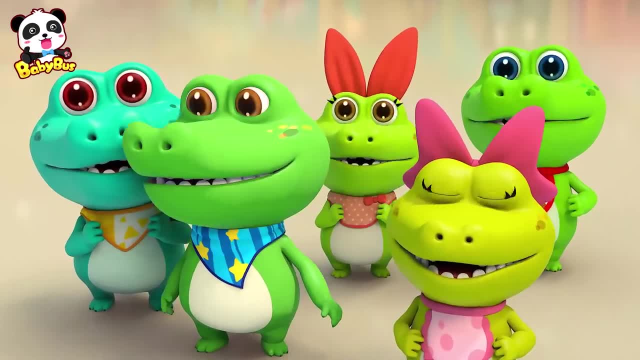 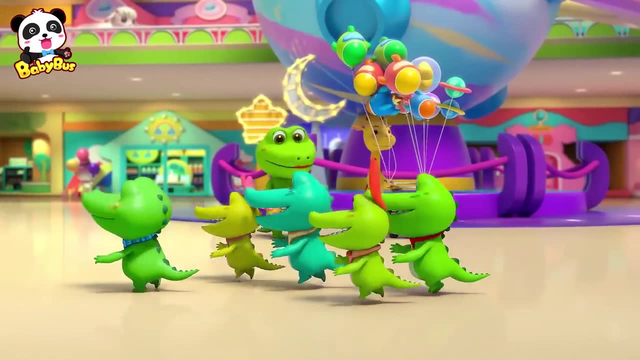 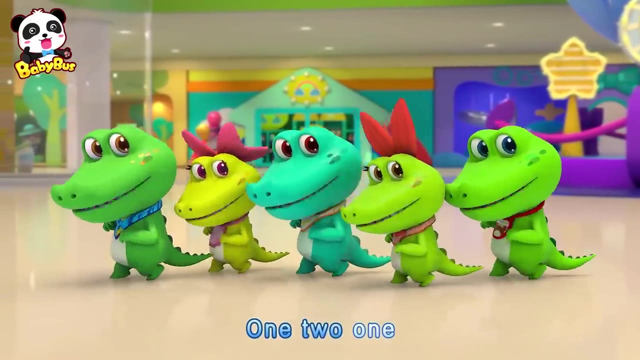 Look over there. Wow, There is a rocket balloon. There is a rocket balloon. There is a rocket balloon. There is a bigger rocket over there. Let's get on it, Don't run around. One, two, one, One, two, one. Five little crocodiles, Five little crocodiles. 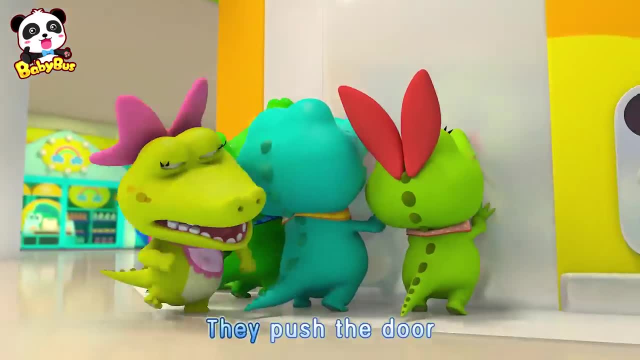 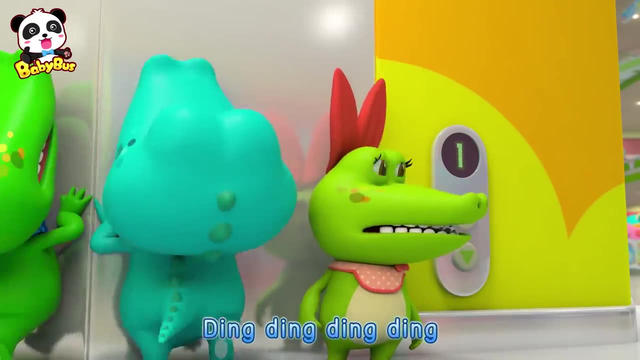 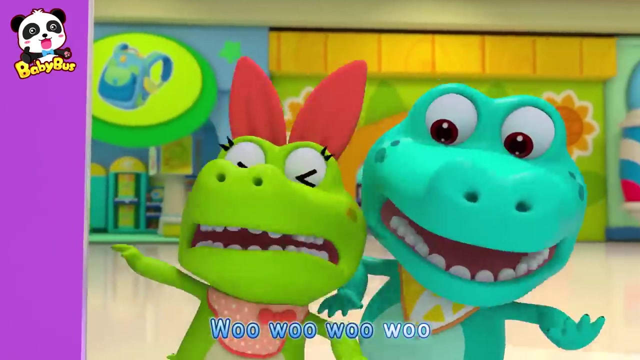 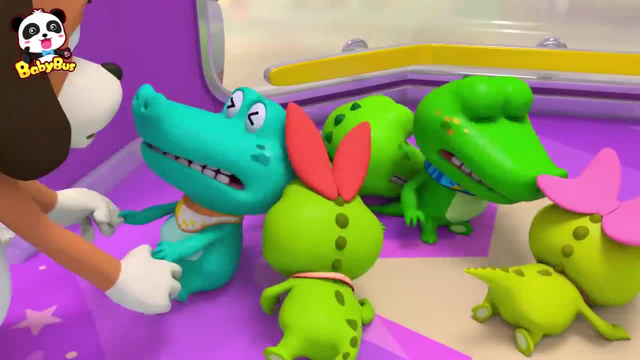 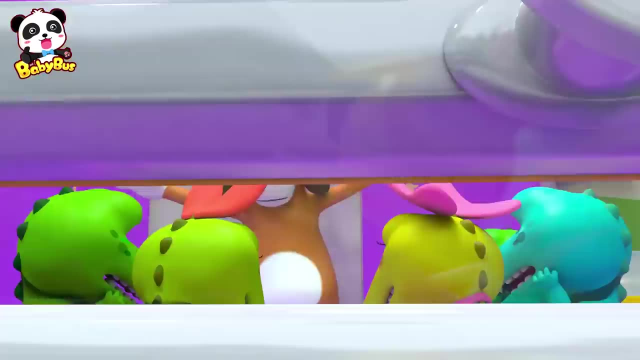 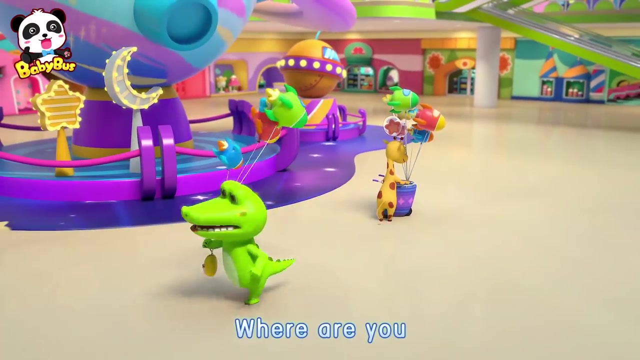 Ooh, ooh, ooh, ooh, We fell down. Ooh, ooh, ooh, ooh, Ouch, ouch, ouch. Don't lean on the elevator door. It's dangerous, You could get hurt. Where are my babies, Kids, where are you? It's mommy. 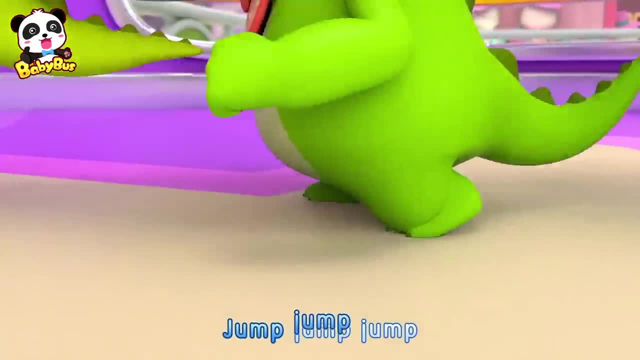 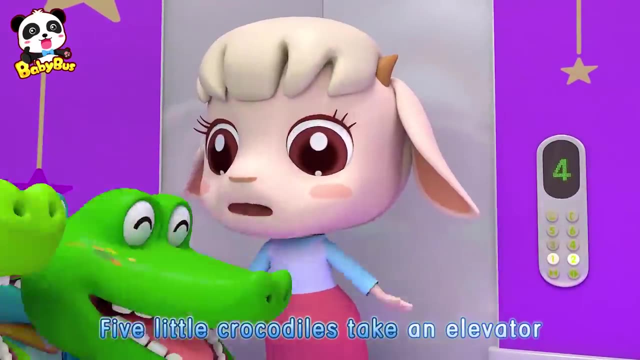 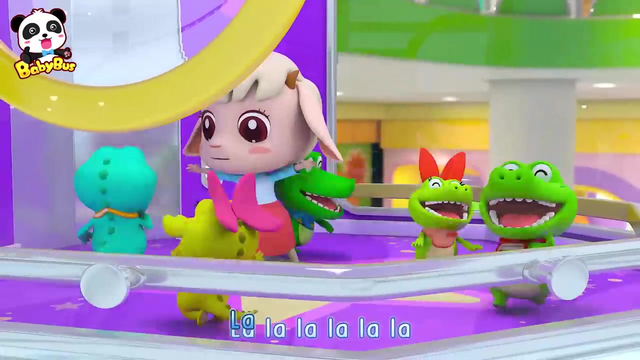 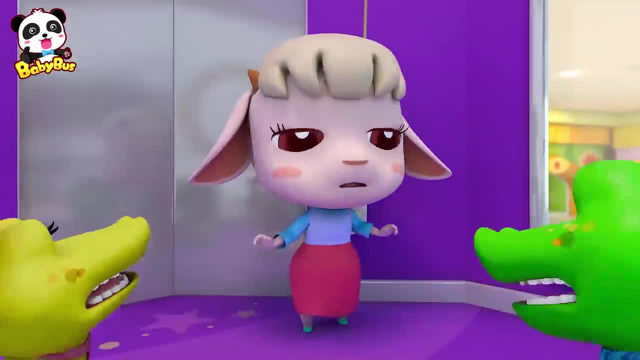 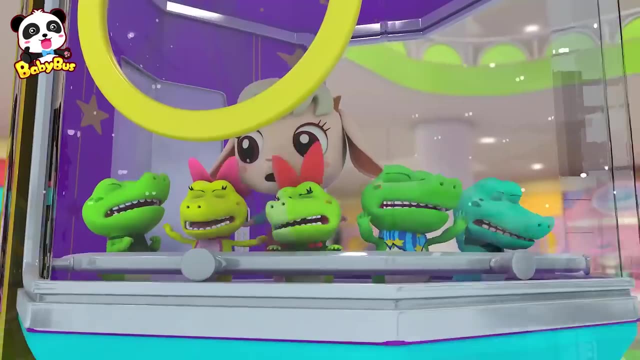 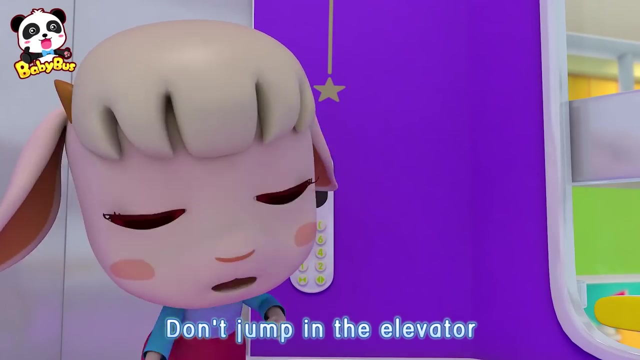 Ooh, ooh, ooh, ooh, What is wrong? Ooh, ooh, ooh, ooh, We are scared. Ooh, ooh, ooh, ooh, Oh, what is wrong? Oh, oh, oh, oh, we are scared. No, no, Don't jump in the elevator. 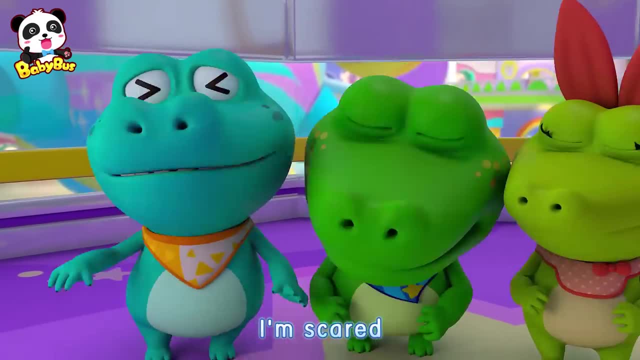 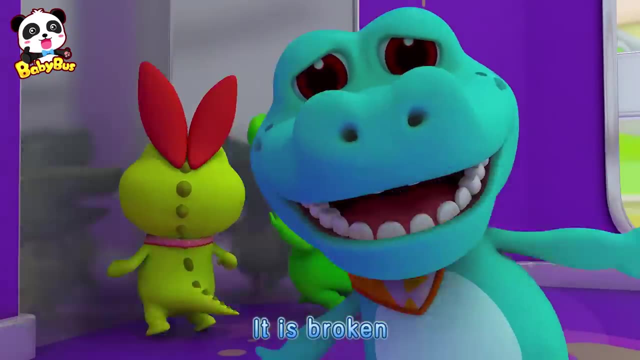 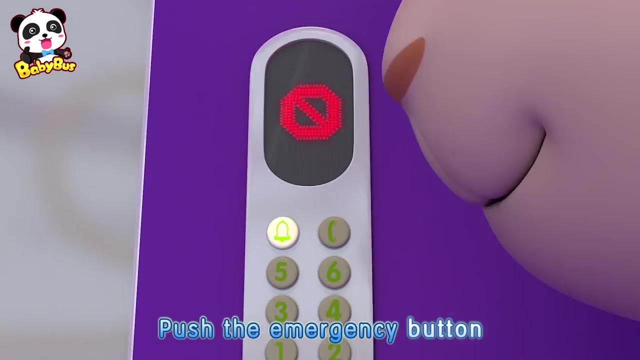 And don't push too many buttons either. I'm scared. I want my mommy. Five little crocodiles take an elevator. It is broken. what should we do? Don't be afraid. please stay calm. Push the emergency button and wait for help. 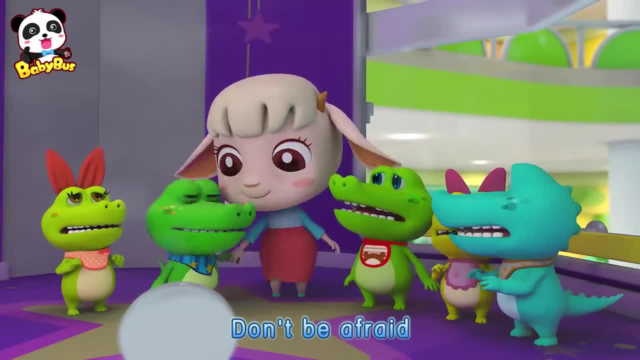 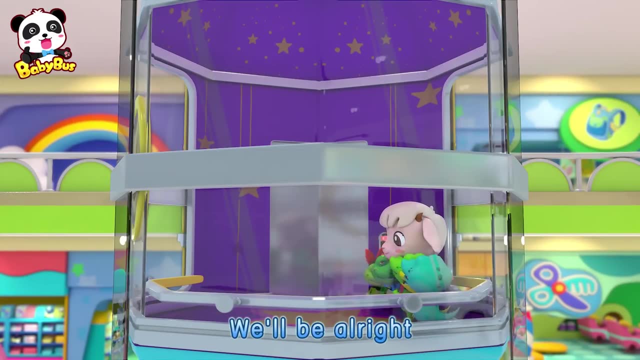 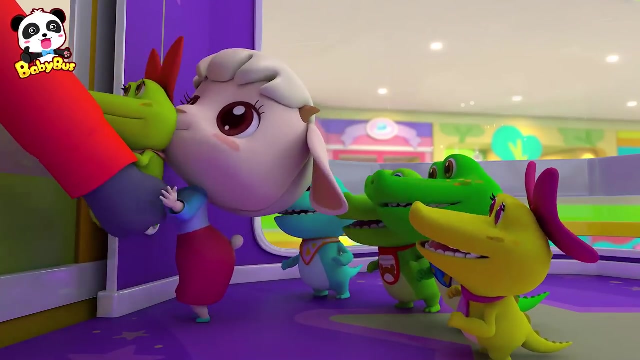 La la la la, don't be afraid. La la la la, please stay calm. La la la la, we'll be alright. La la la la, help arrive My babies. Mom, Mom. 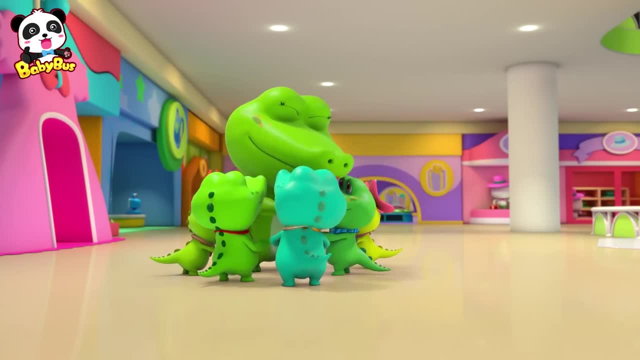 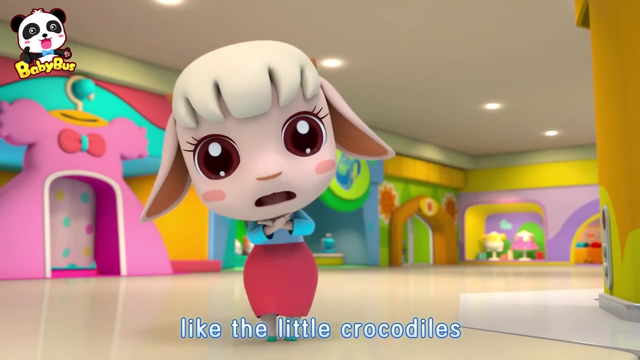 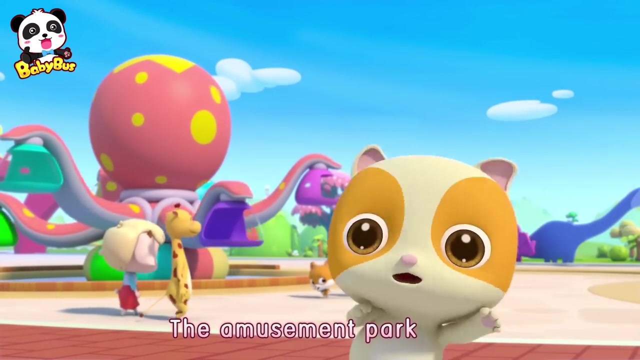 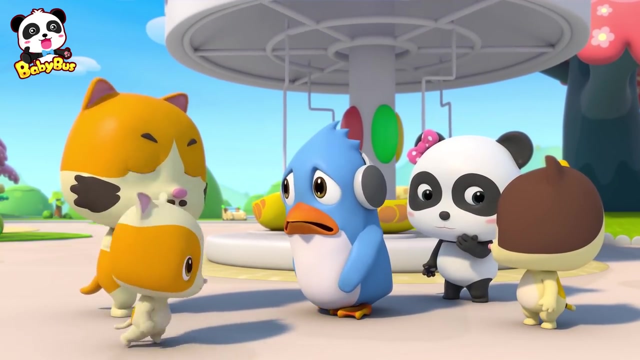 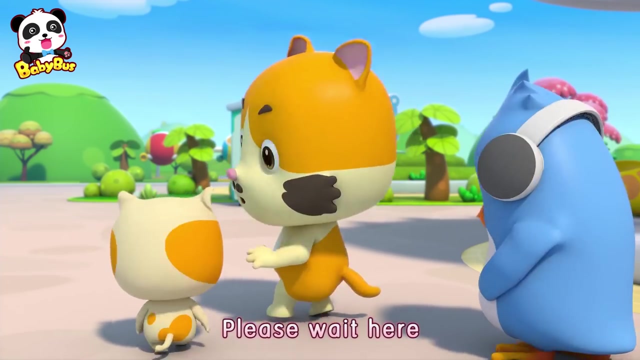 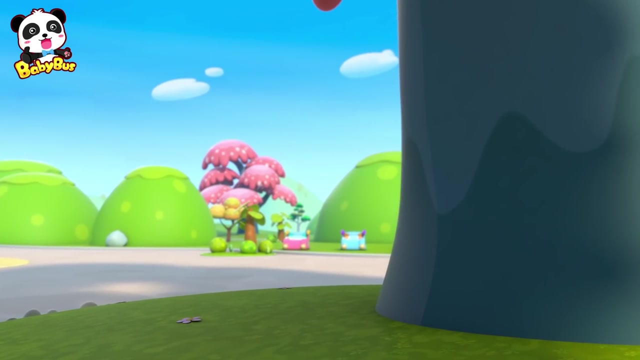 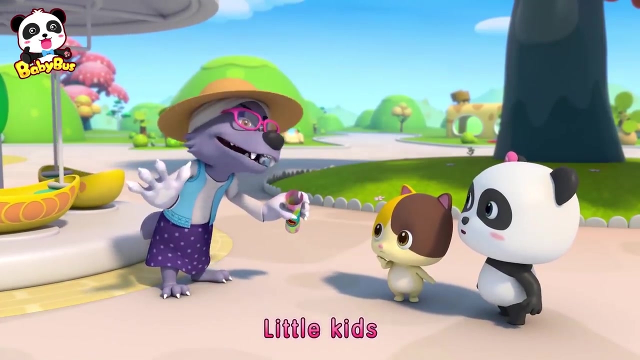 You need to stay close to me. That was really dangerous. Kids do not play in the elevator like the little crocodiles. Hello, hello little kids. I'm looking for a candy shop. Hello, hello little kids. will you go with me? 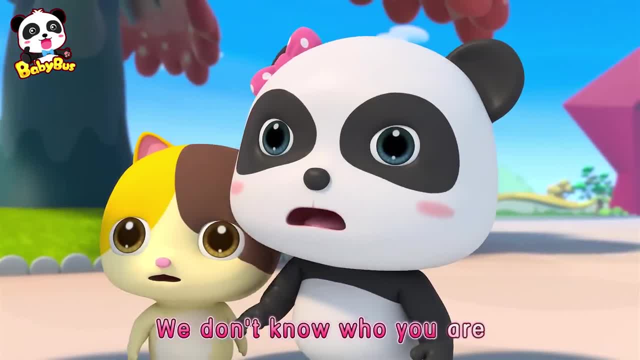 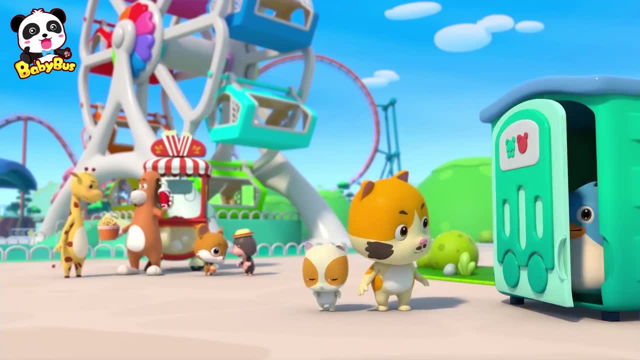 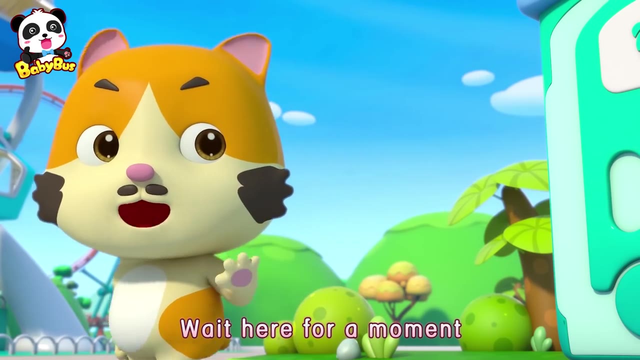 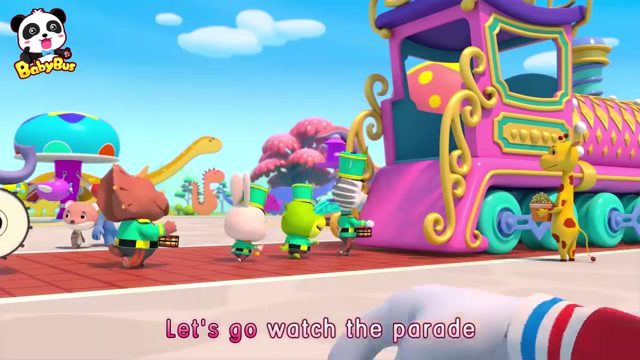 No, no, no way, We don't know who you are. No, no, no way, We won't go with you. No way, Dad, I want some popcorn. Okay, Rudolph, wait here for a moment. Okay, Hello, hello little kid, let's go watch the parade. 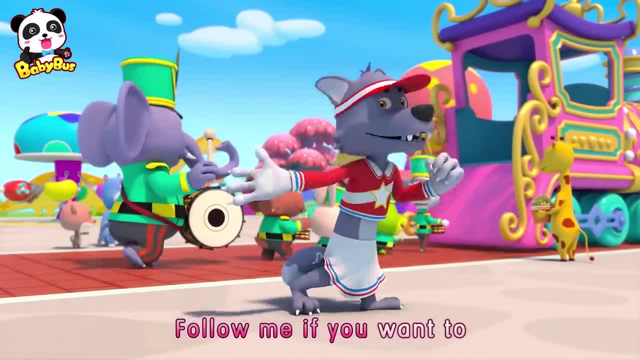 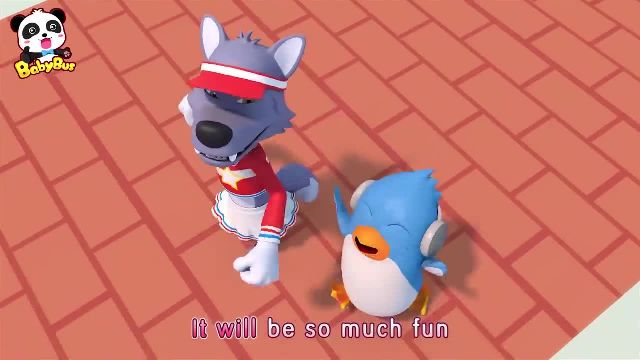 Hello, hello little kid, follow me. if you want to, Okay, okay, let's go. I want to see the parade- Okay, okay, let's go. it will be so much fun. Follow me. Rudolph's going with a stranger. 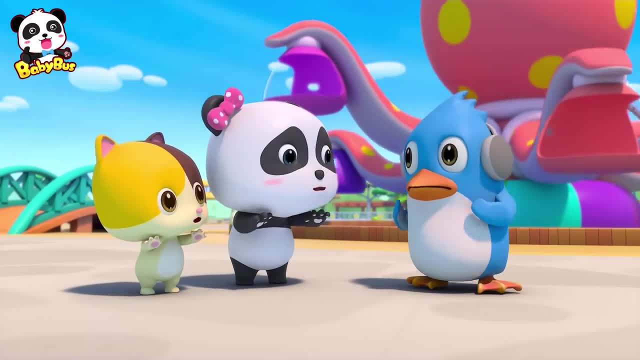 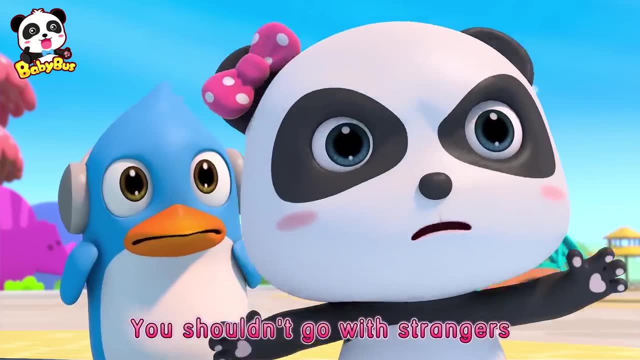 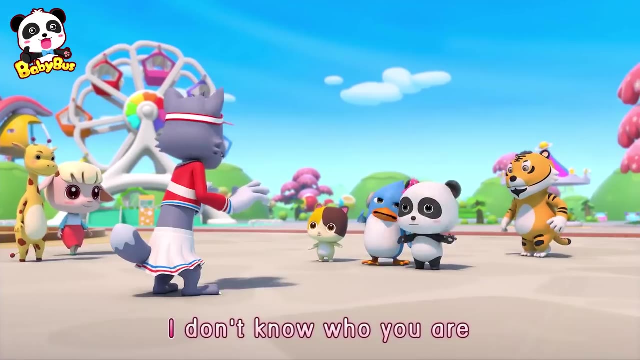 No, no, you should not. you shouldn't go with strangers. No, no, you should not. you shouldn't go with strangers. Hey, hey, stranger, I don't know who you are. Hey, hey, stranger, I don't know who you are. 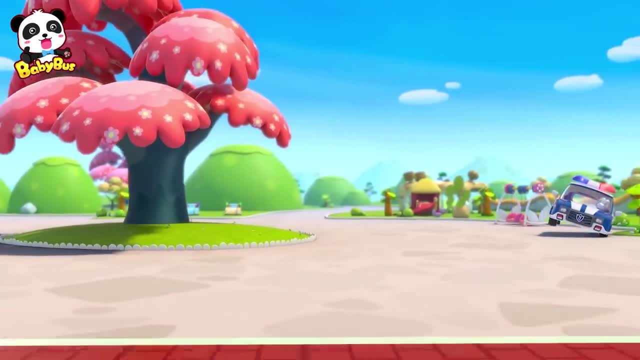 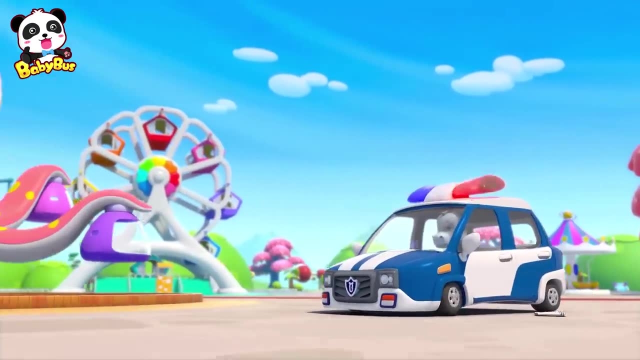 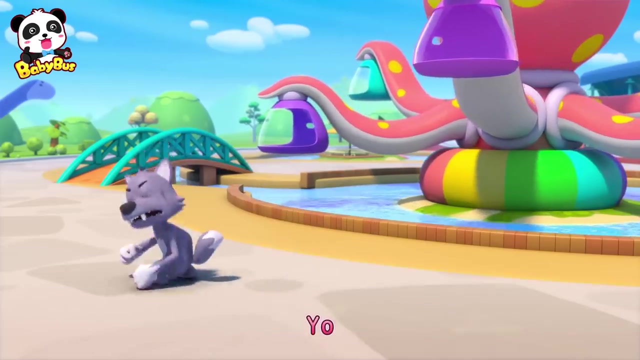 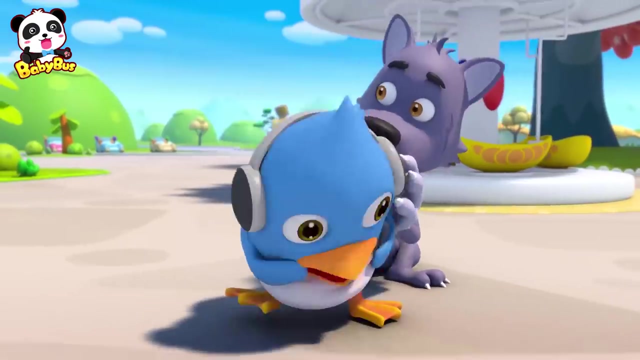 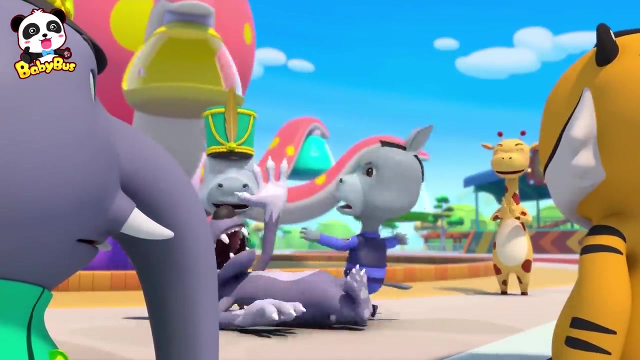 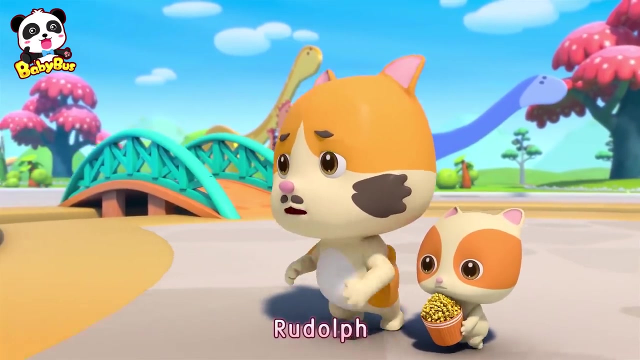 Go away. Hey hey, stop there, Yo, yo, I got you. Hey, hey, stop there, Yo, yo, I got you. It's so dangerous, Tell the stranger. It's so dangerous. Tell the stranger, No, no, Mimi, Miu, Miu Rudolph. 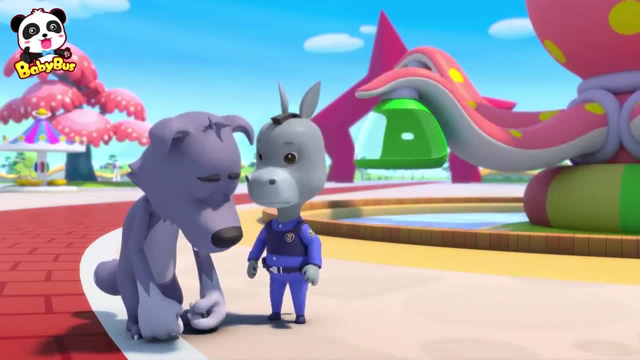 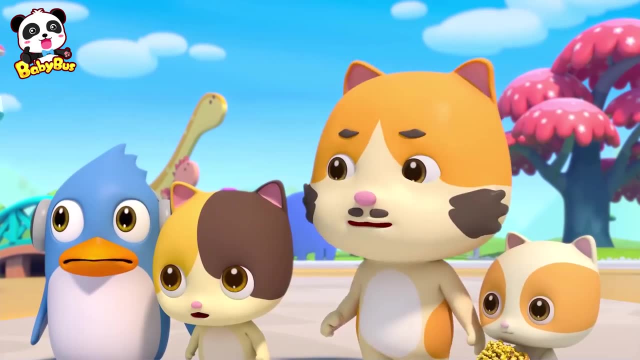 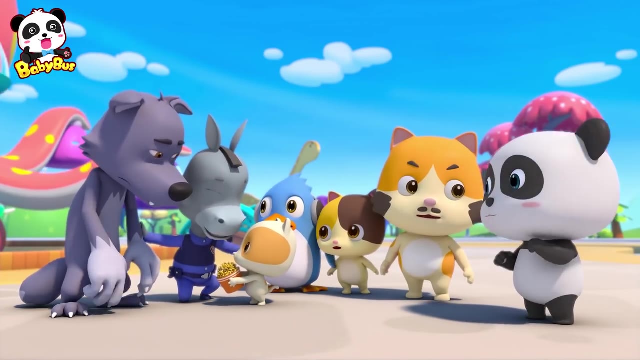 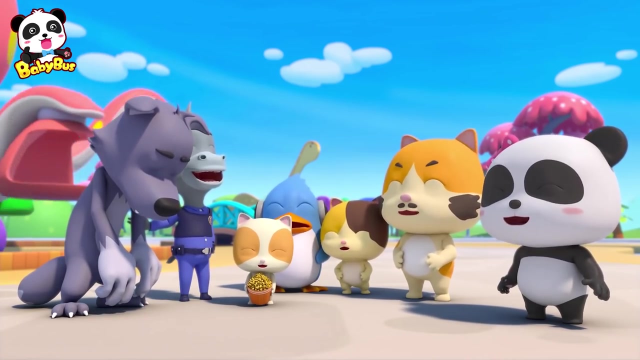 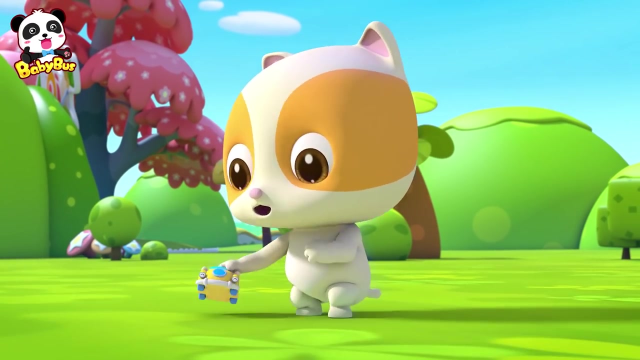 Dad, Are you okay? Yes, You should never leave the children alone. I'm sorry, it was all my fault. Eat, have some popcorn. I shouldn't take food from a stranger Like what I'm doing now, Playing with my car. zoom, zoom, zoom. 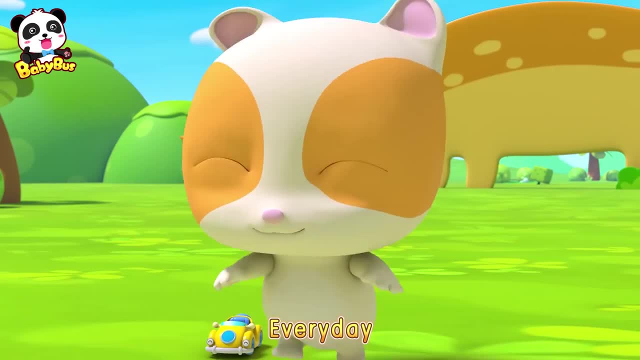 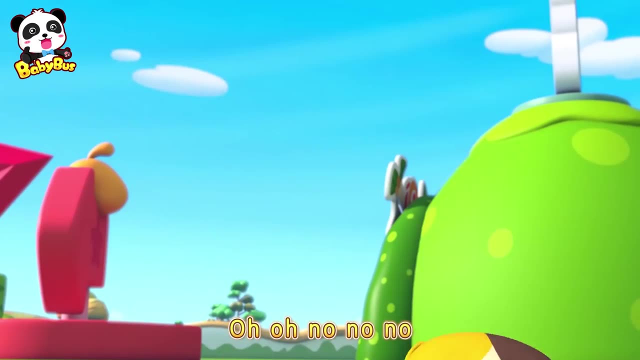 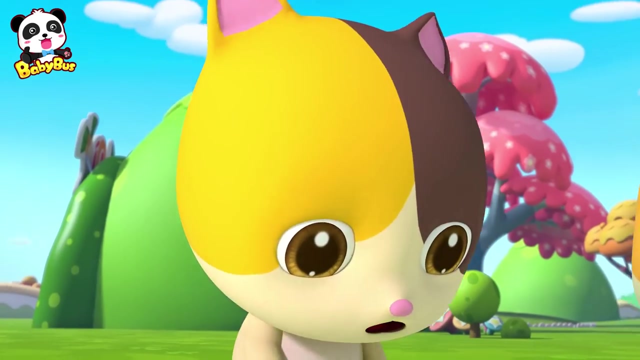 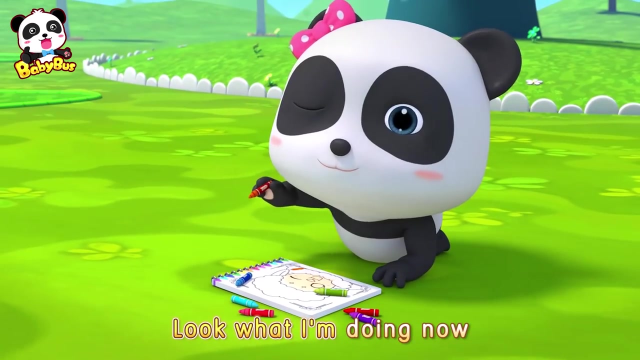 I have fun every day, every day, Oh, oh, no, no, no, Oh, oh, I fell down. Do you know? do you know Who I am? Do you know who did this? I'm sorry, Look what I'm doing now. 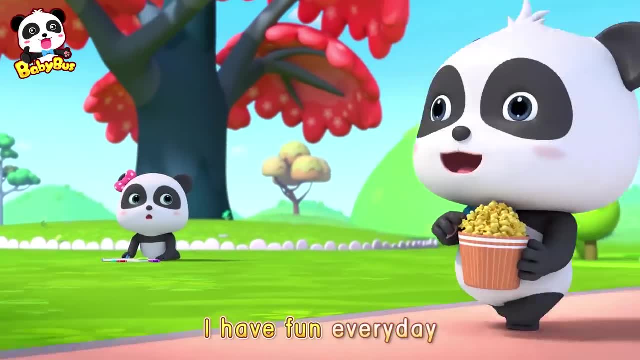 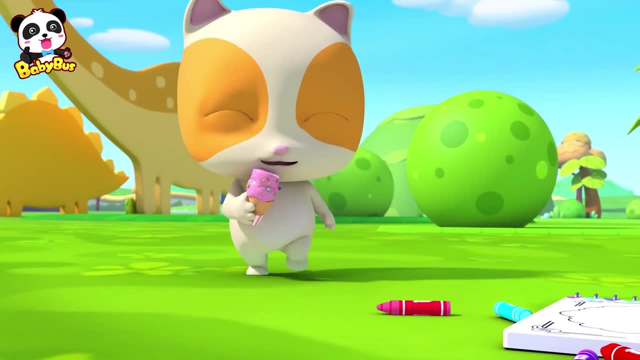 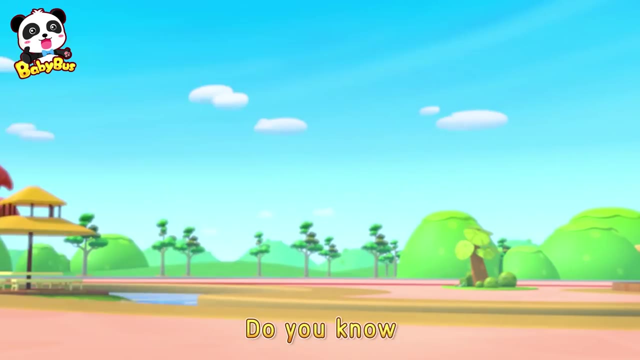 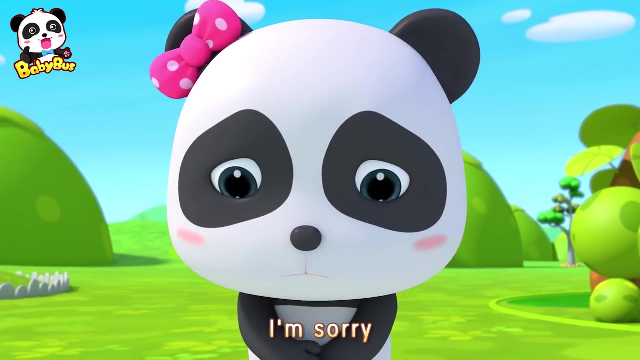 Drawing a picture. ha ha ha. I have fun every day, every day, Oh, oh, no, no, no, Oh, oh, I fell down. Do you know? do you know Who did this? I'm sorry, Look what I'm doing now. 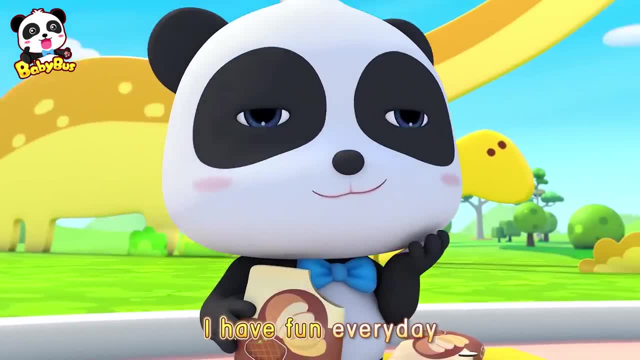 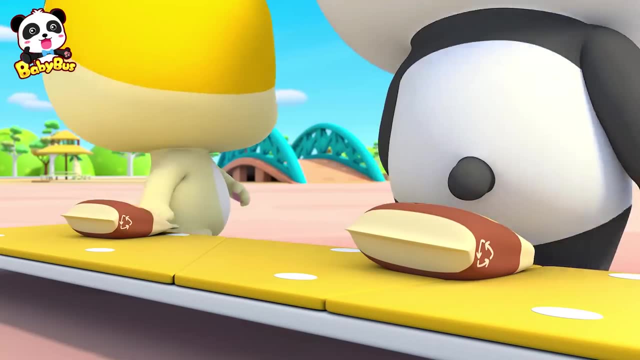 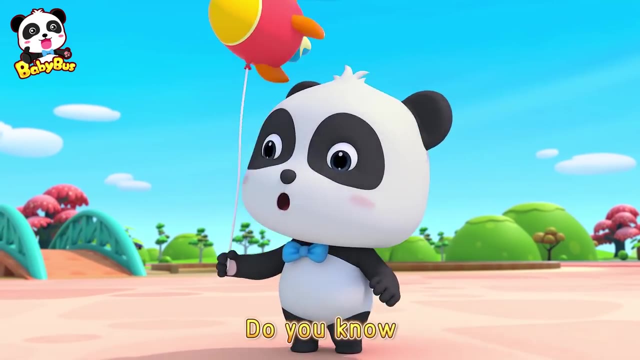 Having some chips, crunch, crunch, crunch. I have fun every day, every day. Oh, oh, no, no, no, Oh, oh, we're surprised. Do you know? do you know Who did this? Oh, oh, no, no, no. 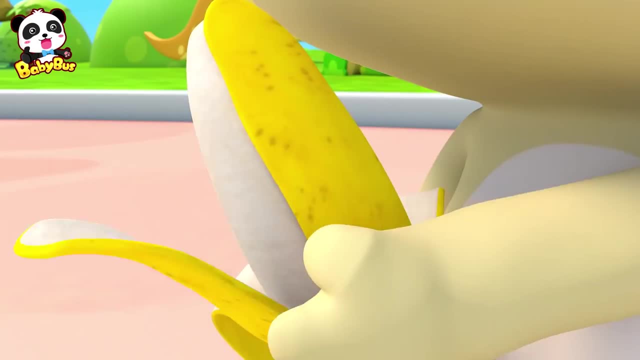 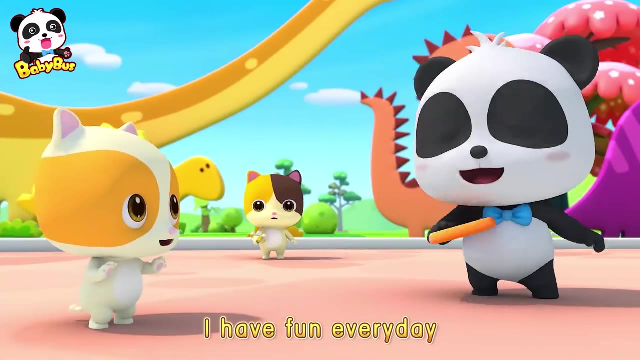 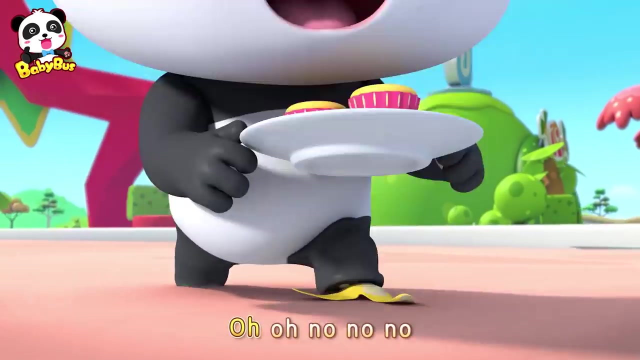 Oh, oh, I'm sorry. Look what I'm doing now, Having a banana. yum, yum, yum yum. I have fun every day, every day, Oh, oh, no, no, no, Oh, oh, I fell down. Do you know, do you know? 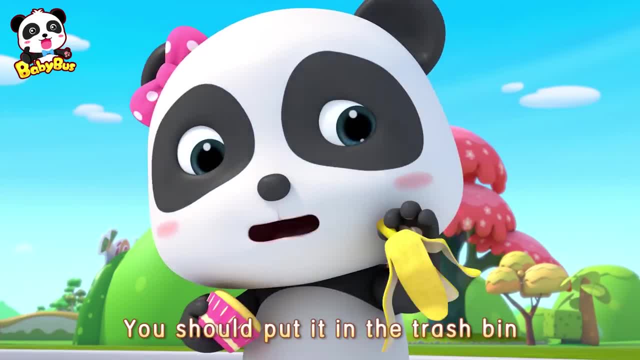 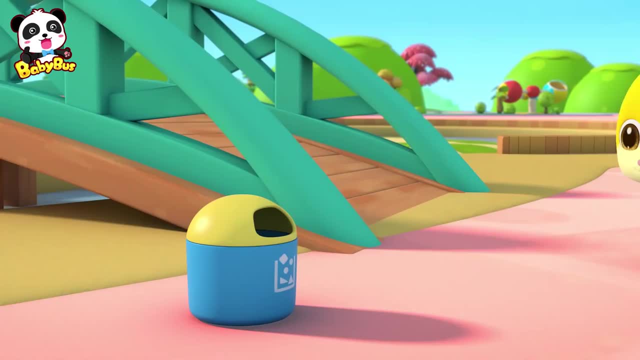 Who did this? I'm sorry, You should put it in the trash bin. Take a bath for me. 뭐라 reag한 것인지? Ah Okay, 자기는 좀 알려드릴게요, aí Notre Dome, Okay. 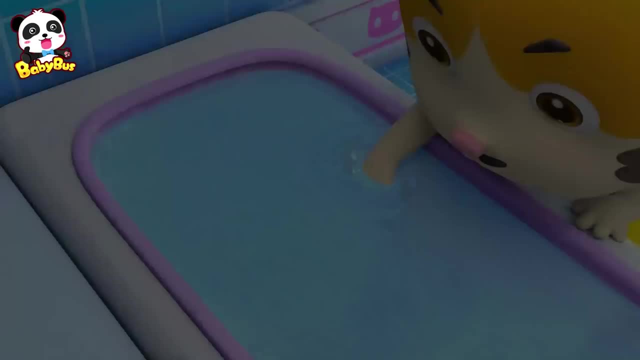 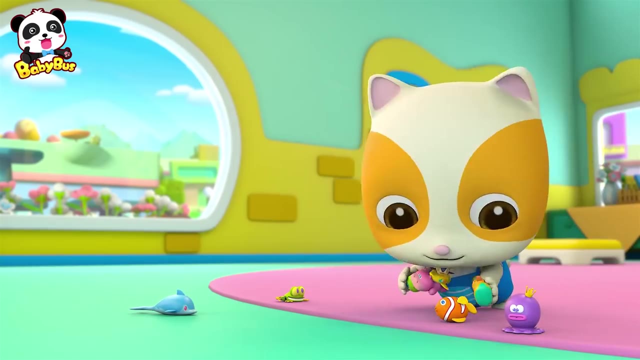 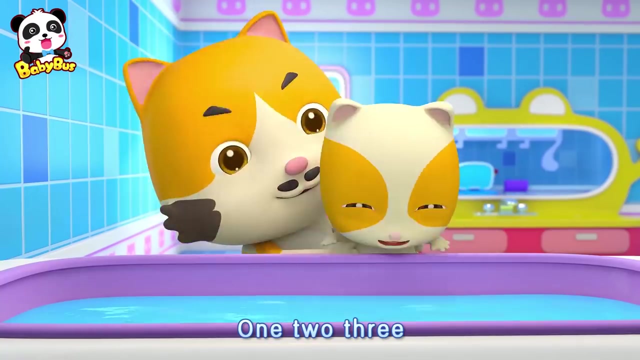 Oka, Let's play over there. Okay, Bahtim Timmy. Okay, Take a bath, Let's take a bath. I'm ready. I'm ready. One, Two, Three. Can you wash your hair? Scrub-a-dub-dub, I can wash my hair. 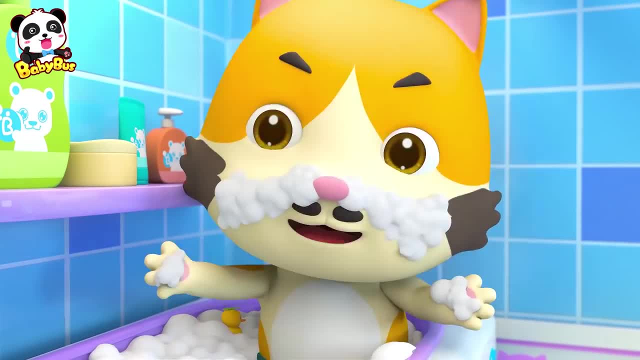 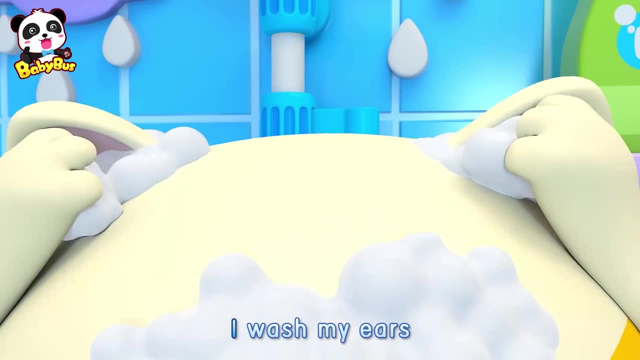 Scrub-a-dub-dub. Can you wash your face? Scrub-a-dub-dub, I can wash my face. Scrub-a-dub-dub: Wash your ears, wash wash. I wash my ears, wash wash. Close your eyes. I'll miss you. 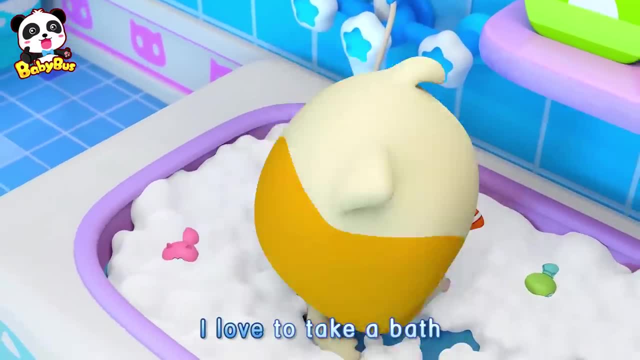 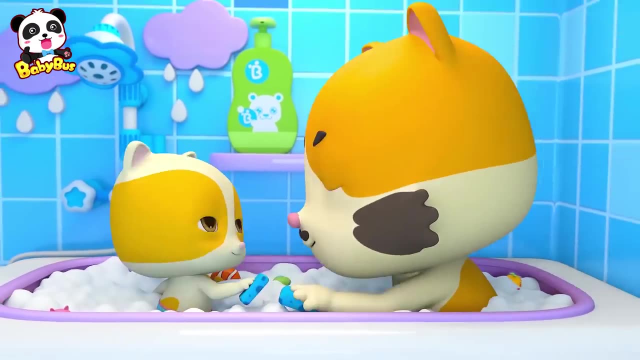 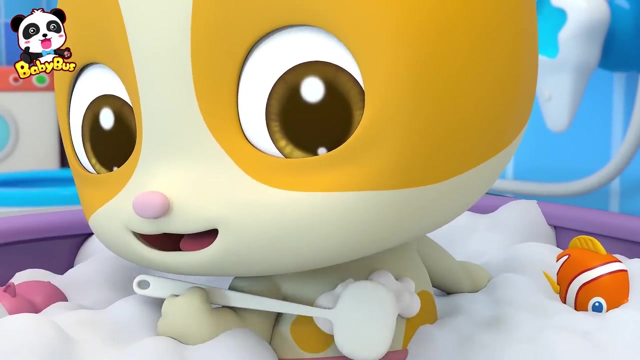 Splash, splash pop. I want to take a bath. Take a bath. Can you wash your back? Scrub-a-dub-dub. I can wash my back. Scrub-a-dub-dub. Can you wash your tummy? I can wash my tummy. 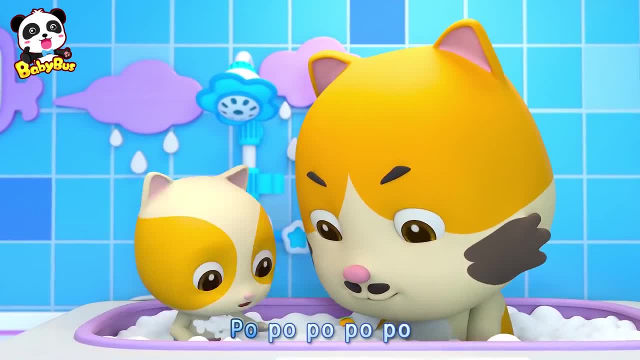 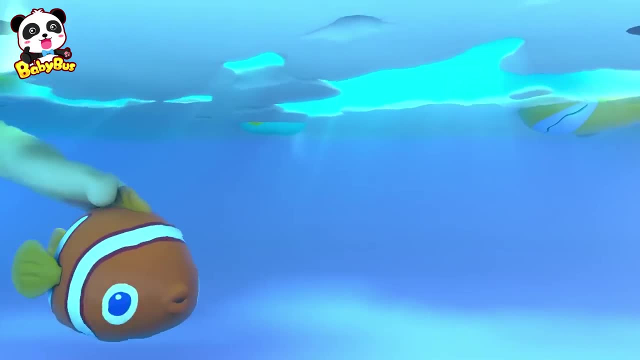 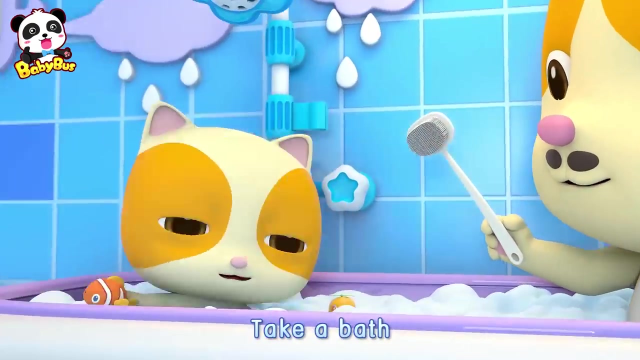 Wash under your arms too. Pop, pop, pop, pop, pop. I want to take a bath. Take a bath, Scrub-a-dub-dub. Take a bath. take a bath. Can you wash yourself? Take a bath, take a bath. Yes, I can. 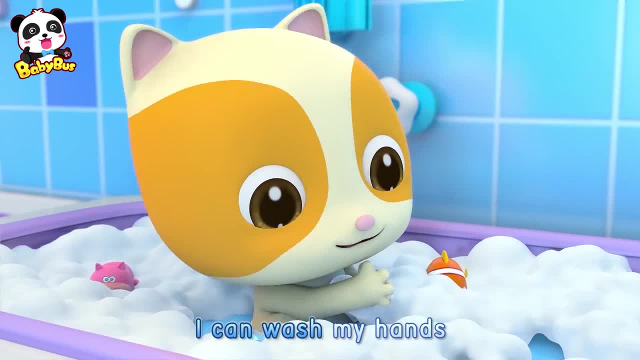 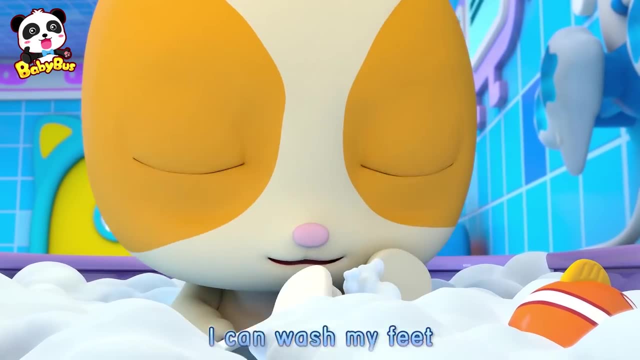 Can you wash your hands Scrub-a-dub-dub? I can wash my hands, Scrub-a-dub-dub. Can you wash your feet? Pop, pop, pop, pop. I can wash my feet, Pop, pop, pop pop. Front and back and fingers. 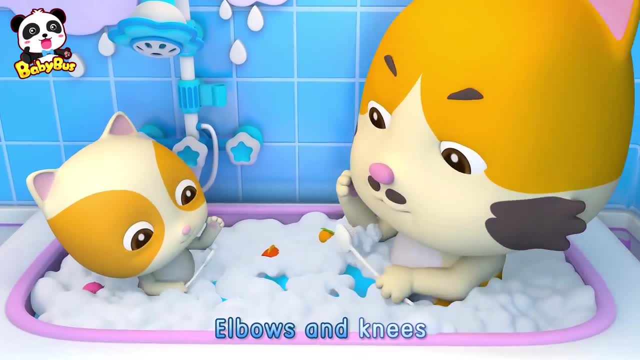 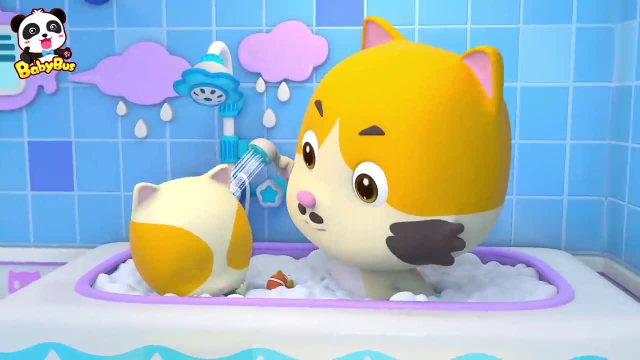 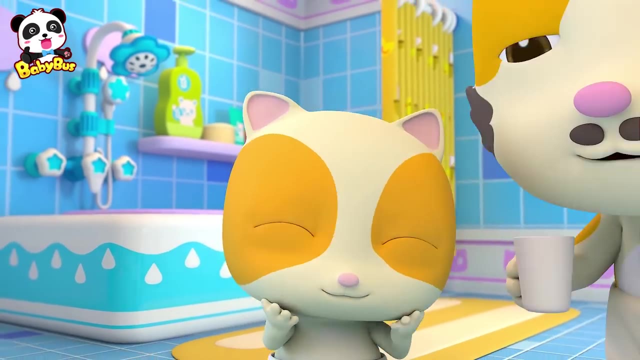 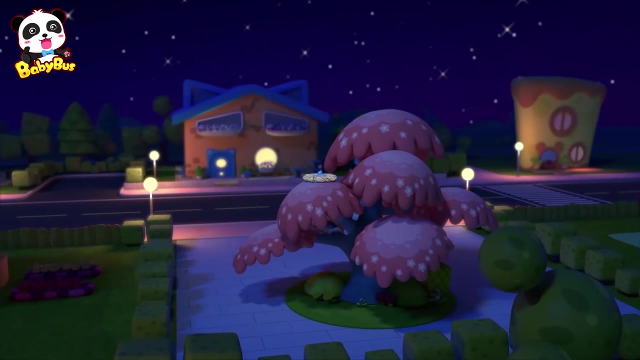 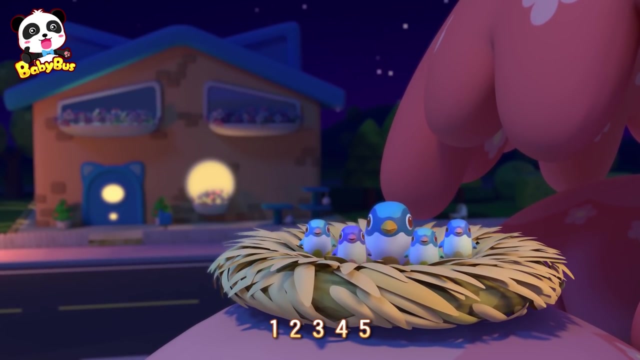 Toes, tops and heels, Elbows and knees, Splash, splash pop. I love to take a bath. It's all done. I feel so refreshed. Drink some water after taking a bath, Wake up One, two, three, four, five. I'll be back in a minute. 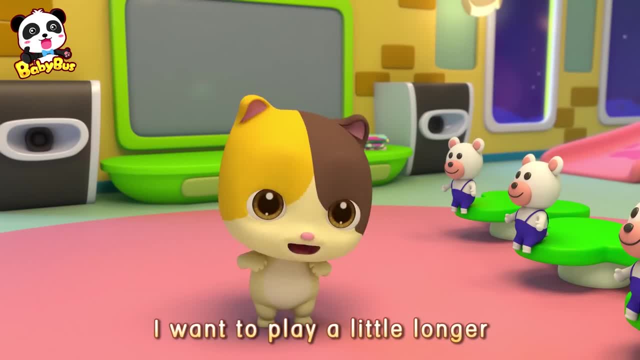 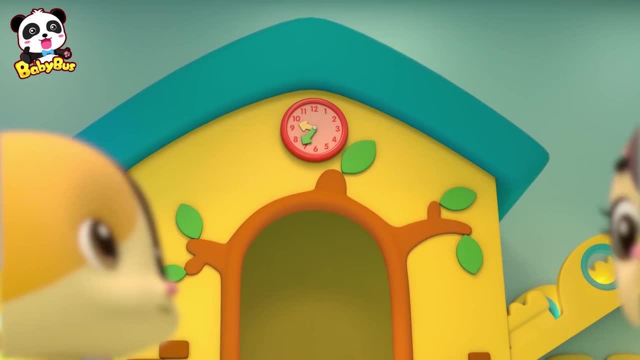 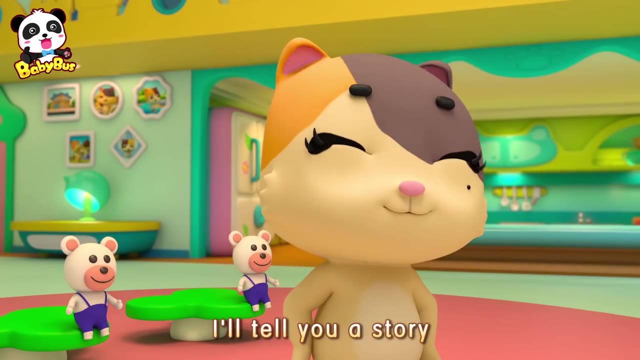 Mimi, it's too late. Mom, I want to play a little longer. Baby, it's already past your bedtime, But I don't want to sleep now. Alright, then I'll tell you a story. Great, I love bedtime stories, Haha. 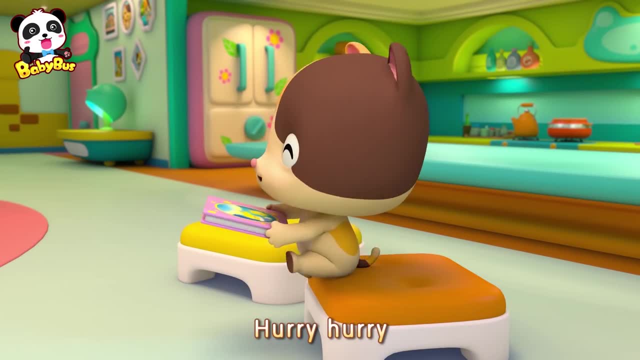 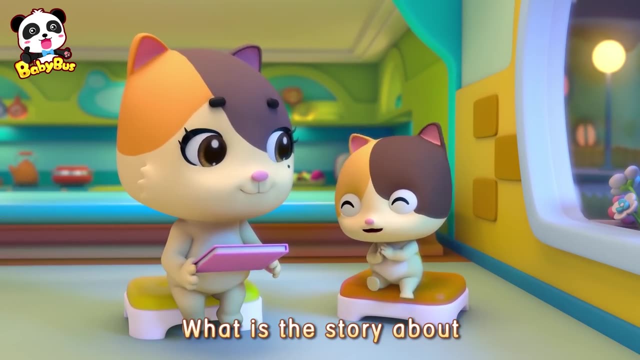 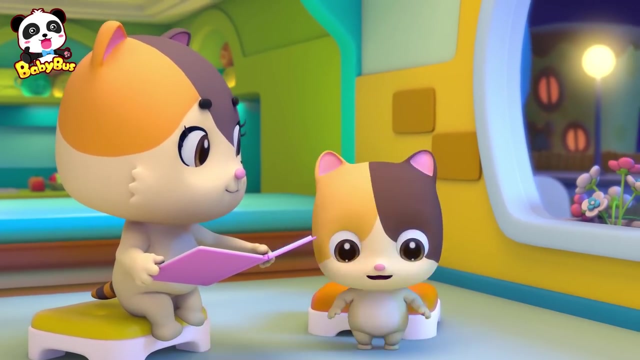 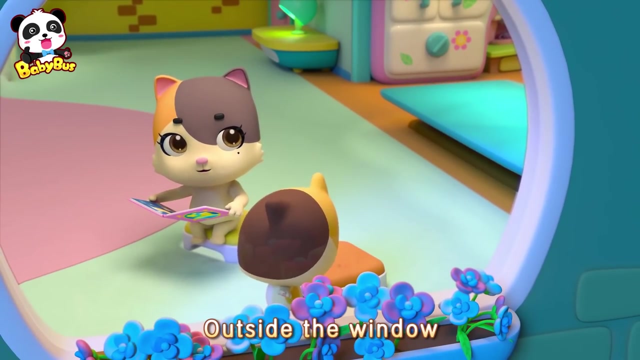 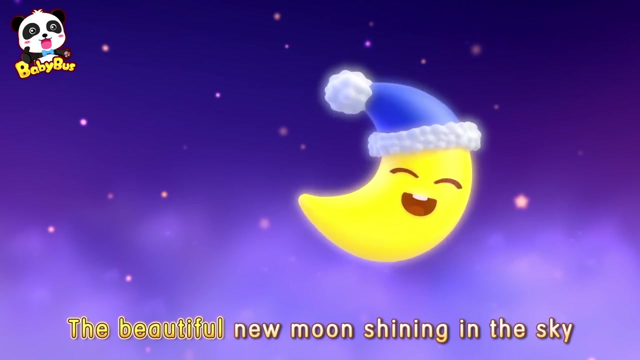 Hurry, hurry, Hurry, Hurry, Mom. what is the story about? It's about the moon and the stars. Wow, Mom, I can see the moon and stars outside the window. The beautiful new moon is shining in the sky. 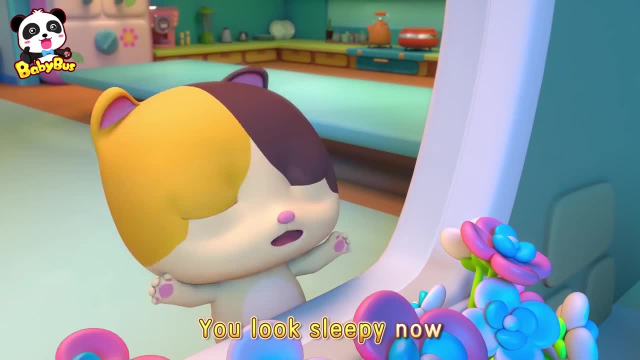 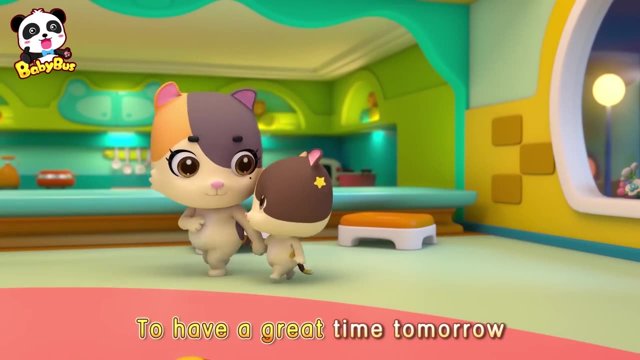 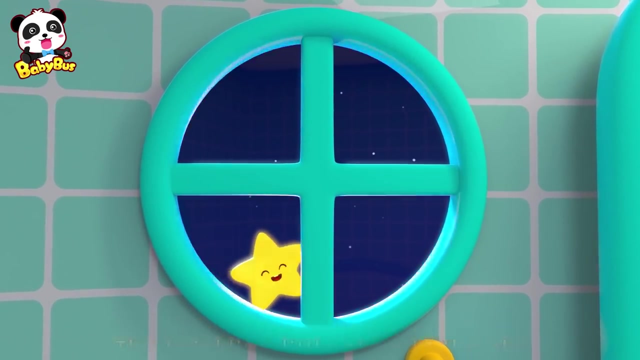 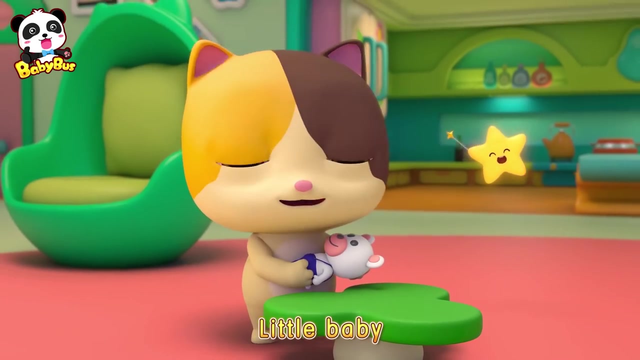 Seeing you rub your eyes. you look sleepy now. Little baby, go to your bed To have a great time tomorrow. The twinkling little stars in the sky. Seeing you blink your eyes. have a good night, Little baby. go to your bed To have a great time tomorrow. 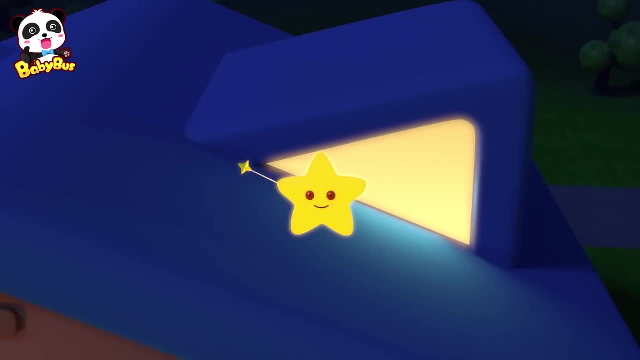 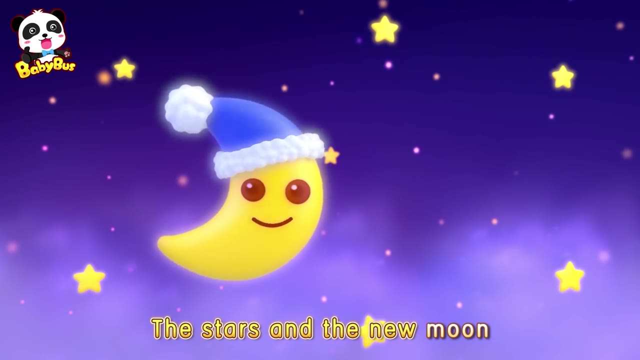 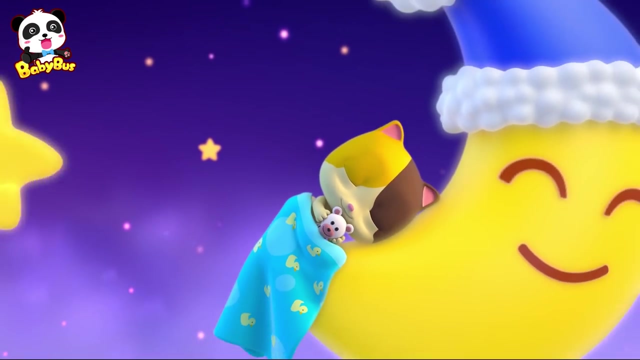 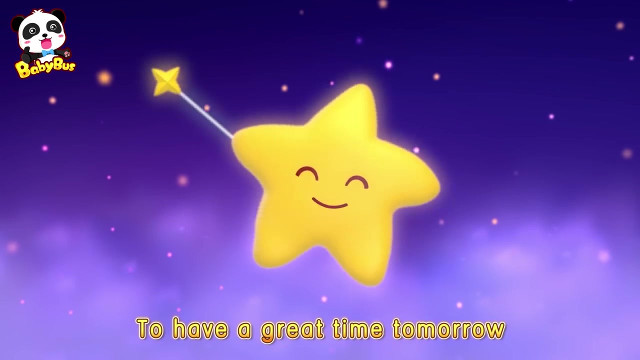 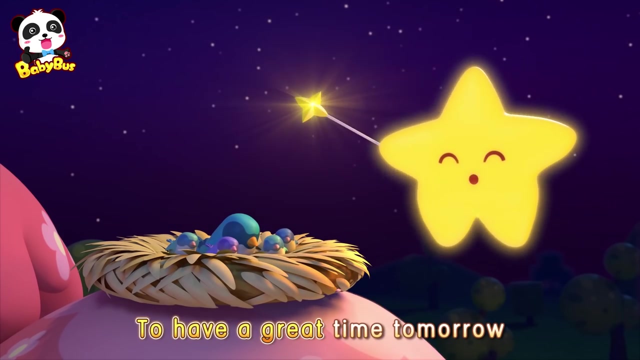 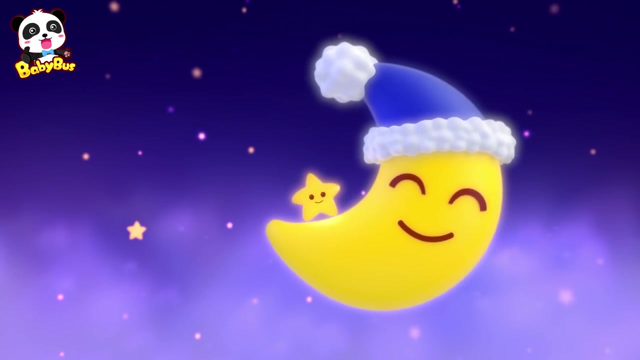 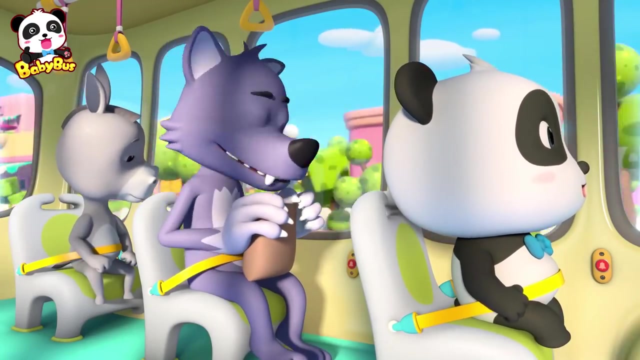 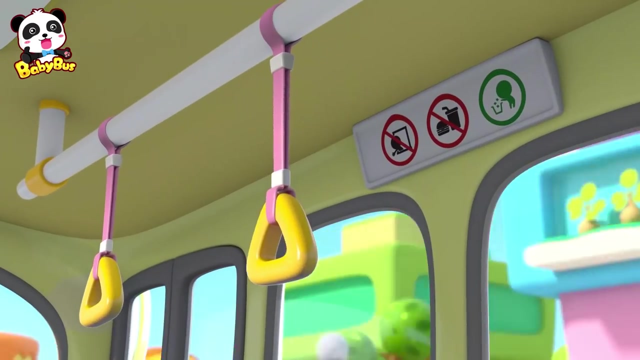 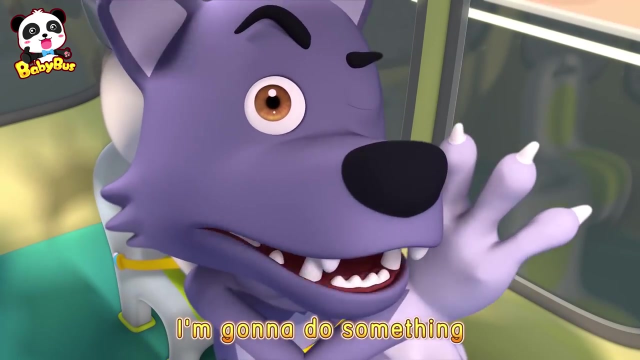 Good night. The stars and the new moon are shining in the sky, Seeing you close your eyes and fall asleep. Little baby, Have sweet dreams To have a great time tomorrow. Everyone fell asleep. Now it's your turn To have a great time tomorrow. Good night, I'm gonna do something. 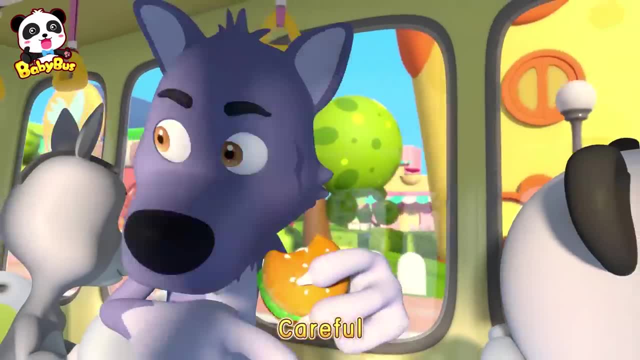 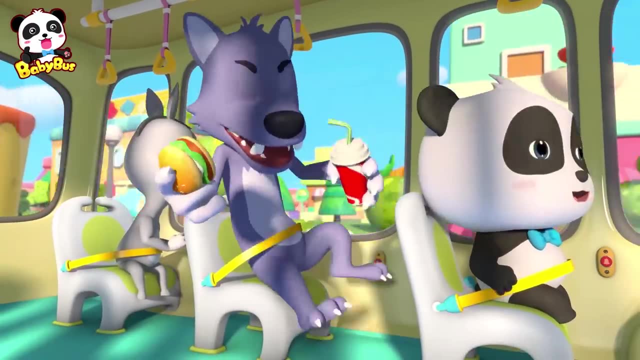 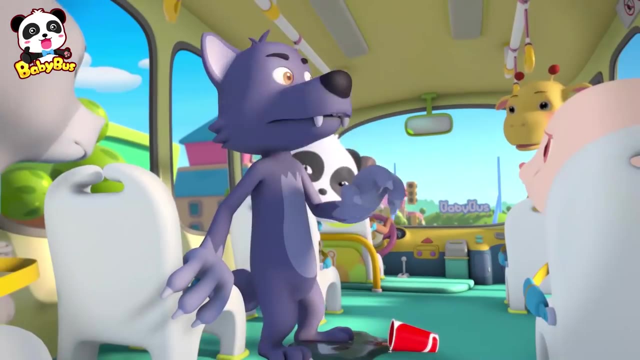 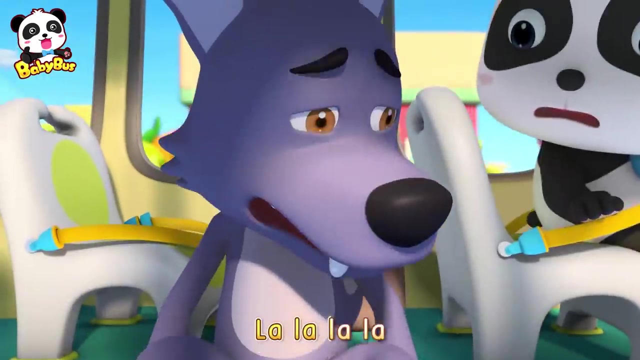 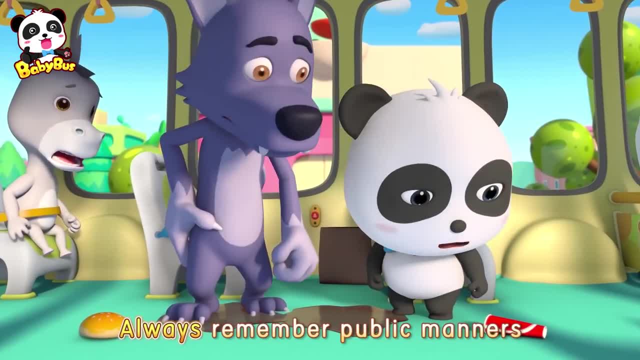 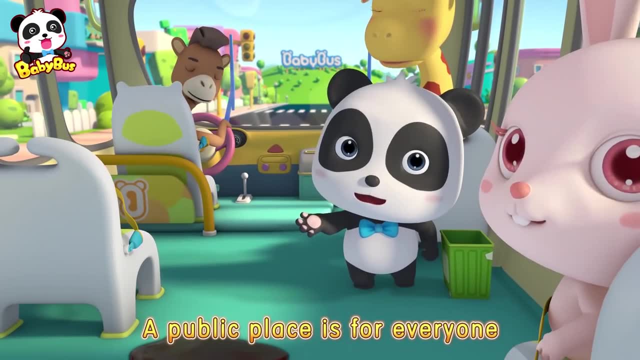 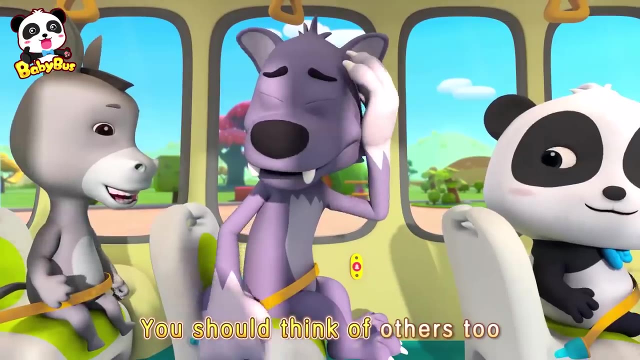 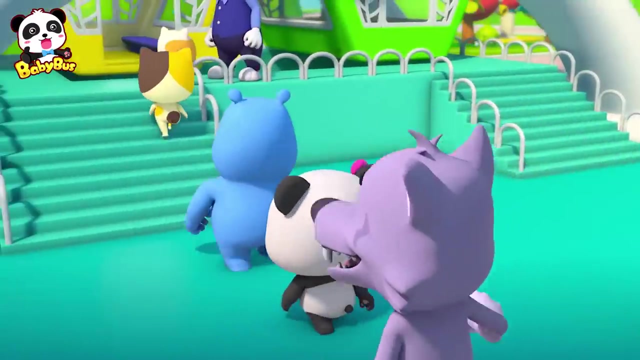 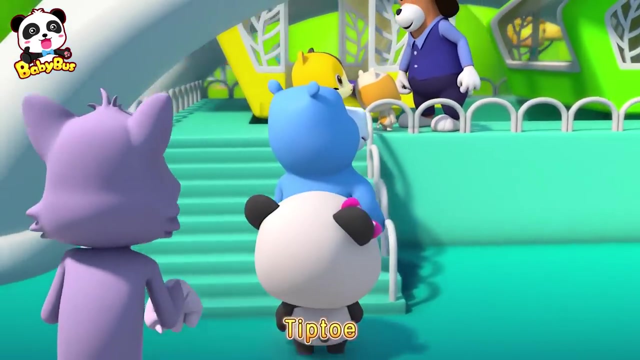 Oh man, Always remember public manners, Public manners, No public places for everyone, for everyone. Before you do something, think again, Think again. You should think of others too. I'm gonna do something. nobody's watching me. Tiptoe, tiptoe, Tiptoe, tiptoe. 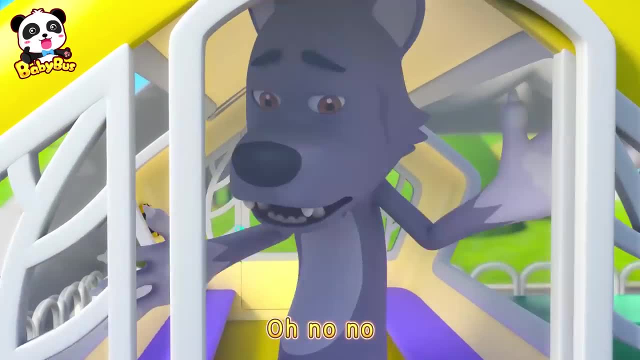 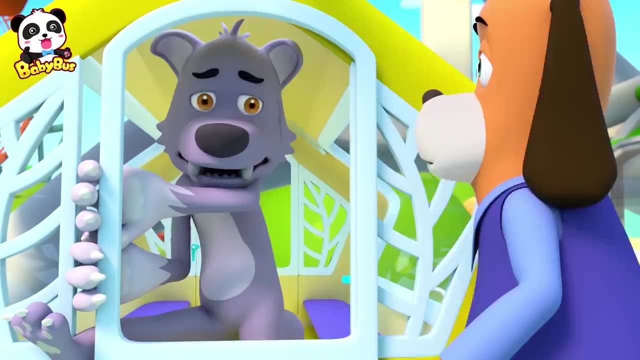 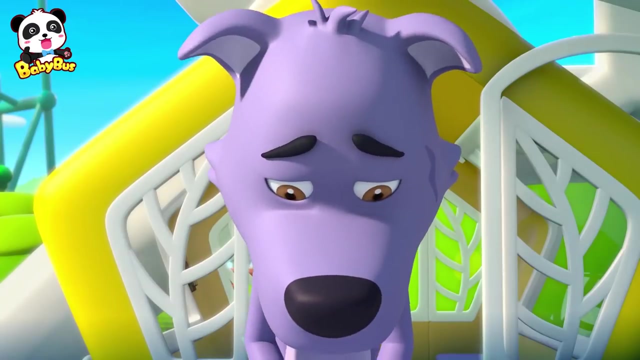 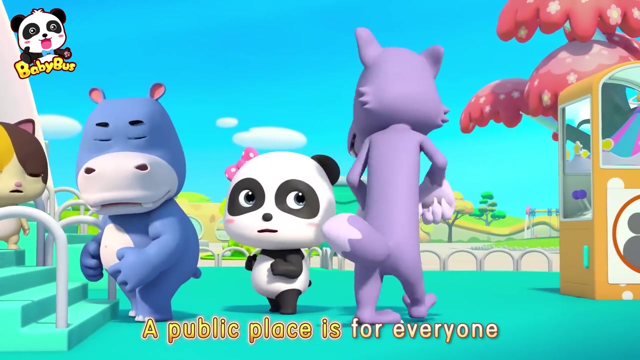 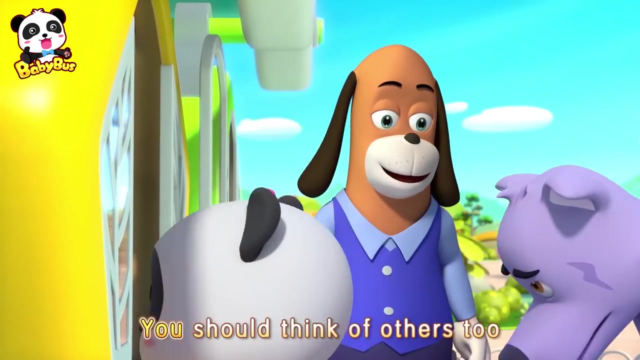 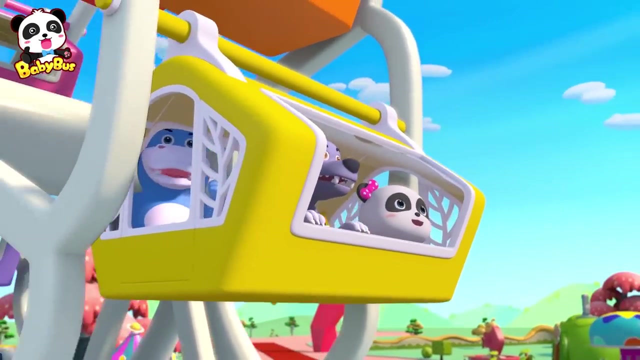 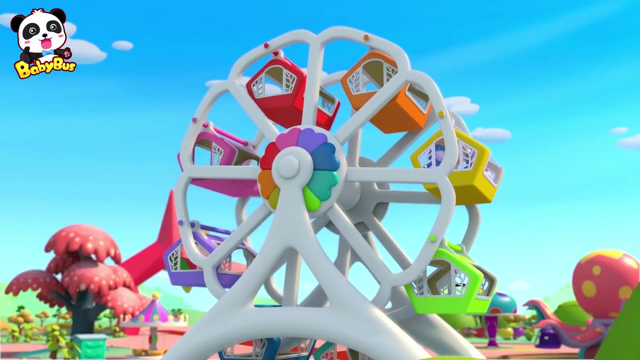 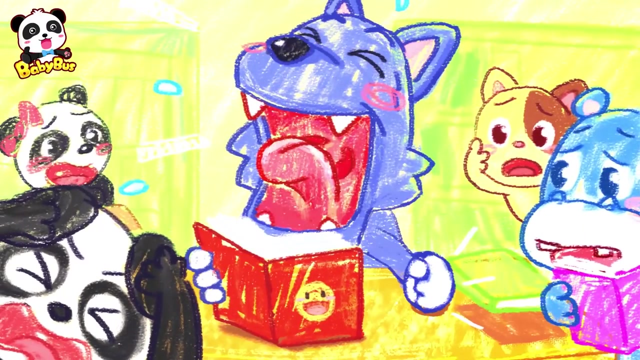 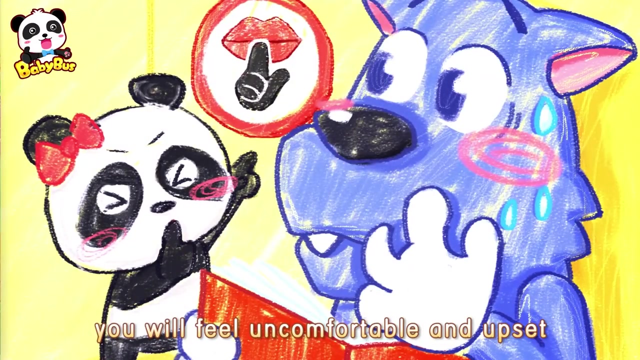 Oh no, no, I'm in trouble. Always remember public manners. A public place is for everyone. Before you do something, think again. You should think of others too. Why should we have good manners in public? If someone has bad manners in public, You will feel uncomfortable and upset, won't you? 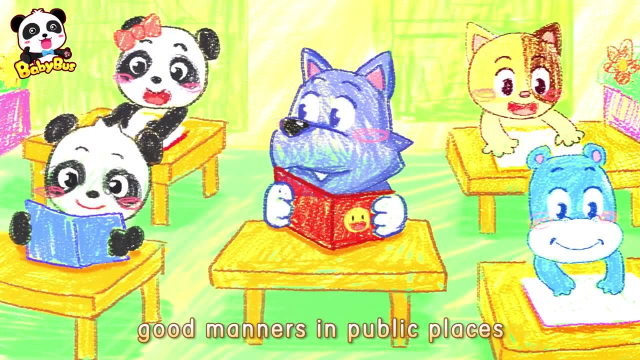 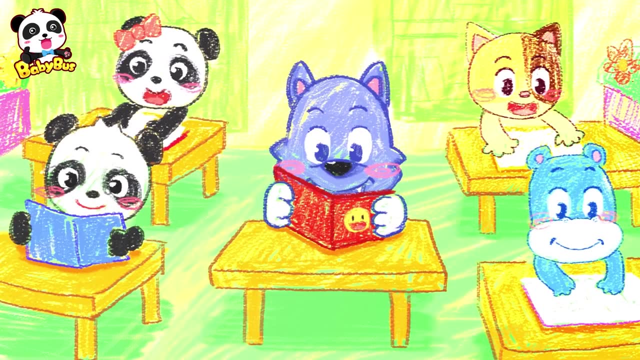 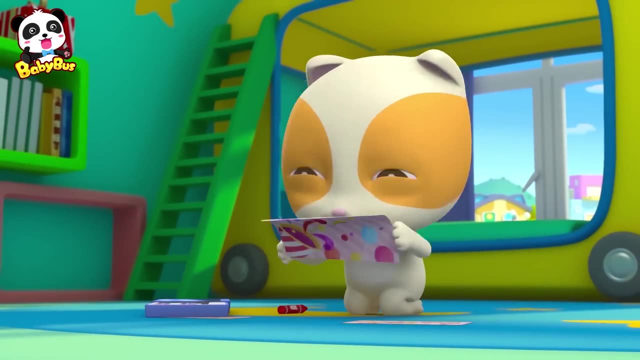 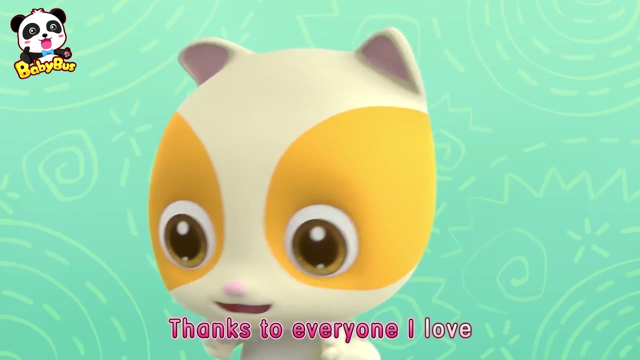 That's why we all should have good manners in public places. It will make our world a better place for everyone. I want to say thank you, Thank you to all. Thank you, thank you. Thanks to everyone I love. Thank you, thank you, Thanks to everything I got. 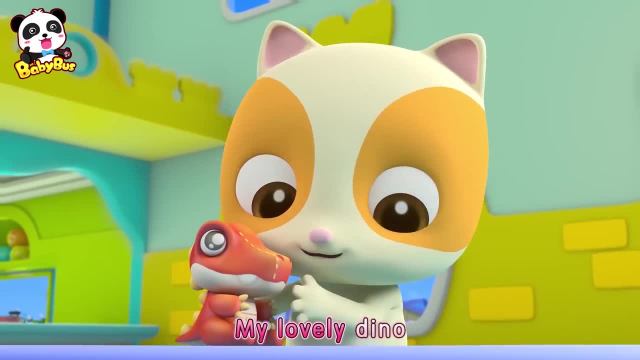 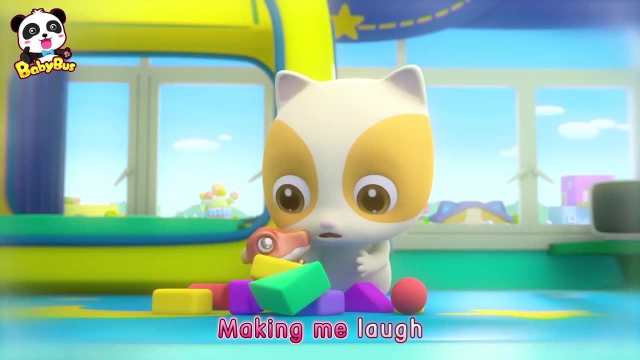 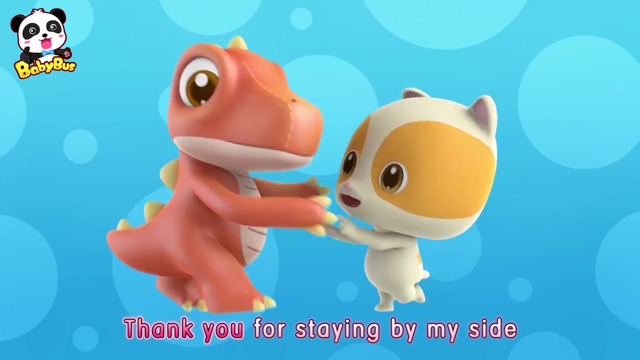 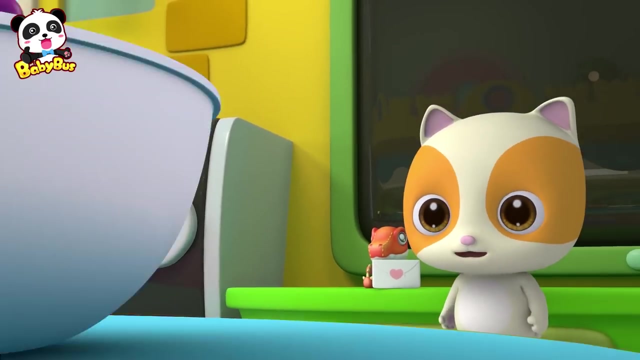 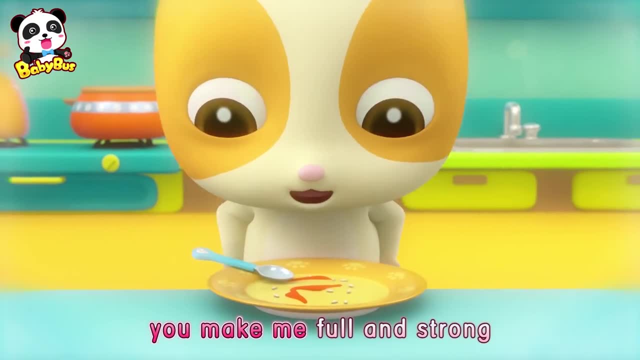 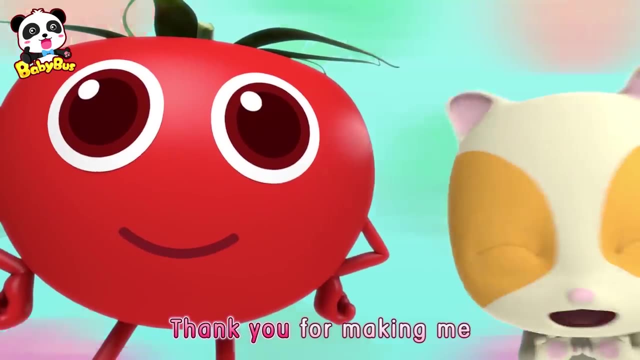 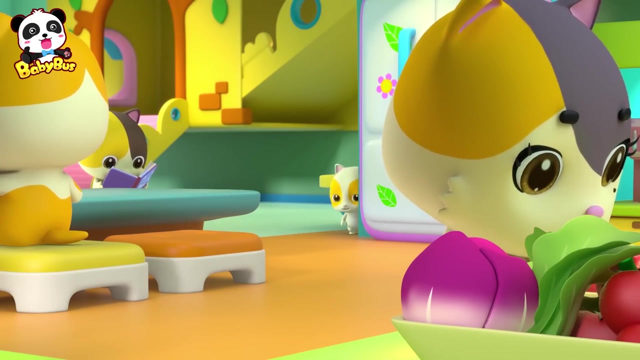 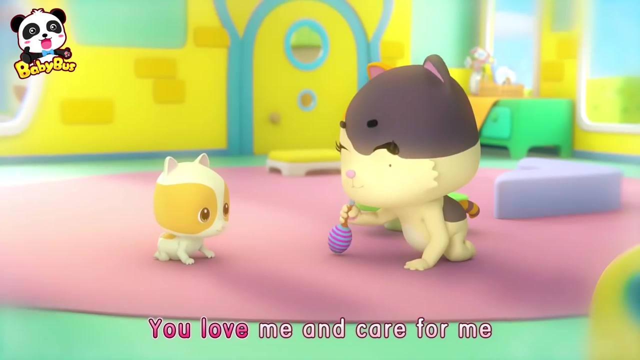